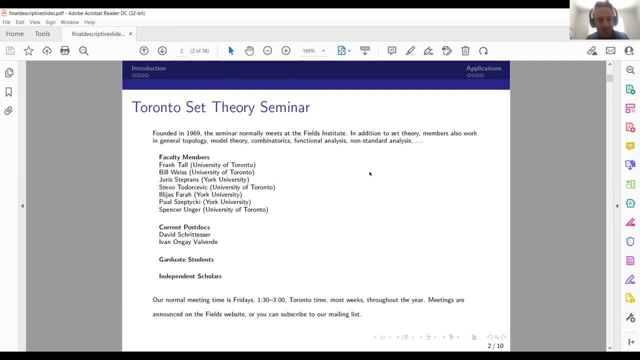 And his title is: Oh, it's just there, but now it's gone, So you have to say it yourself, Frank. All right, OK, but I want to start off by just saying a word or two about the seminar Founded in 1969, we meet at the Fields Institute and for entirely too long we've been meeting virtually. 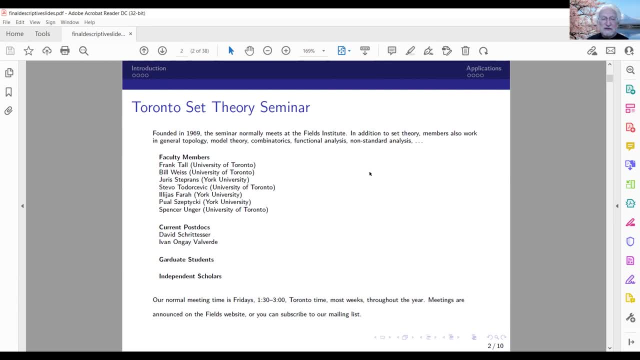 It's called the Set Theory Seminar, but members also work in whatever they're interested in, which is, for example, general topology, model theory, combinatorics, operator algebra, There's Bonnax spaces, non-standard analysis or whatever. 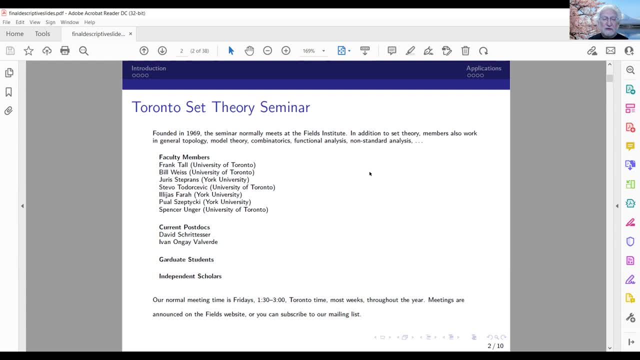 So the regular members from University of Toronto and from York University are up there, And then we have our current postdocs, And then there are graduate students- too numerous to name- and independent scholars and anybody else who shows up, which it's easy to do virtually. 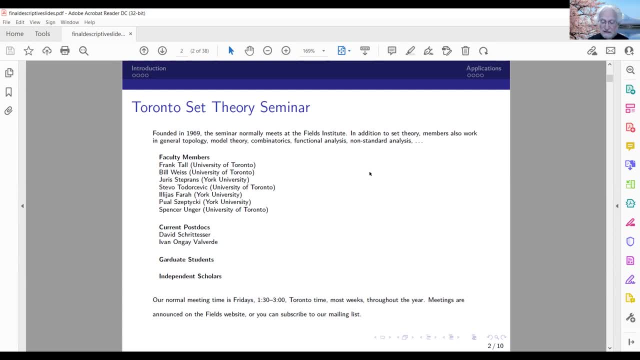 And David has Has shown how to subscribe to the mailing list. He'll show it again, I guess, at the end, But the normal meeting time is Fridays 1.30 to 3.. Today we'll run a bit longer. 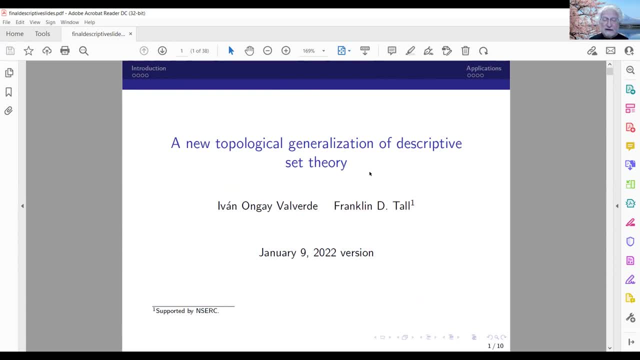 OK, so descriptive set theory deals with definable whatever. that means subsets of the real line In particular- and there's a history there of more than 100 years- things like Borel sets and later projective sets, whatever. 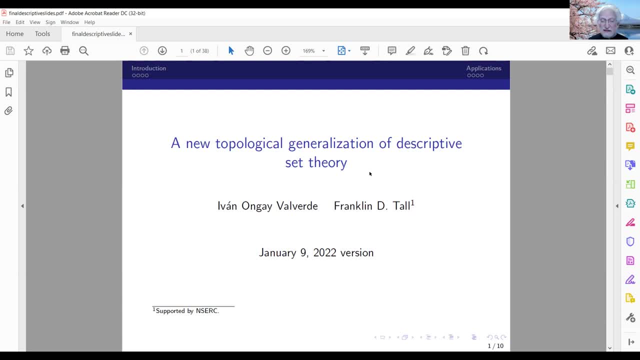 And the idea is that these are nicely behaved, they're measurable, or at least consistently they're measurable. But if you throw out the definability then you get using an action choice, non-measurable sets and whatever. So people have tried to generalize. 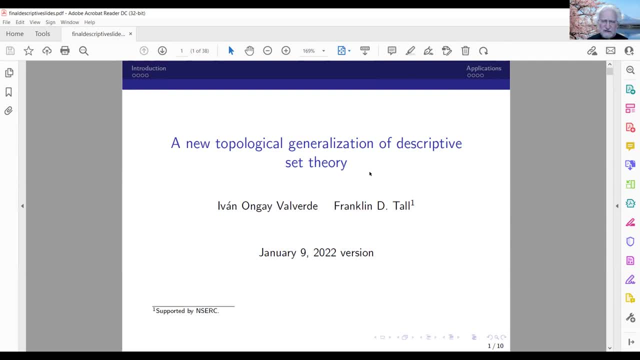 This from the original context of the real line To other contexts. one that's popular now is quite set theoretic. It looks at analogs of descriptive set theory on capital, the Kappa rather than the irrationals, which is omega to the mega. 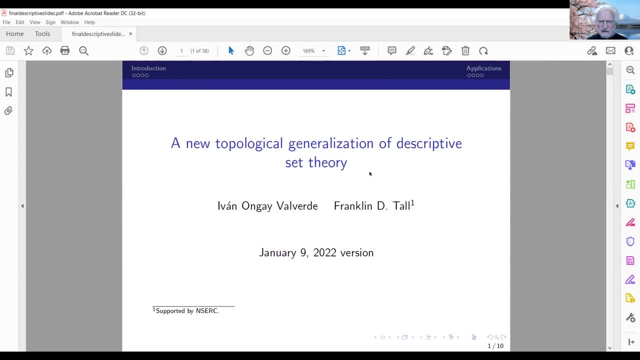 This is fine and interesting set theoretically, but it's not clear what applications it has. There's another line of attack started by Froehlich, Choquet and Rogers and Jane in the 1960s and later Also there was Stone tried to. 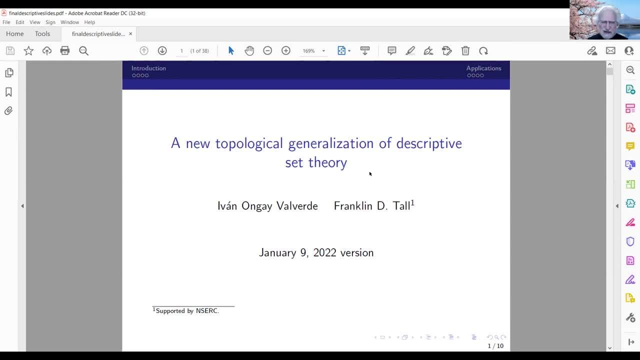 H Stone tried to generalize this to non-separable metric spaces rather than the usual Polish spaces: separable- completely betrisable. I don't think that worked out very well. Another line of attack that I just mentioned Was reasonably successful in generalizing the analytic sets, that is, the continuous images of Borel sets, to what are called the K analytic sets, which are generalizations of analytic sets to spaces that are not necessarily separable- betrisable. 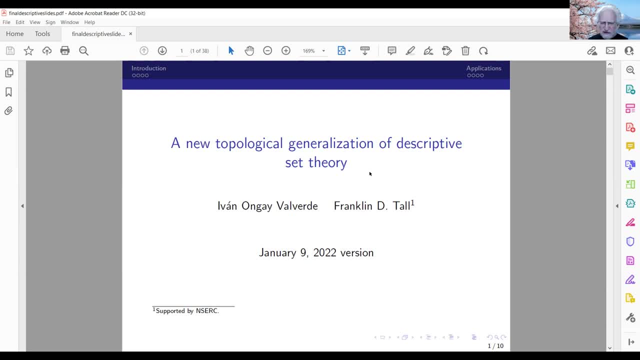 And curiously nobody seems to have Tried before me to Generalize the, the K analytic sets which have been used in functional analysis by a variety of people, to the K projective sets. So K analytic is the analytic is K projective is projective and so forth. 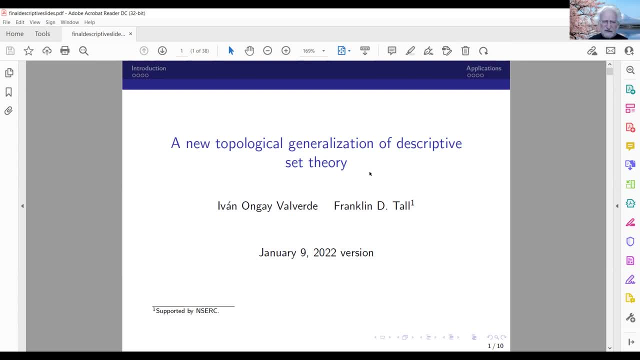 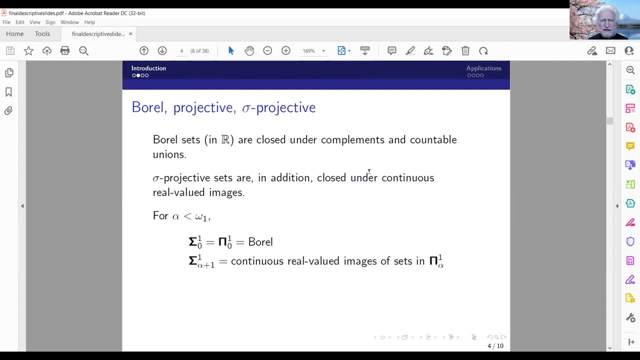 And then, if you continue that hierarchy, you get the sigma projective sets. So they're closed under complements, countable unions, countable intersections, continuous real valued images, Okay, And the notation you have: sigma 1, 0 equals pi, 1, 0 equals Borel, and sigma 1 alpha plus 1 equals the continuous real valued images of sets in pi 1 alpha. 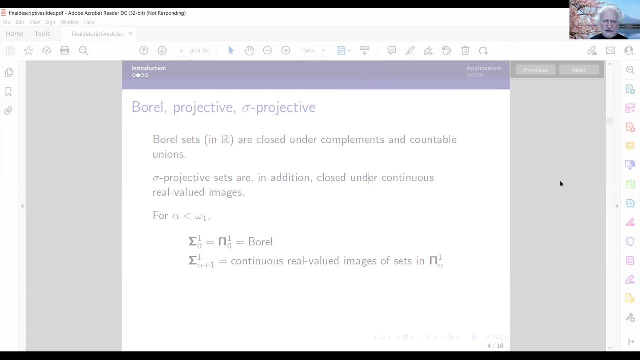 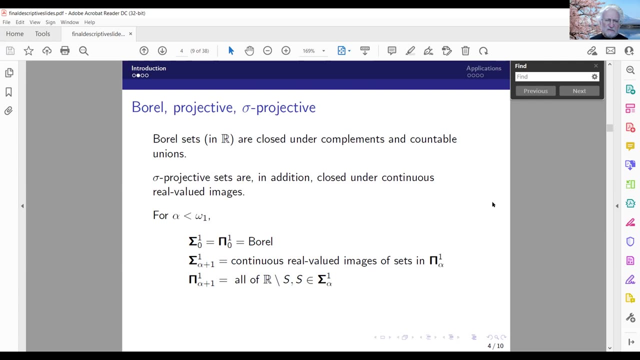 Just a minute, Minor technical difficulty. Okay, All right. So you would have sigma 1, alpha plus 1 as the continuous real valued images from the previous place in the hierarchy, and then the pis are all the complements of those, And then, at limit ordinals, you take unions. 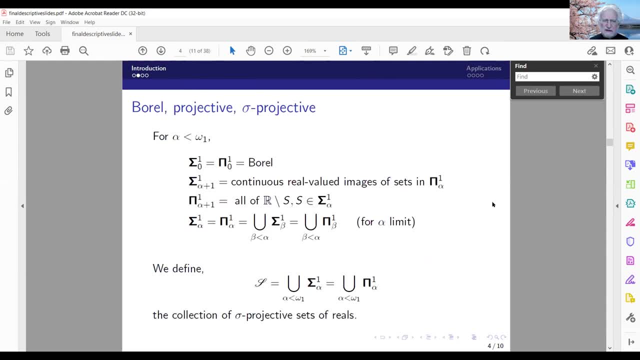 Now, and so if you do that up to omega 1, you get the collection of sigma projective sets of reals. Maybe these haven't been looked at too much because to do anything useful with them you have to assume sigma projective determinacy. 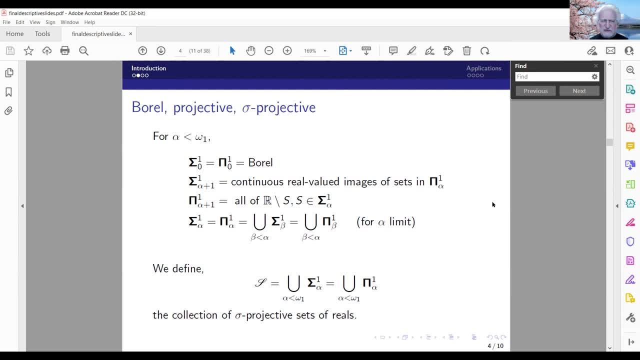 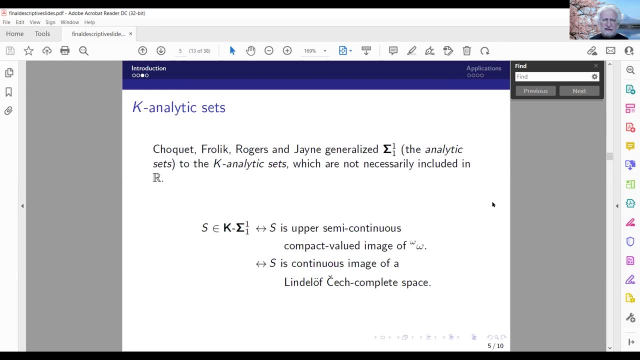 But that's okay these days because that just involves assuming some large cardinals. All right, The k analytics sets: generalizing the analytic sets. These are defined in 2 ways. One is the upper, semi-continuous, compact, valued image of the irrationals. 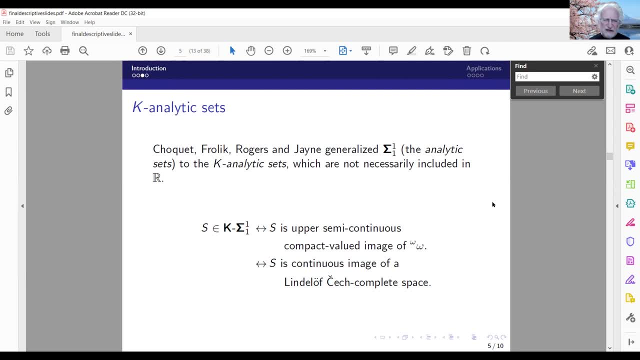 Yvonne in the next talk will explain what that's about. an equivalent definition Is there the continuous images of Lindelof check complete spaces, And the check complete means absolute g delta, that is, g delta in any compactification, In fact any superset, super space, and that's a simultaneous generalization of complete matrice, full and locally compact. 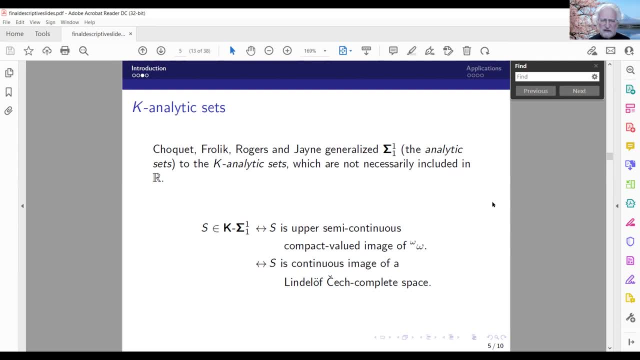 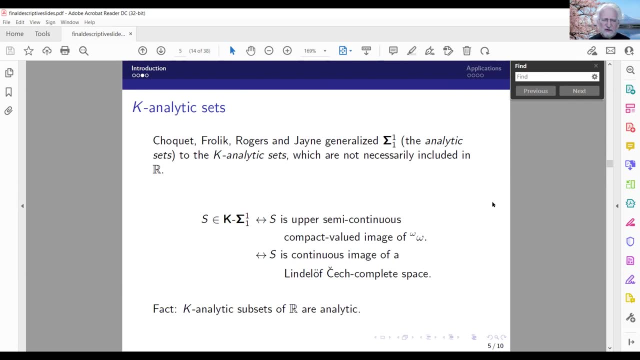 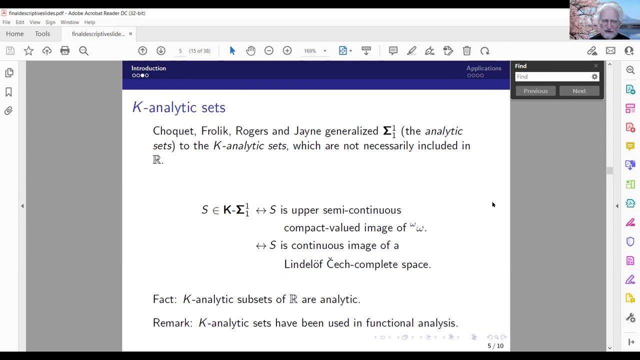 So here you're no longer a subset of the reals. However, when you look at, when you bring it down to the reals, Okay, Analytic subsets of the reals are, in fact, analytic, continuous images of Burrell. What does compact valued mean? Yeah, that's, we're gonna leave for Yvonne. 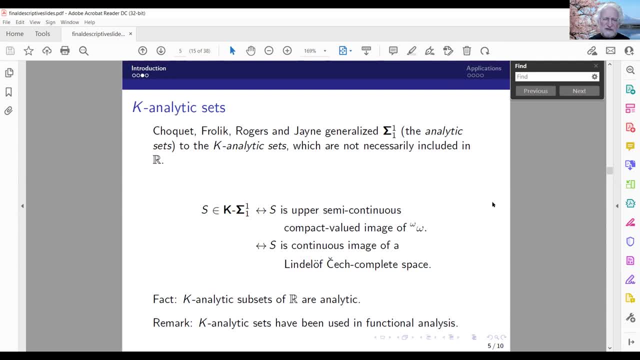 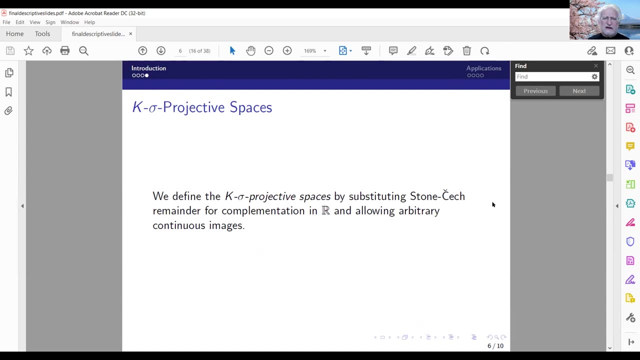 You can. i'm just mentioning it here for the purposes of my talk. We'll just consider the k analytic sets as the continuous images of Lindelof check complete spaces. Oh, of course, Yeah, that's all right. All right, So in defining the k sigma, projective spaces, 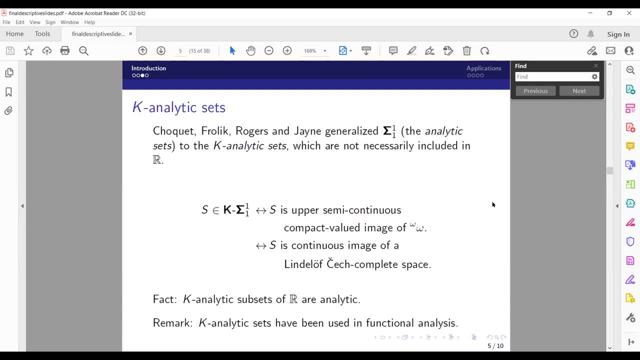 Wait, no, but I have a little question still, like: what are the target? What target spaces do I mean? Any target spaces, Any target space? Yeah, So this is what's different from the usual analytic and projective hierarchy where you are all looking at subspaces of some Polish space. 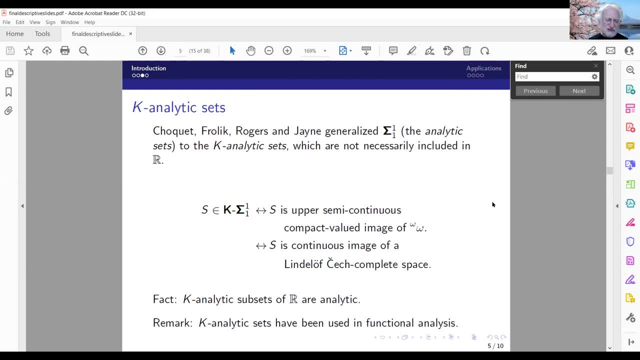 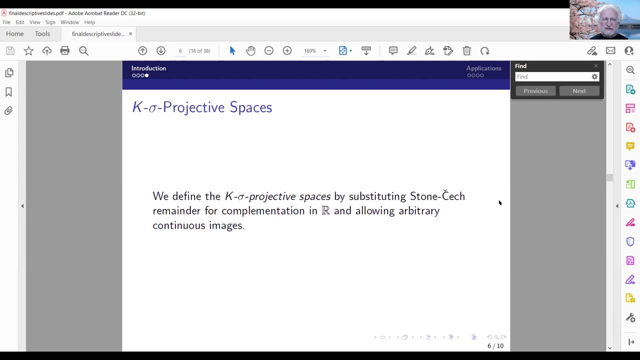 Some Polish space, such as the reals. here There's no such restriction, and this gets more complicated when you start trying to throw in complementation and continuous images. So, rather than taking the complement, we're gonna define the k sigma projective spaces by taking stone check remainder. 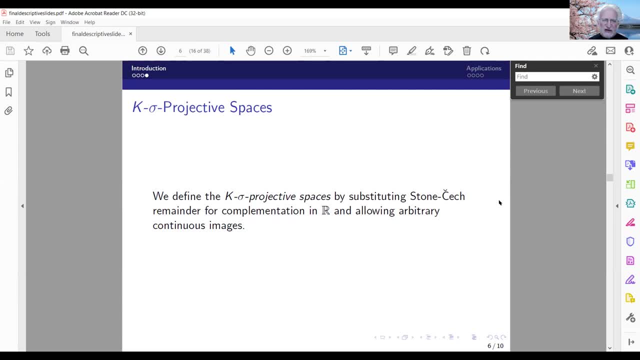 Or really could be any compact remainder in a compactification and allowing arbitrary- not just real- valued continuous images. All right, So immediately you see some obvious problems because now you're dealing with whole classes of spaces. You don't have a class problem when you're dealing with the usual projective or signal projective hierarchy. 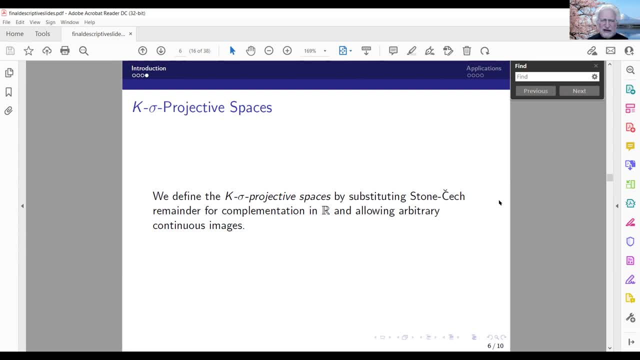 However, you can avoid dealing with classes By noticing that if you have class, if you have arbitrary, large, inaccessible cardinals, then you can just look at the V Kappas and notice that when you're working in a particular V Kappa, Kappa in excess, strongly inaccessible complementation- 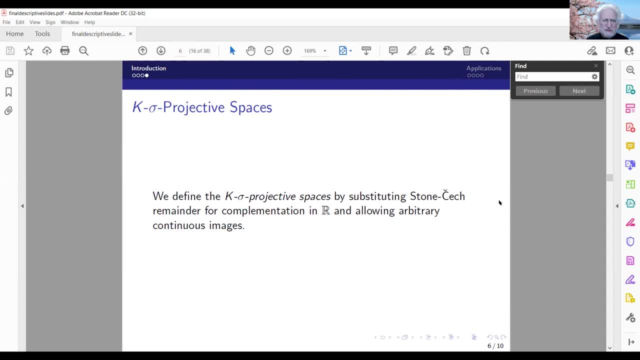 I mean sorry, stone check remainder and continuous image. do not take you out of the Kappa, So you can think of this As just all these V Kappas getting bigger and bigger, and then you don't have to deal with classes. 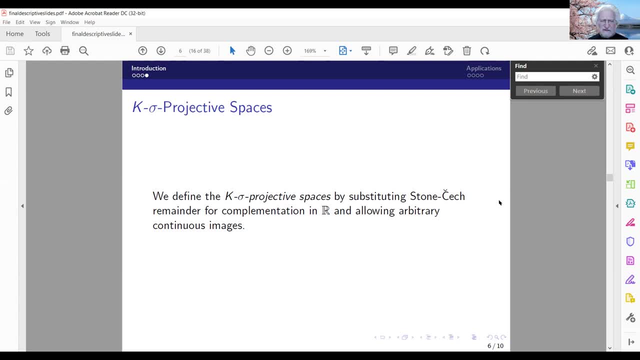 This is arbitrary. large, inaccessible cardinals is a relatively innocuous assumption these days, And in fact, we need to do more than that to get the amount of determinacy we need. All right, So is this useful? All right, So the K? 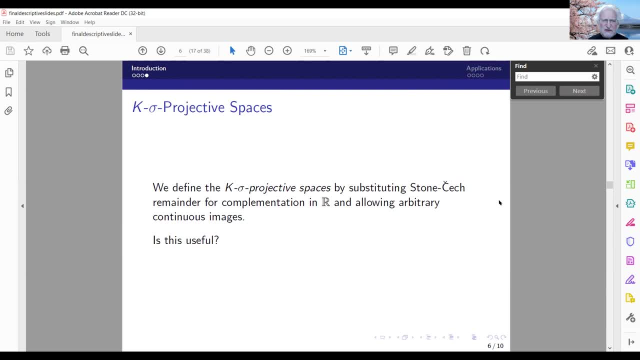 Analytics sets, as I said, have been used in functional analysis. Can I do anything with the K Sigma projective spaces? And so i'm going to give an example in selection principles theory where I can do something with it. So the key concept here: a space is projectively sitting, projective- 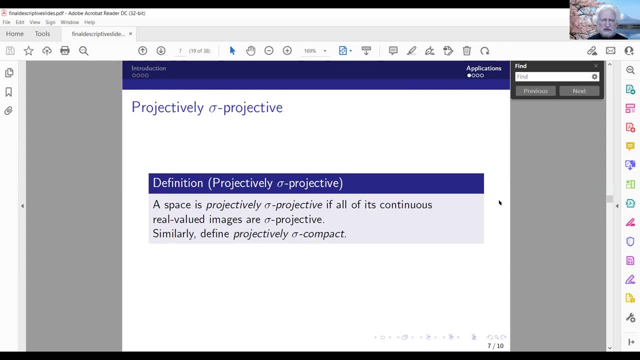 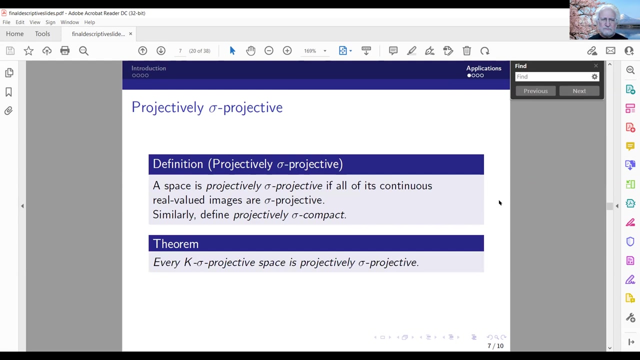 If all of its continuous real valued images are sigma projected. similarly- and this was defined long before I started working on this, Our hoggles key defined it: projectively: sigma compact. If a space had all its continuous real valued images: sigma compact. Okay. 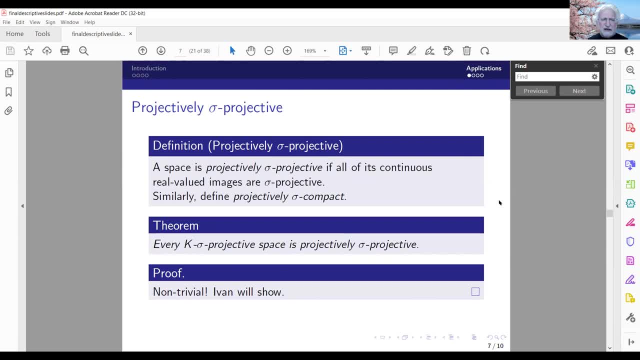 The main theorem Here Is that every K Sigma projective space is projectively sigma projective. When you map it down to the real line you get a sigma projective set. This is not so easy to prove and Yvonne will show that in the next talk. 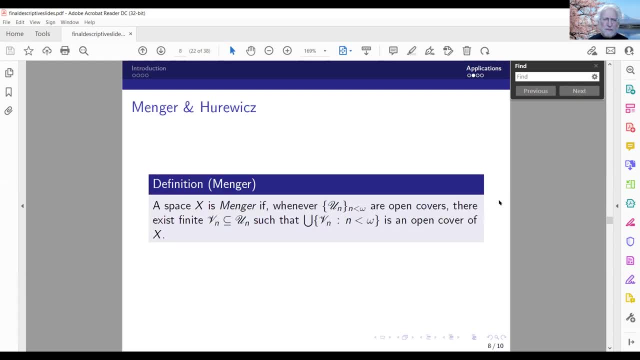 And using that we get a non-trivial theorem. All right, So this is a cross selection principles. before have probably heard about Manger and a ravage subsets of the reels and question of whether Manger implies her a rich or sigma compact or whatever. 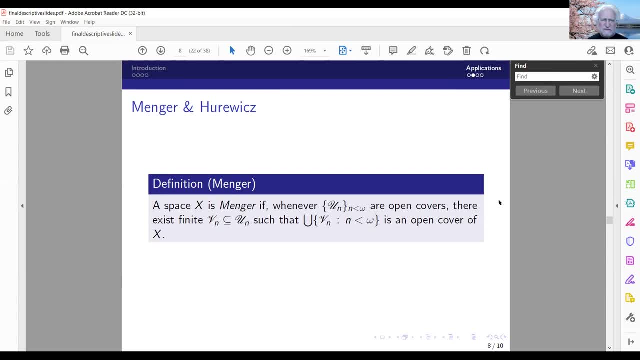 Definition of Manger is relatively simple. It's a generalization of Lindelof or no special kind of Lindelof. I should say, if you have countably many open covers, you can get finitely many open sets from each cover. 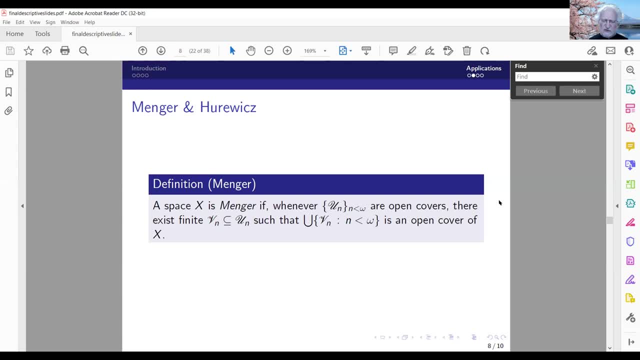 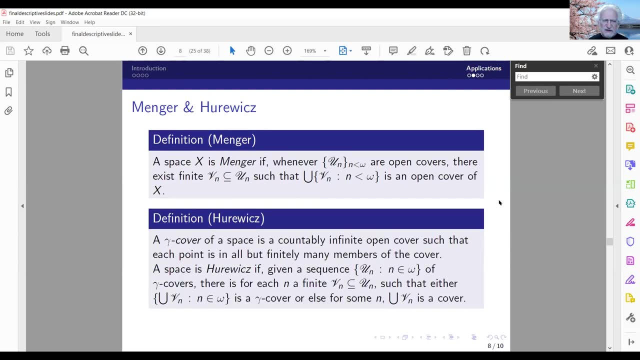 Such that If you have two of them you get an open cover. So stronger form of Lindelof Horavitch has a complicated definition. I can never remember it, But if you take a look at it here you can see it's has some sort of the same flavor as Manger. 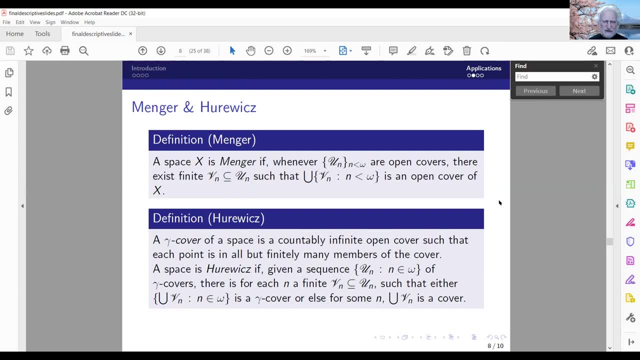 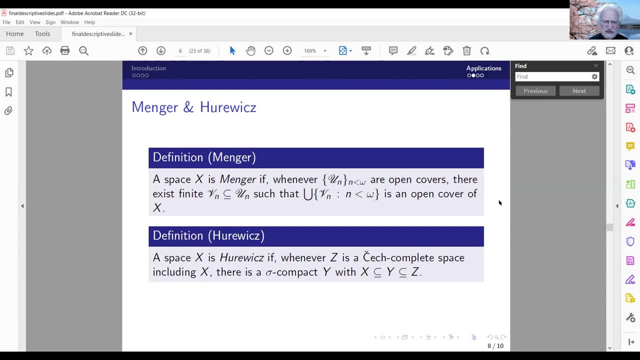 Anyway, this is the classical definition. I guess you can figure out who it's due to And I prefer, because it's easy to remember, at least for me, an equivalent definition that a space is a ravage If, whenever you take a check complete space including X, you can fit in a sigma compact space between X and the and the check complete space. 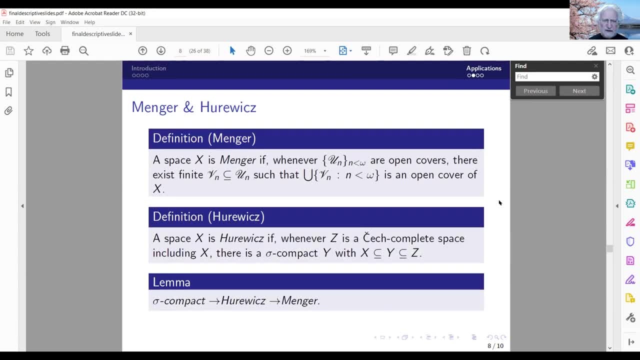 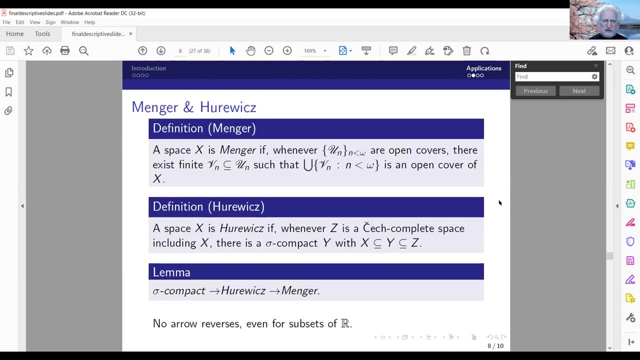 Okay, All right. So it's not too hard to show that sigma compact implies a ravage, implies Manger. It's hard to show that the arrows don't reverse, But that is the case, And people working in selection principles have amassed a variety of results about when the arrows go back. 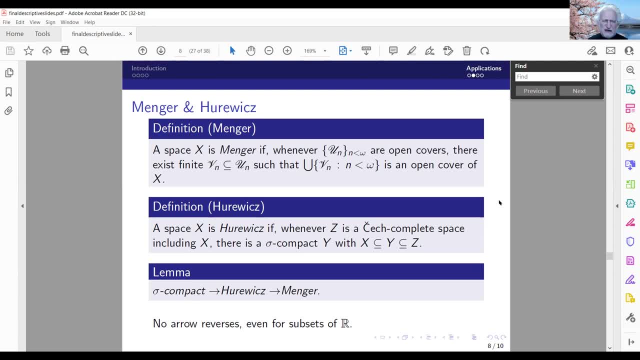 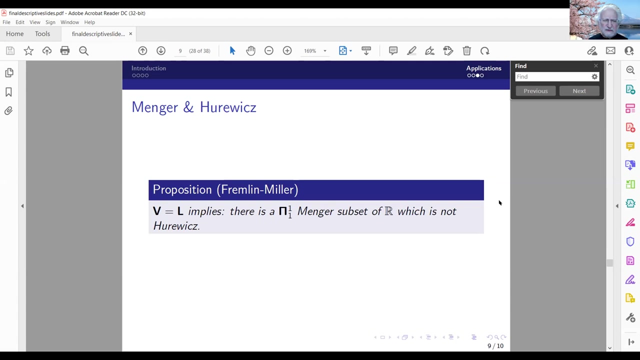 And the general theme is that for definable sets, However you define definable Manger, definable sets are consistently, possibly assuming large cardinals or something, They're consistently sigma compact, On the other hand, from Miller showed that vehicles L implies there's a pi one, one or coanalytic. 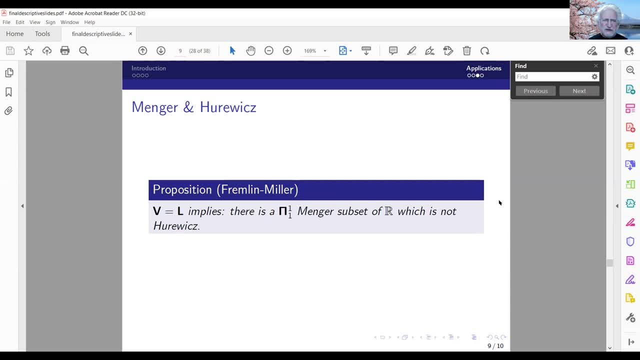 Manger subset of the reels which is not Kurevich. But on the other hand, if you assume coanalytic determinacy, you get coanalytic Manger subsets of our, our signal compact. So lots of undecidability going on here. 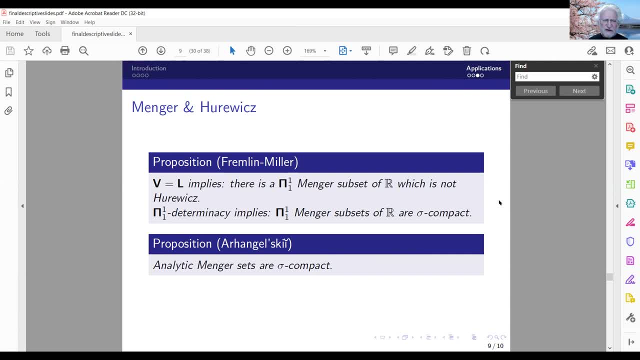 On the other hand, if you try to see what you can get without extra set theory, Our Hangelski showed that analytic Manger sets are sigma compact, Where you can define analytic, even to be continuous images of Burrell without requiring them to be real, valued continuous images. 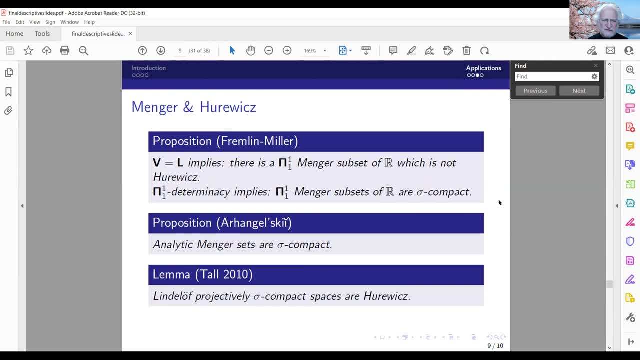 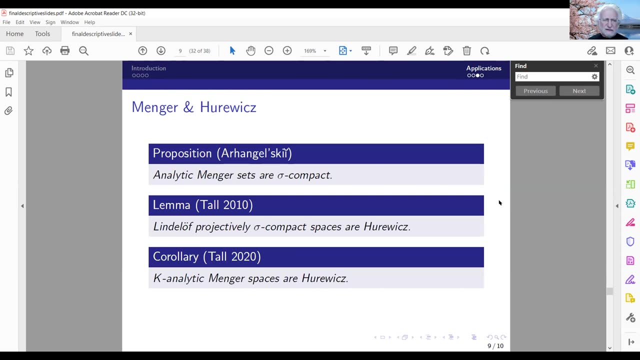 Okay. I showed in my paper on productively Lindelof spaces that Lindelof projectively sigma compact spaces are Horavich. using our Hangelski's methods And as a corollary of that work I was able to show that K-analytic Manger spaces are Horavich. 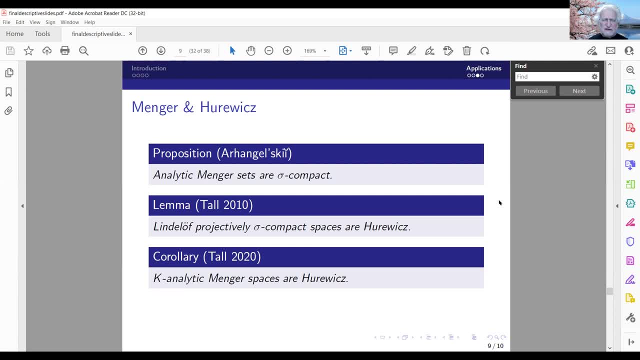 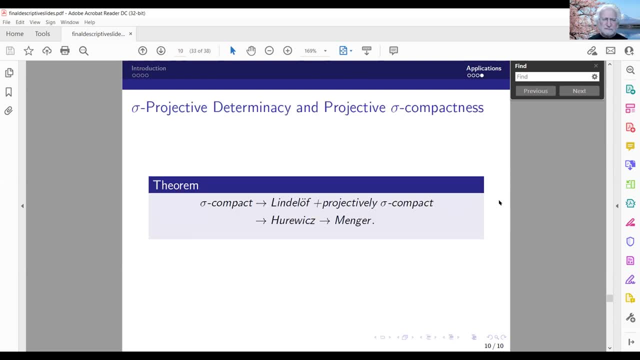 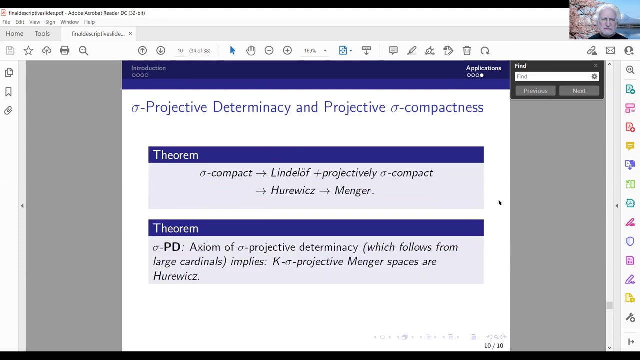 But there are ZFC examples of K-analytic Manger spaces which are not sigma compact. So the situation we have is: sigma compact implies Lindelof, plus projectively, sigma compact implies Horavich, implies Manger, And without extra restriction. Without extra restrictions, no arrows reverse. 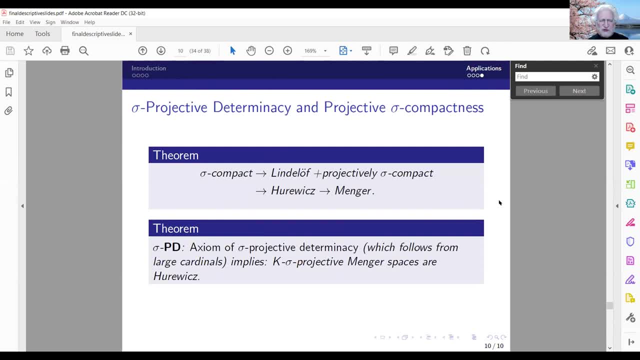 All right. So our theorem is that the axiom of sigma projective determinacy, which follows from large cardinals and talks about games being determined on sigma projective sets, This implies K sigma projective Manger spaces are Horavich, And so let's see how this is going to go. 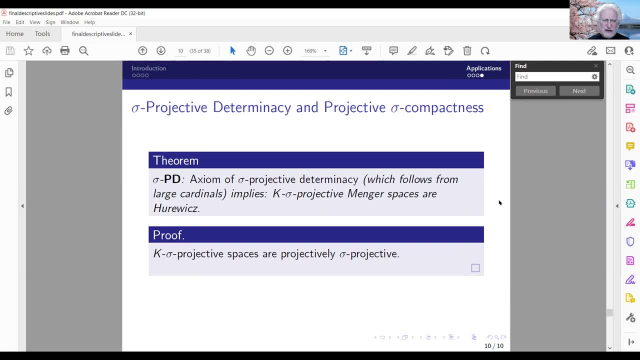 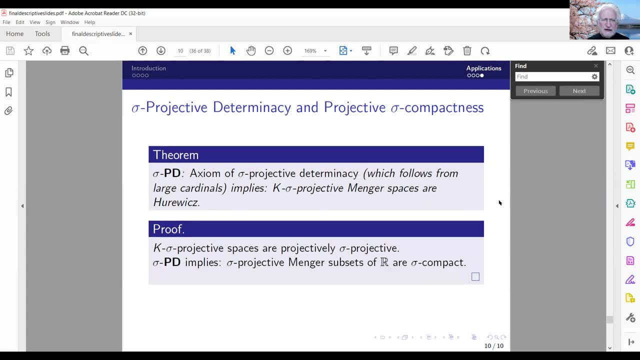 All right. Well, we need the main theorem that K sigma projective spaces are projectively sigma projective And that sigma projective determinacy implies sigma projective. Manger subsets of the reals are sigma compact And that's proved. the same way as from Miller do the coanalytic. 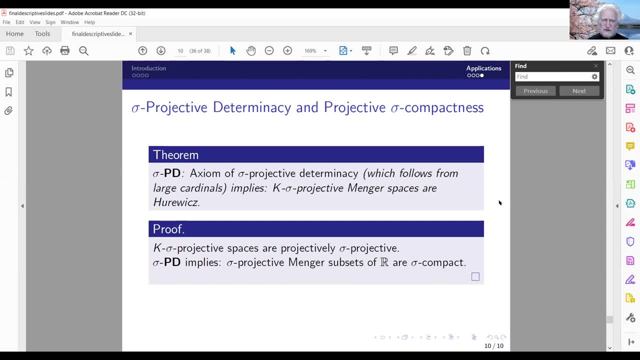 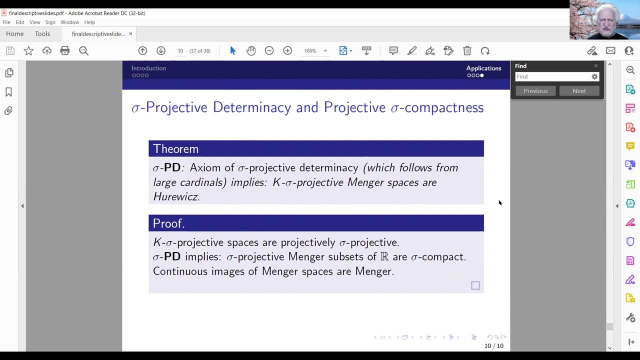 And other people, including myself, have done it for projection, And other people, including myself, have done it for projective. Okay, so continuous images, Manger are Manger. that's just like continuous images of Lindelof or Lindelof. 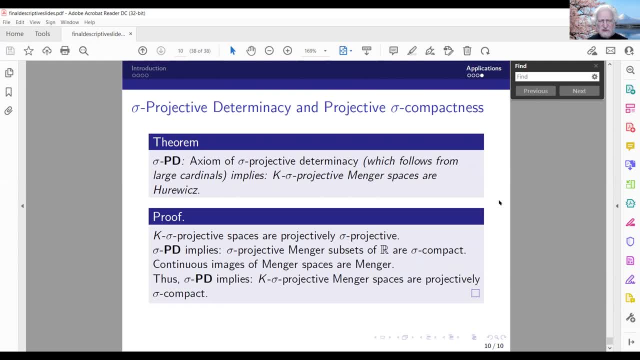 And so sigma projective determinacy is going to imply that K sigma projective Manger spaces are projectively sigma compact. And then, since they're Lindelof and projectively sigma compact, they'll be Horavich, And so that'll prove the theorem. 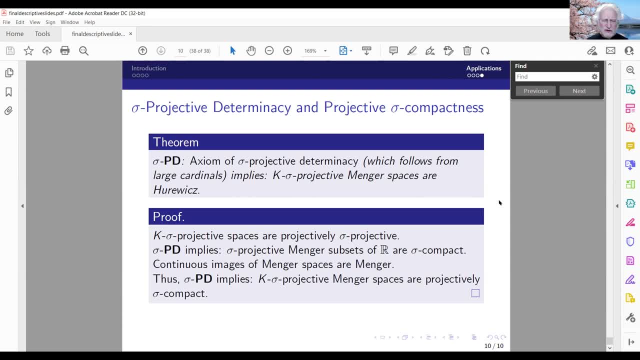 Okay, so that's a quick introduction to the K sigma projective hierarchy and a possible application. I think there are probably some applications to functional analysis. I just have to find some graduate student to go through all the K analytic uses in functional analysis and see which of them work for K projective. K sigma projective. 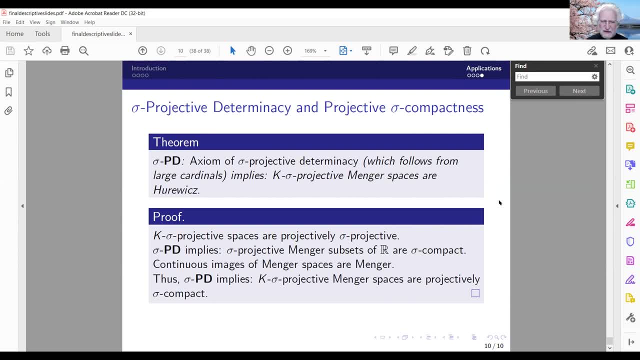 Assuming sigma Pd, I suspect some of them will go through, Some of them won't, We will see. But anyway we've extended the spaces that you can plausibly call definable to a much larger class than previously, And so hopefully those will have some good applications. 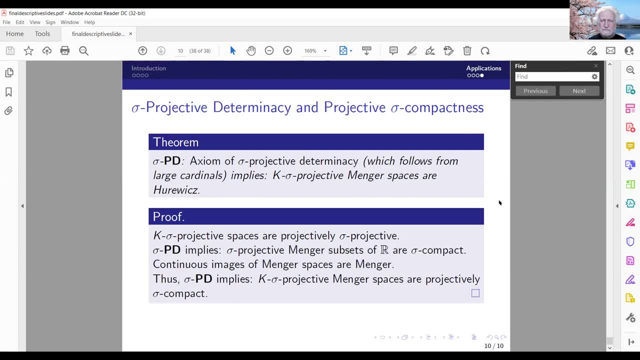 Thank you. Thank you, Frank, Very interesting. So are there any questions From the audience? I have a question, One other people hopefully make up their mind to also ask something, But okay, maybe it's a stupid question, I don't know. 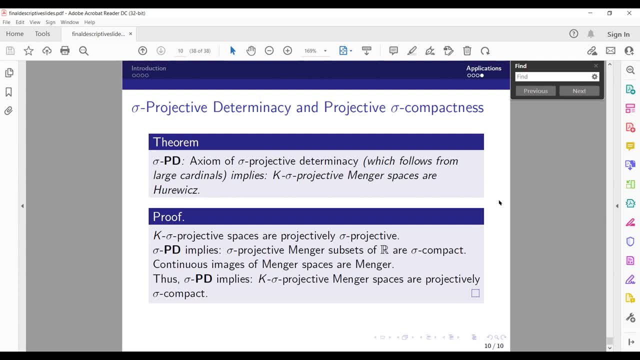 This, this thing that the it's. it reminds me a little bit of universally bareness. Maybe it's dual, because you know you're not restricting the domain of spaces, and universally bareness It's more sort of the other way around. 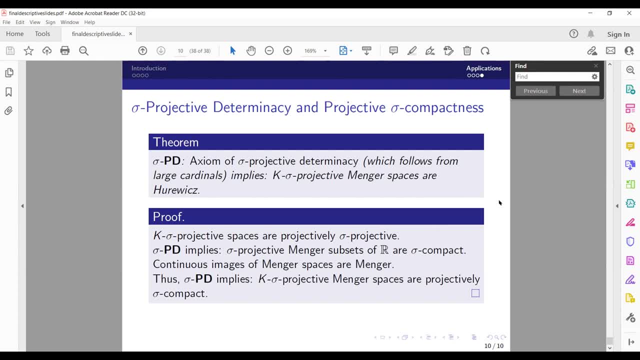 But is there any relation between these notions at all, or is it just superficially similar? Well, both are attempts to, I guess, make definable as wide a class as possible, But, if I remember correctly, aren't universal, aren't universally, bare spaces, subsets of the real? 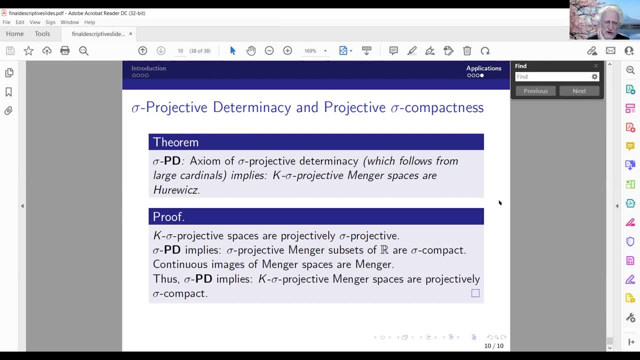 Yeah, exactly So in that sense it's. But what you could do to make the class I'm talking about even bigger is look at the K universally bare spaces, You know just like. Oh right, I didn't have to use sigma projective, that just seemed the easiest, most natural collection of definable subsets of the reals to use. 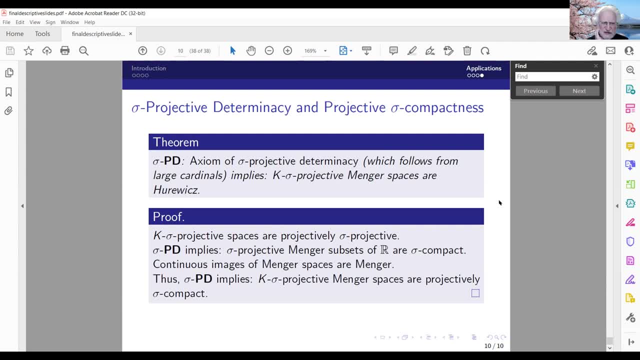 But I could have used those subspaces of the reals which are in L of R, for example, and then use projectively L of R to get an even larger class of spaces. So you know why not projectively K, universally bare spaces, is a perfectly reasonable thing to think about. 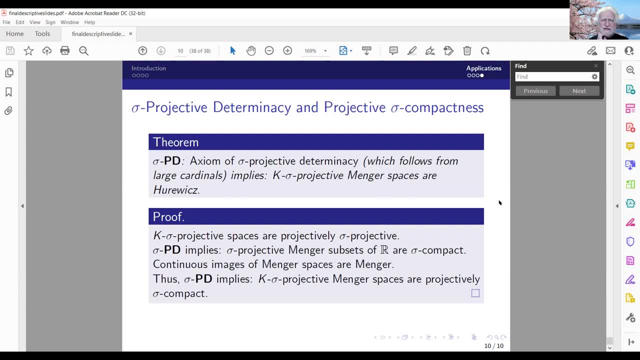 I don't know about universally bare, but I do know it is consistent that Let's see that. I believe it's Equally consistent with an inaccessible That Manger subsets of the reals which are an L of R are Sigma compact. 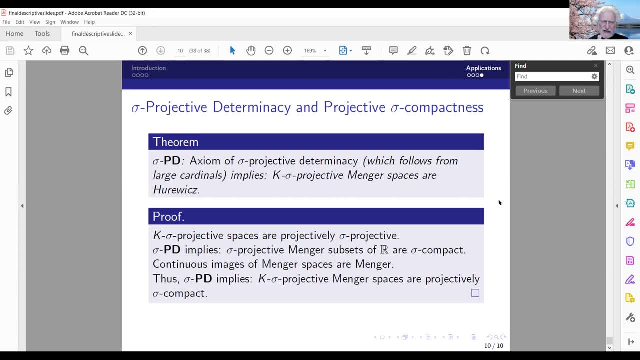 So You are going to get some results for projectively in L of R, I see. Okay, So what I see, So if I'm either began to here, I mean the stuff on capital of the capo which is quite popular these days. 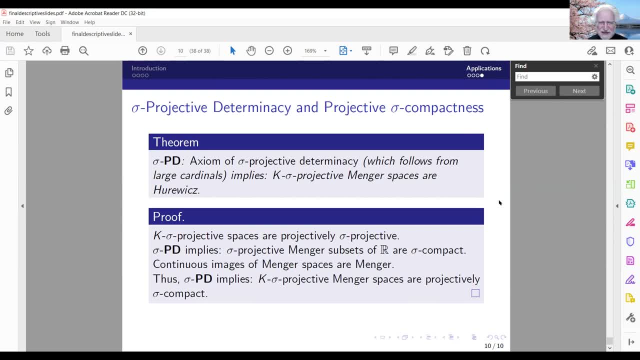 It's interesting set theoretically, but are there any applications anywhere else? I don't know, But here we At least have a chance of applications elsewhere. Right, Are there any other questions? Okay, So I think the next speaker is even on, guy Valverde, and I think it's kind of a continuation of this talk, isn't it? 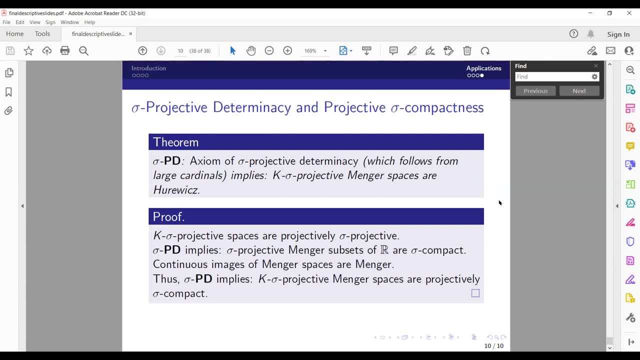 All right, Even, Okay, Okay. So I think the next speaker is even on guy Valverde and I think it's kind of a continuation of this talk, isn't it? All right, Even, Okay, Okay, Okay. 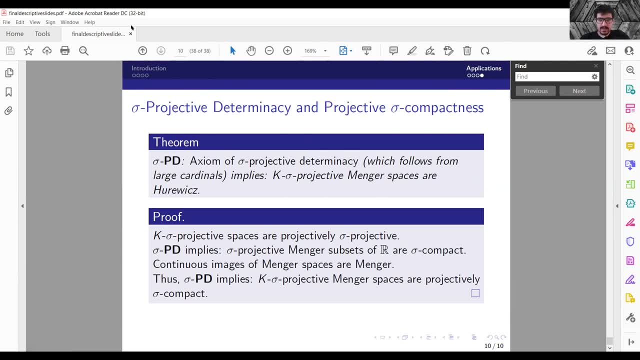 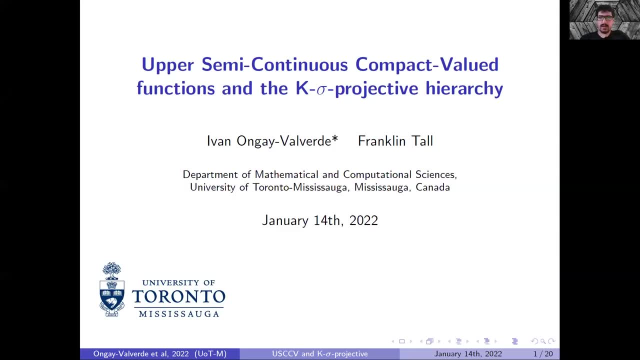 Thank you. Would you share your screen? Yeah, I will start sharing. And so close Franks. Yeah, All right. So the speaker is even On guy Valverde And his title is a person Me: continuous, compact, valued functions. 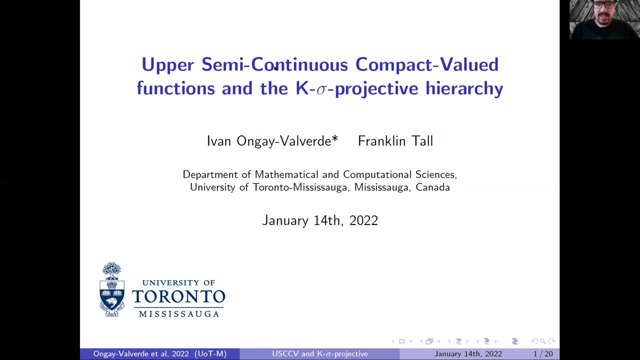 and I'm happy that the seminar was invited to be part of the World Logic Day and I hope everybody is enjoying. And this is a continuation of the last talk And, as Frank announced, I will be talking about the upper semi-continuous compact value functions. 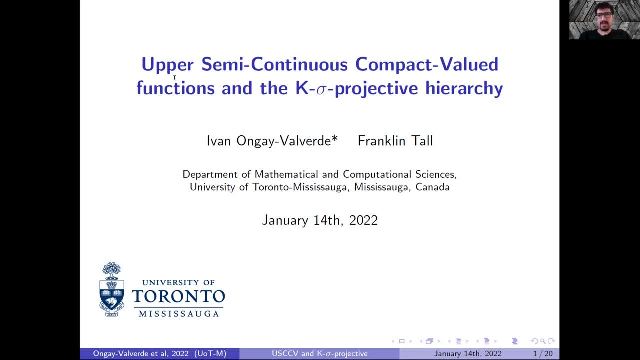 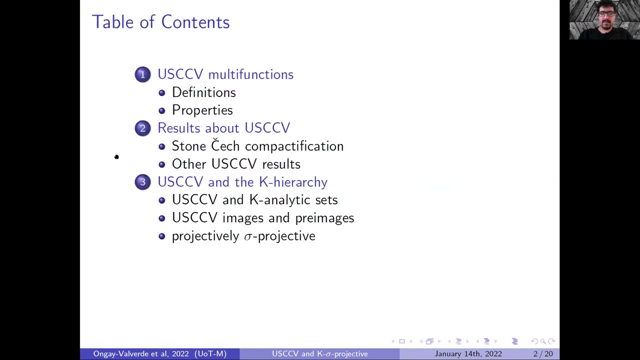 And I will actually define the whole K-sigma projective hierarchy. And at the moment I'm a postdoc, as Frank mentioned, in the University of Toronto, Mississauga, And yeah, thank you very much for being here. So, yeah, so let's start. 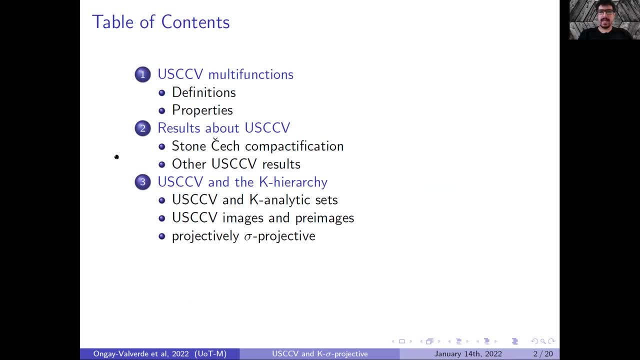 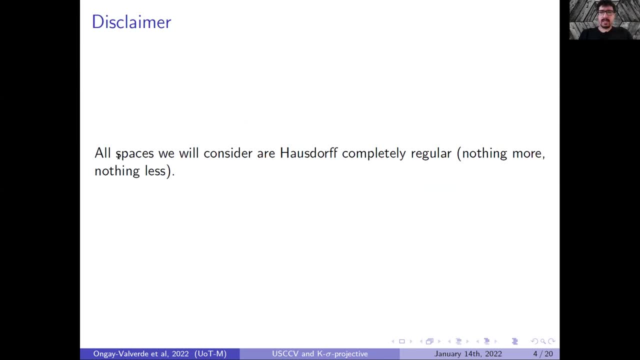 This is the plan for the talk. We will go little by little through it. So first disclaimer: we will be working exclusively with Hausdorff, completely regular spaces. This is to make the stone check compactification nice, because otherwise the space doesn't get included nicely. 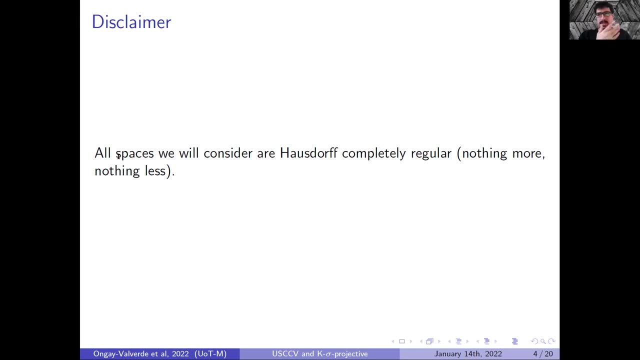 So there's an assumption that I will not mention again, but it has gone to be in the background. So first definitions. So we will talk about multi functions, which I mean it's a function that goes from X to Y, but instead of selecting H'' and putting it down, 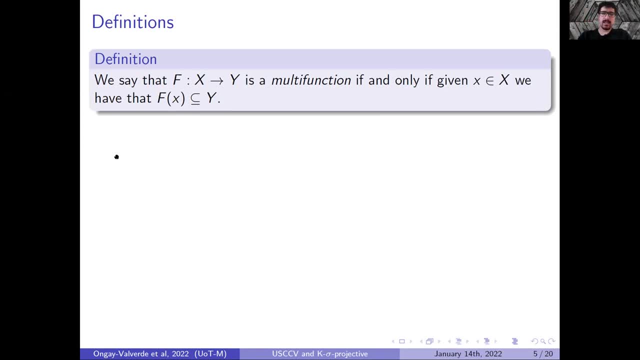 selecting a point, you select a subset of y. Now you can be thinking: okay, why don't we describe it as a function to the power set? And the reason is that mentally it is really useful to think it as a function to the space, because then you can use again the topology of the space. 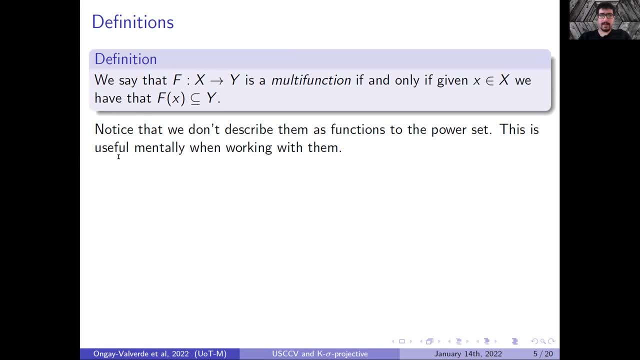 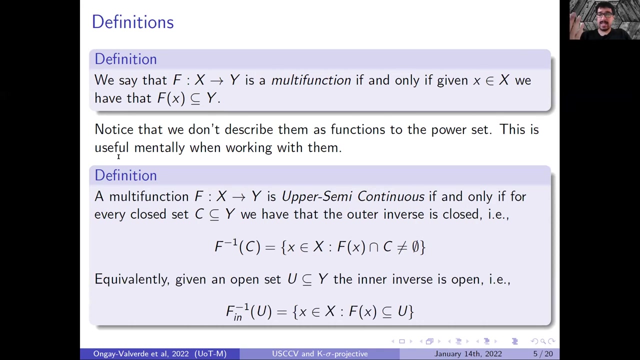 We will see an example soon about that. Okay Now, a multifunction is upper semi-continuous Whenever the outer inverse, those are everything that intersects certain set of a closed set, is closed, And this is equivalent to say that the inner inverse of an open set is open. 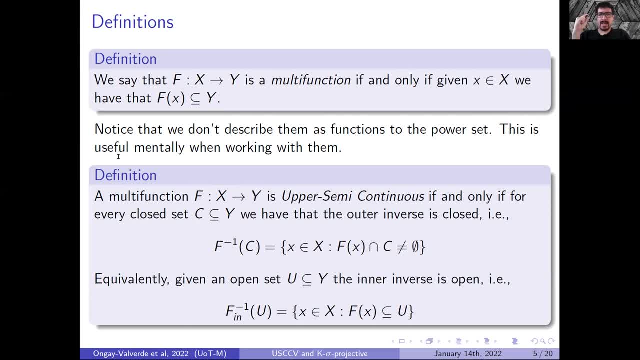 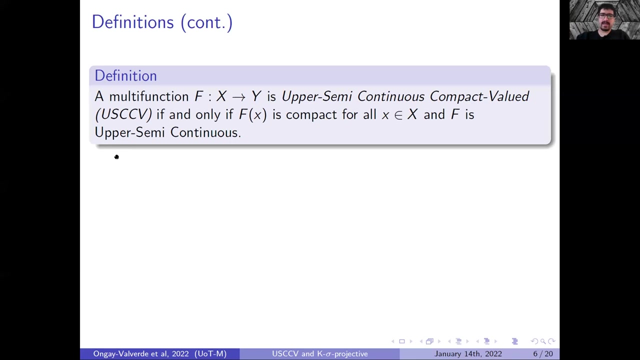 Now notice that for single valued functions, like the usual functions, the outer inverse and the inner inverse are the same, And this is just continuity. Okay, So a little more definitions. So we say that a function is upper semi-continuous compact value, And I will be using the term USCCV because 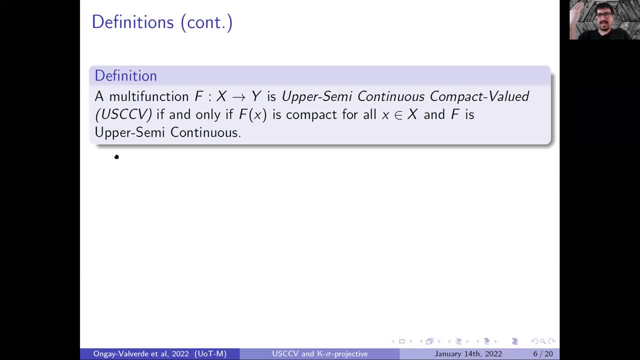 the other one is a mouthful, So whenever it is upper semi-continuous and for each point you assign a compact set. Now this is the first example where I say that it's useful to think of the topology of the space y, because we say that a multifunction is closed whenever the image has like the union of all the 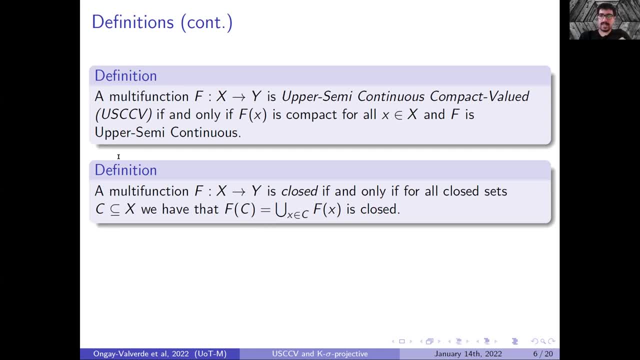 points in C of a closed set is closed, And this is just like translating the idea from closed functions And we're using the topology on y. And finally, we say that a multifunction is perfect USCCV, whenever of course it is USCCV, it is a closed function And the preimages of singletons. 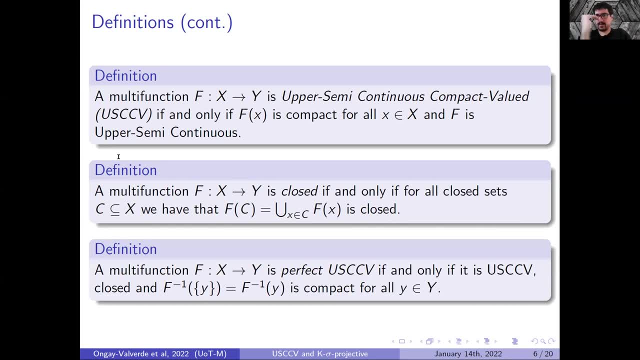 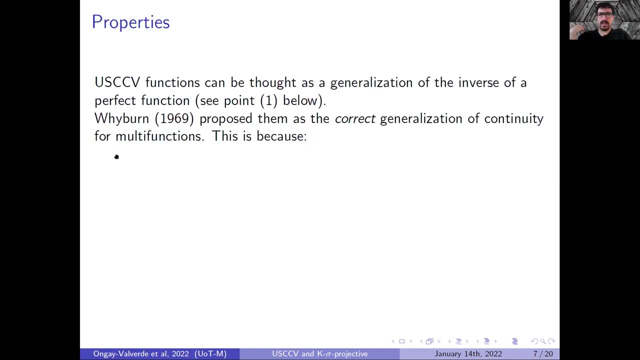 the preimages of points are compact for everything. Once again, this is the same definition as with usual functions. A perfect function is the same, because that is a function instead of a multifunction. Okay, so why talk about them? So, as you can notice, I mean points are compact. 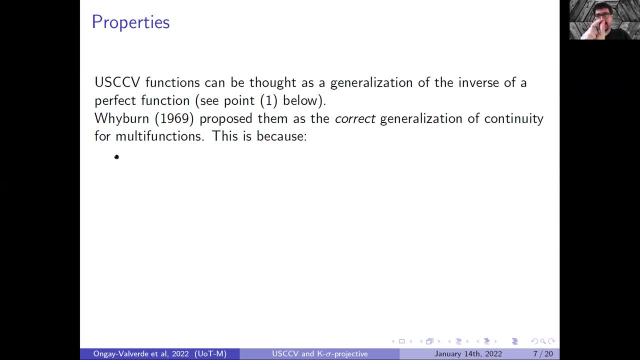 So asking for a multifunction to select compact subsets can be seen as a nice generalization, And this was also think as a generalization of the inverse of a perfect function Wyborn in 1969 actually makes a whole argument about saying that this is the correct generalization. 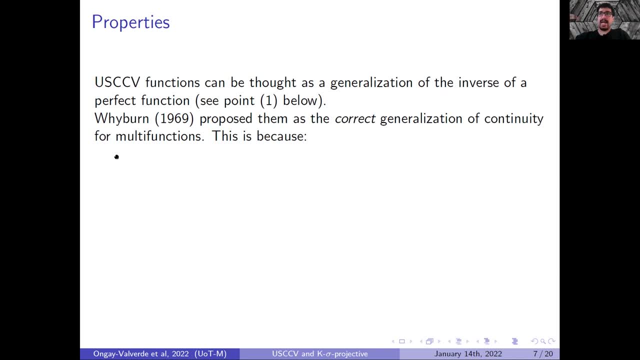 of continuity And in his paper he argues that the generalization of the inverse of a multifunction is called multifunction and other things like that, that it's a better way to describe some results. Can I think of this as a topology on the space of compact sets? 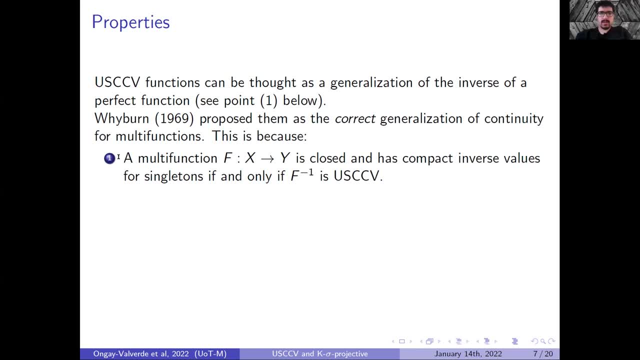 You could, but I will not be super sure. how do you translate that? Okay, I'm sorry. Okay, I mean, I'm sure there's a way to do it, but it's usually just thought as the topology in one. Okay. 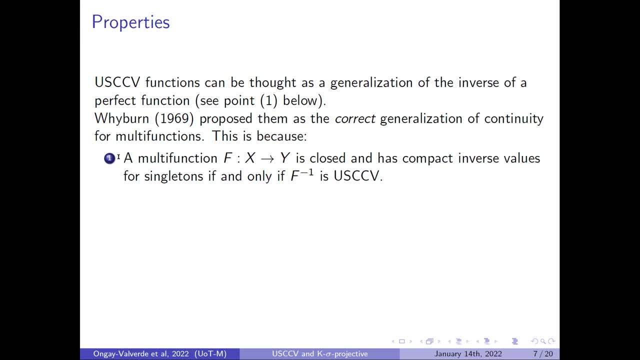 And for example, I mean the reason this is a generalization of inverse, of perfect functions- is the result of Wyborn That a multifunction, even if it has no continuity property, if it's close and has compact inverse values, then the outer inverse is different. 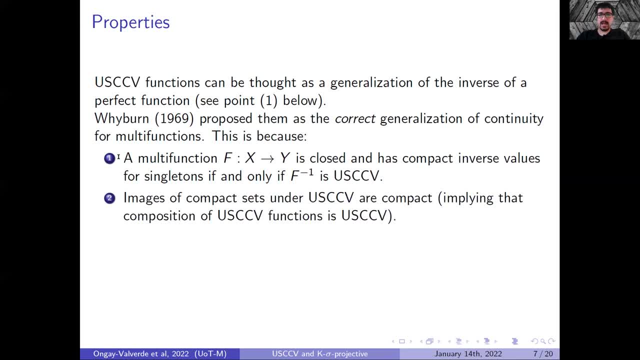 So that's why the generalization of compact sets is called U-S-E-C-V- Okay. Also, the images of compact sets on their U-S-E-C-V functions are compact, which means that when you put them together, like when, like composition of U-S-E-C-V functions. 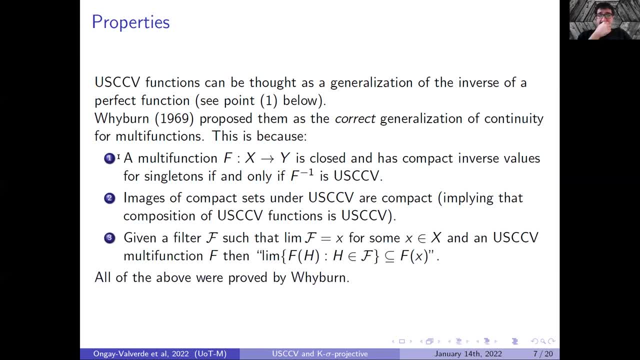 is actually U-S-E-C-V. And finally, I mean, if you remember, for metric spaces, like if you have a sequence that converges to a point, then the image of the sequence converges to the image of the point And Wyborn's show using filters. 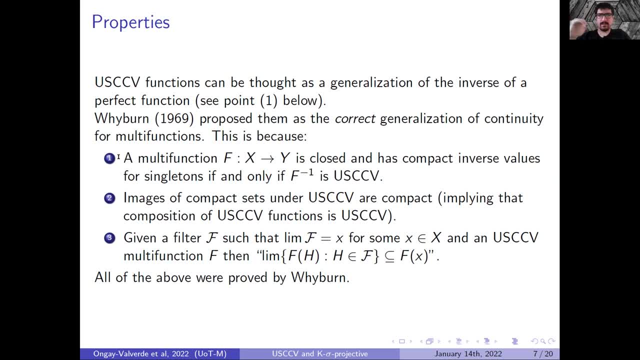 although he doesn't mention that word, it's a little like weird notation, but he's essentially saying that if you have a filter that converges to a point, then the accumulation points of the image of the filter are contained in the image of the point. 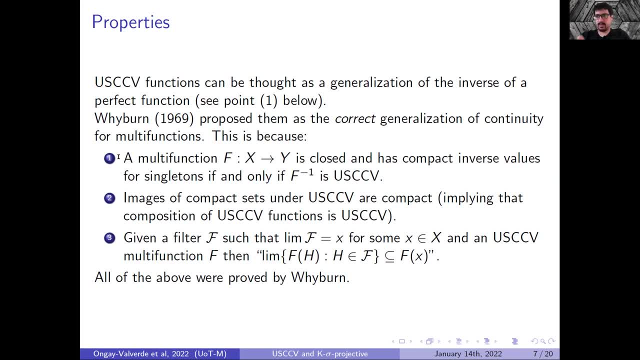 And you can do examples that make that contention proper, but it's still the same idea that somehow you get. you are getting closer to the image of the limit. Okay, And all of these were proved by Wyborn in that paper. Okay, 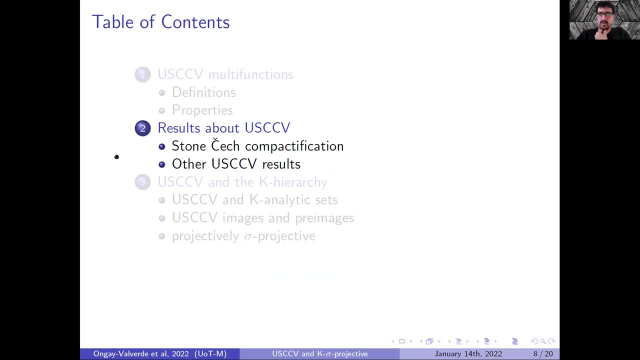 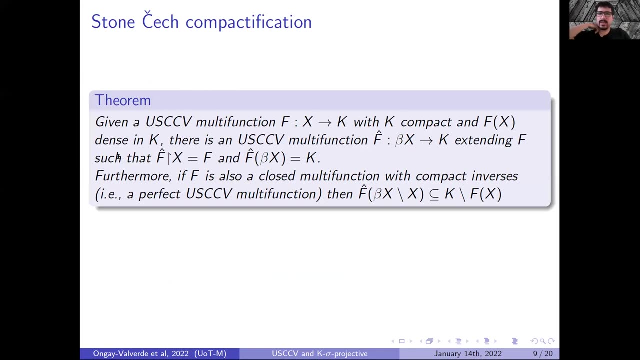 And actually you can get more about these U-S-E-C-V functions. The first part- and, as Frank mentioned, we will be working a lot with the stone check- compactification. It turns out that you also have this same theorem of extension, that if you have a function from any space to a compact set. 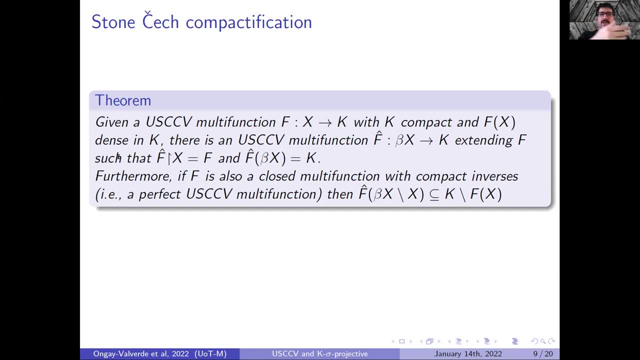 then you can extend- I mean not continuously, but U-S-E-C-V-ing- the function to the whole stone check thing And furthermore- and this is also part of the classic theorem- if it is a perfect U-S-E-C-V multifunction. 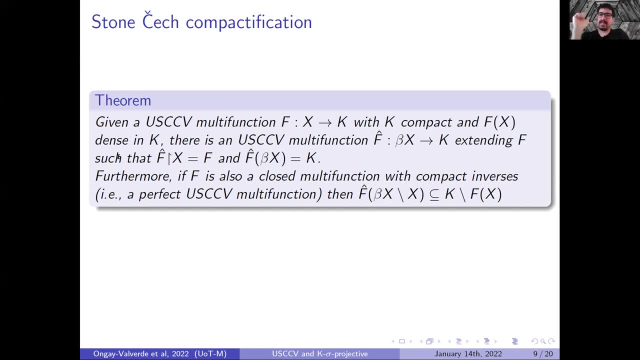 then the image of the compliment goes to the compliment of the image of the usual set. Okay, Now, something interesting about this proof is that once you go through it, you- actually we don't use anything special about the stone check compactification. 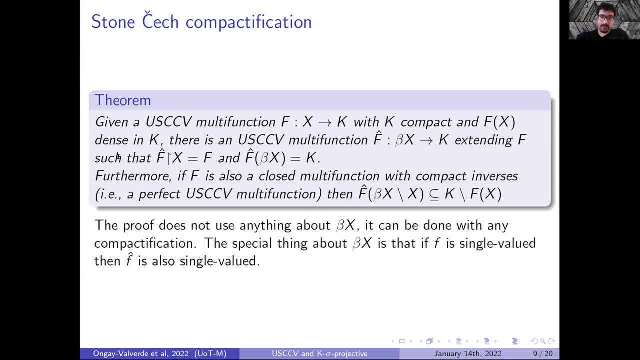 But once you think about it, what is special about the stone check compactification is that whenever you have a single value function, the extension is also a single value. I am not really good with category theory, but I'm not sure if this can be expressed. 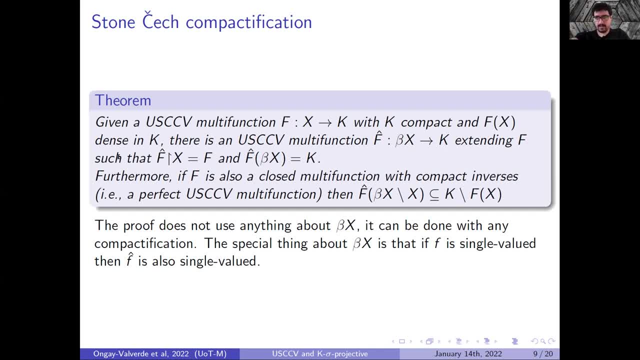 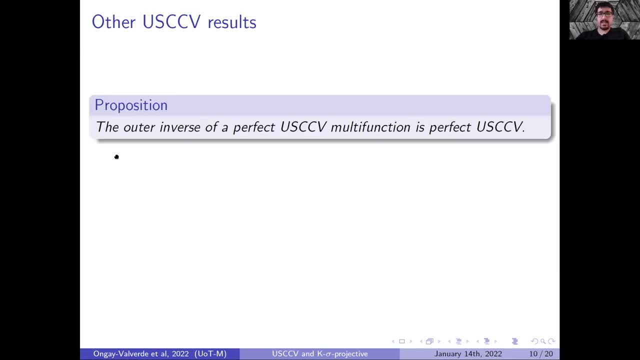 as a universal property in the realm of you know, like compact spaces, spaces and USCCD functions, multifunctions. Now, another nice property is that the outer inverse of a perfect USCCD function is perfect USCCD. 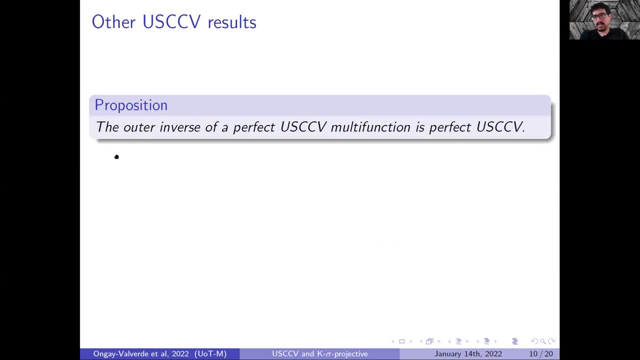 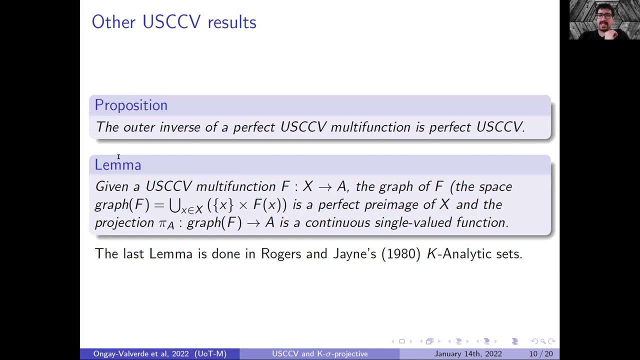 which, given the first result of Wyvern, should not be impressive because he had almost this for without continuity. So you kind of get everything little by little And finally this lemma turns out to be more important than one will think, because USCCD multifunctions. 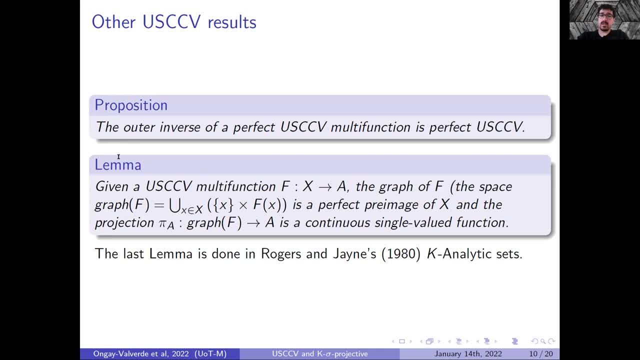 can be translated to useful functions. So what you do is you look at the graph space, which is just what you imagine. You put each point across the compact set you are taking as image, you union all of them and it turns out that this space 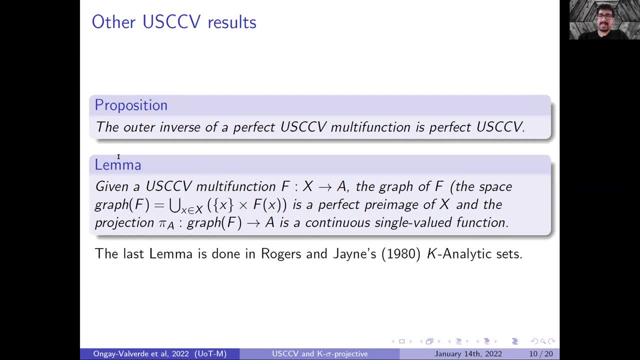 is the perfect pre-image of X, And then A is going to be a single, a continuous image of this space. okay, And this lemma was shown by Rogers and Jane in 1980 in a chapter of a book that is called K-Analytic Cells. 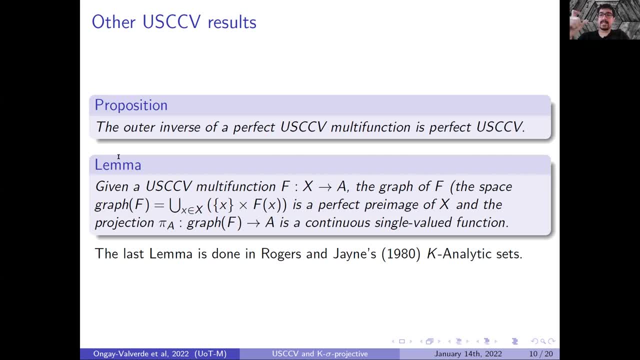 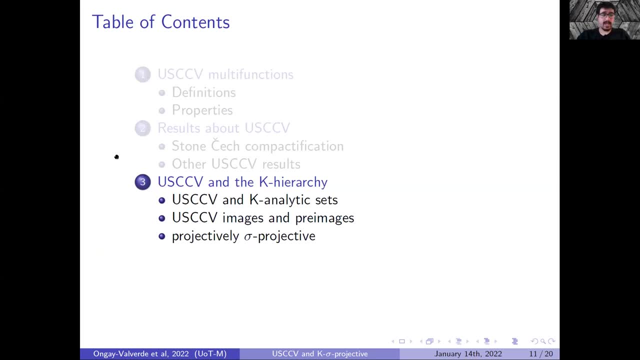 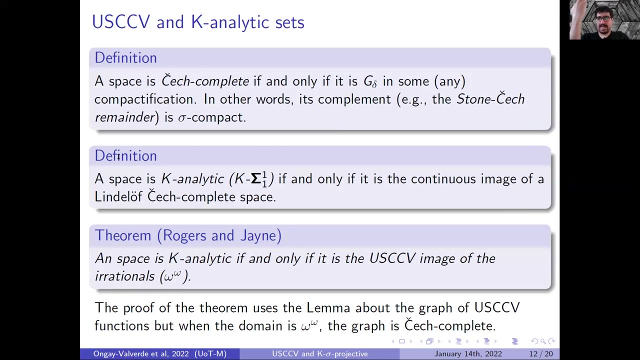 And this is essentially how they prove that the equivalence of definitions for K-Analytic Cells that Frank mentioned, which we will actually talk about them right now. So, as Frank and the space is check, complete if, and only if, it is G Delta in some or any of. 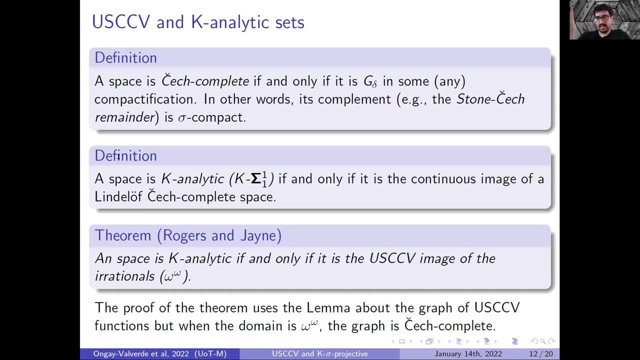 that is actually any of their compactifications. As Frank mentioned, it is, it is generalizing being completely matrixable and being locally compact, right, On the other hand? okay, so then a definition, as Frank said, is that a space is K-Analytic. 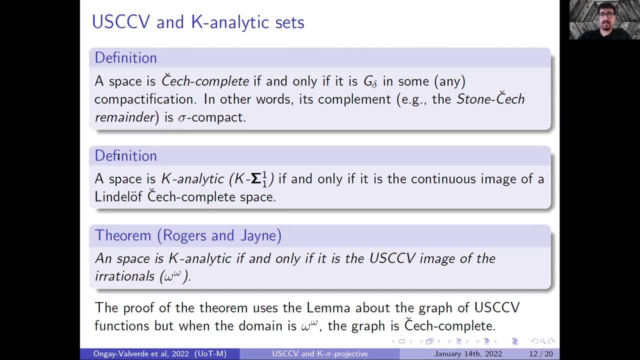 if and only if. it is a continuous image of how Lindelof check complete the space And Rogers and Jane show that this is equivalent of being the USCCB image of the rationals of omega to the omega For one side of the proof. 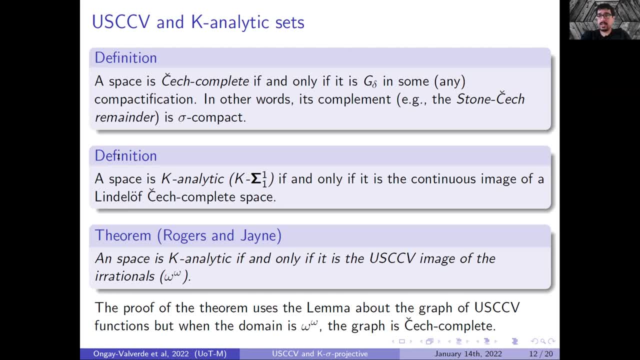 they use this lemma or the graph of the USCCB function And because the graph is the perfect preimage and omega to the omega is check complete, the perfect preimage is also going to be check complete. They don't know, They don't prove it that way. 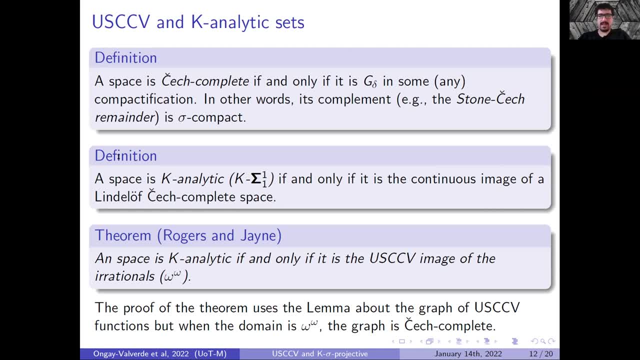 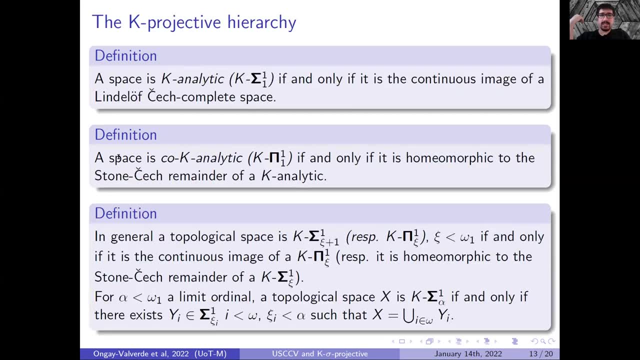 They go to earlier definitions, but that would be like the simpler proof. Okay, So now we can continue defining everything. So we have defined k-analytic as frank. Okay, so this definition for co-k-analytic of or k pi, one one is different from frank. 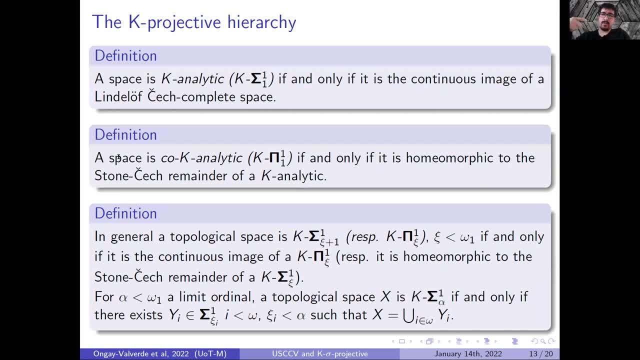 because what I'm saying is that the space is homeomorphic to a stone check reminder of a k-analytic, The way Frank defined it. he was saying that the stone check reminder of the space was k-analytic, But I will show in a second that is the same right. 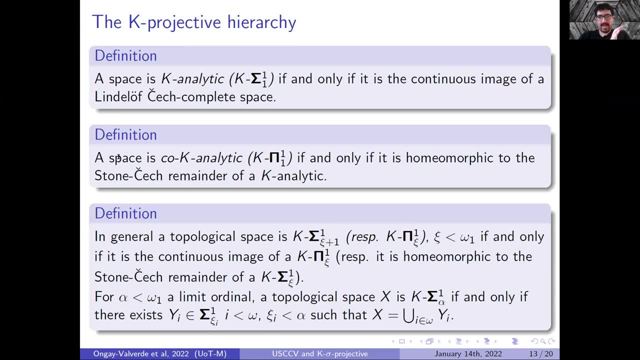 So it is a pretty nice way to. I mean, the hierarchy behaves pretty well and then you continue defining it as frank. Like the sigma, powers are going to be continuous images of the pi parts and the pi parts are going to be compliments of the sigmas. 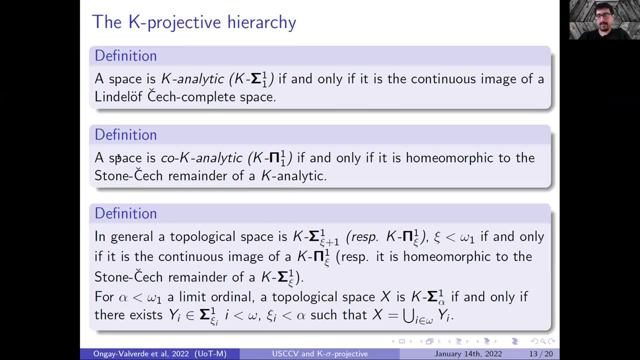 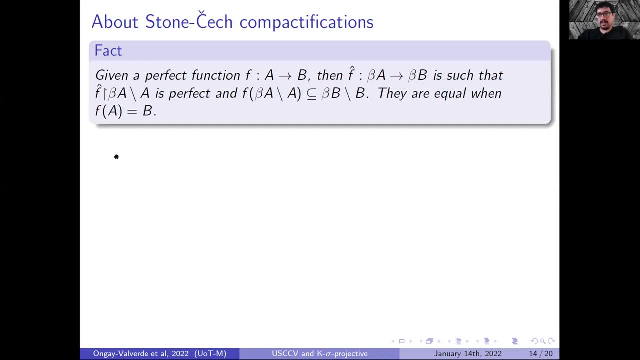 Okay, And at limits you just take units, countable units, Okay. So this is a quick reminder before our first move. So remember that classically, given a perfect function, you can't just take any function from A to B If you take the stone, check on identification of A. 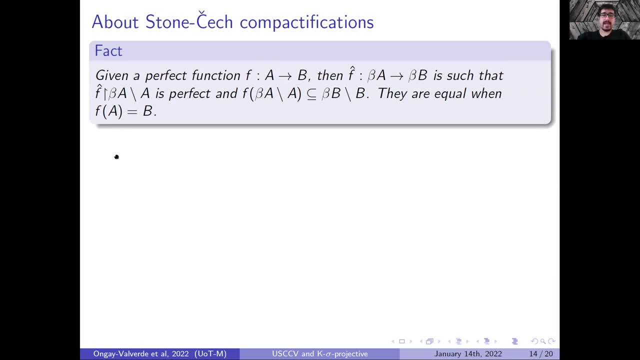 and any compactification or people, let's say also the stone, check one and then the function restrict, the image is perfect And to the couple of means, perfect and it goes inside the complex, the, also the reminder. So reminders goes to reminders and they are actually equal. 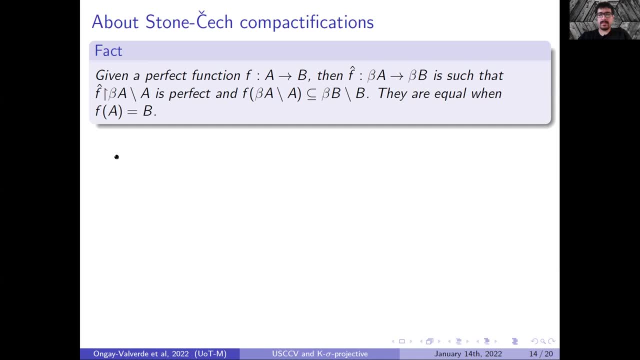 Okay, Okay, when the image is all of it. So the lemma is that, given a k pi one, one space, the reminder is k analytic. So how do we do this? By definition, there should be a space a, k analytic, space y. 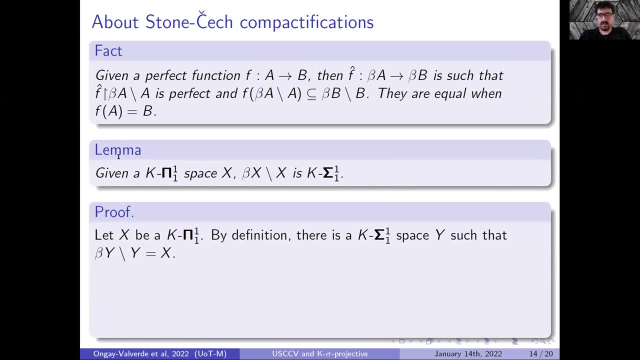 such that the stone check reminder is x. It's a mnemorphic, but let's say it's x, Then the closure of x in that space is a compactification of x. So using the above, I mean the above fact, there is this function that is extending everything. 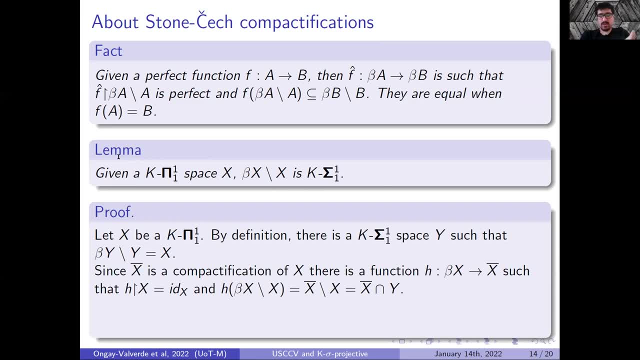 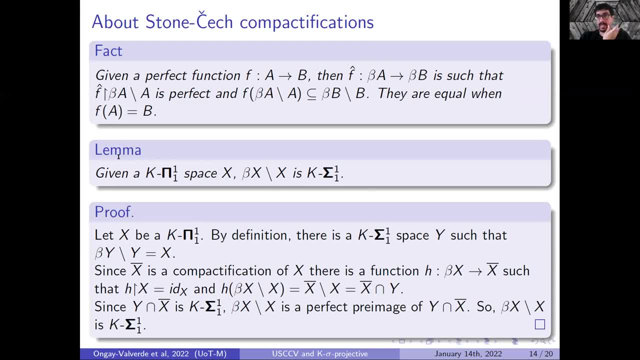 And the reminder goes to: x is the identity. But the class of these classes are pretty nice And you can show that they are close on their. I mean the first, the first, countably many are close on their countable and unions and intersections. 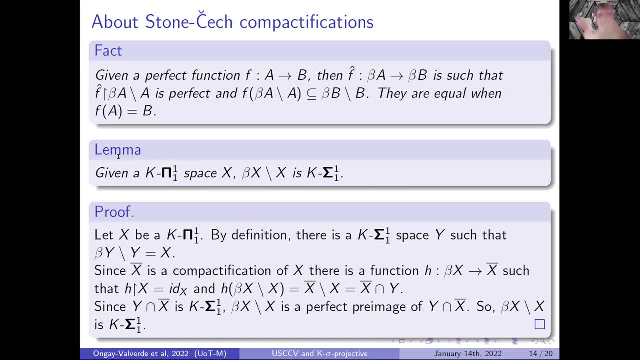 And all the others, at least, are close on their finite ones. So you can take that intersection. It's also going to be k analytic And this is the perfect pre-image of so the compliment is a perfect pre-image of that, And a perfect pre-image is a USCCB function. 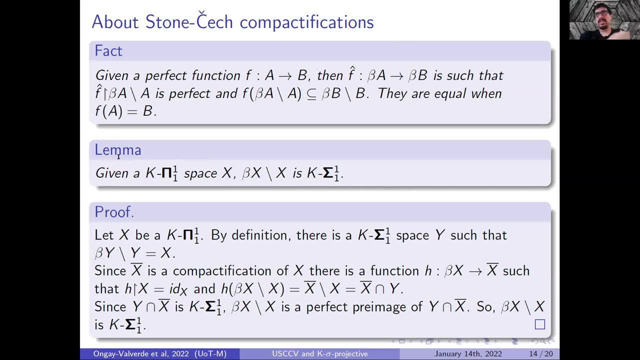 So if this originally was a USCCB image of the rationals, the reminder of x in its stone check compactification is also that, which means that that the reminder is also k-analytic. okay, And this strategy of taking the stone check compactification. 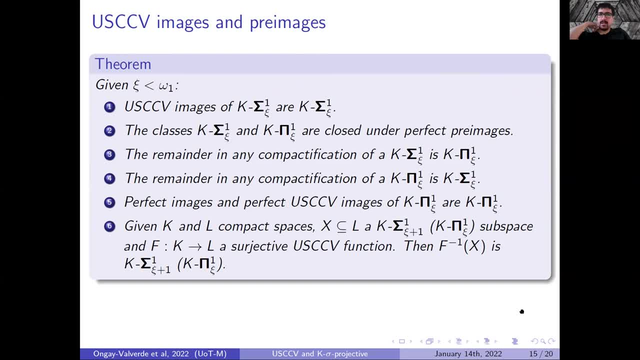 actually lets you prove a lot of things. You can show that all the sigma classes are close on their continuous function and actually on their USCCB function. And you can show that all the classes are close on their on their USCCB images. 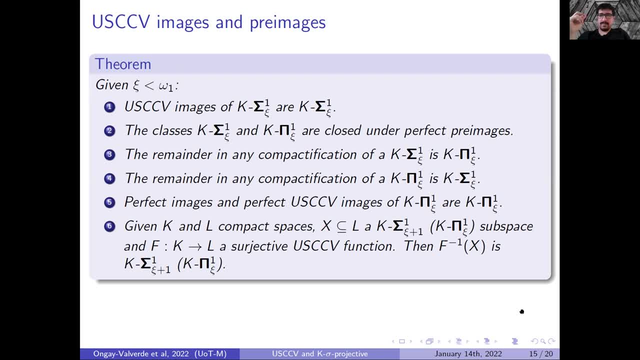 You can show that in any compactification, the reminder is going to be the other class right. For the sigma, it's going to be a pi of the same level. for a pi, it's going to be a sigma, And you can also show that perfect images. 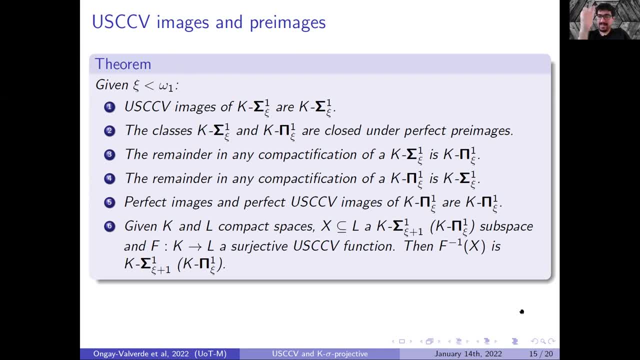 and perfect USCCB images of the pi ones are the corresponding pi ones. okay. And finally, for example, for projective spaces, we have that if there is a function from a positive space to another, then the inverse of an analytic is analytic. 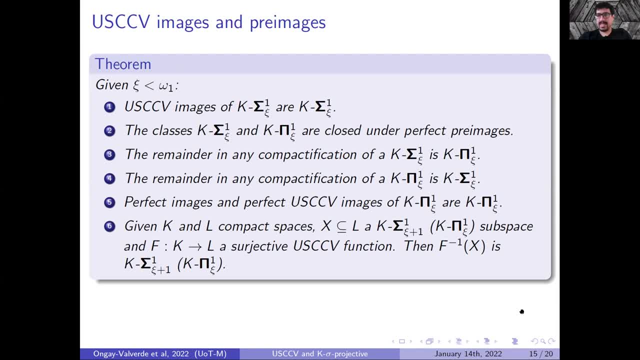 the inverse of a co-analytic is co-analytic and so on, And we get the same. here I put the result with compact spaces. It will also be true with check, complete ones And even maybe with care, analytic ones. 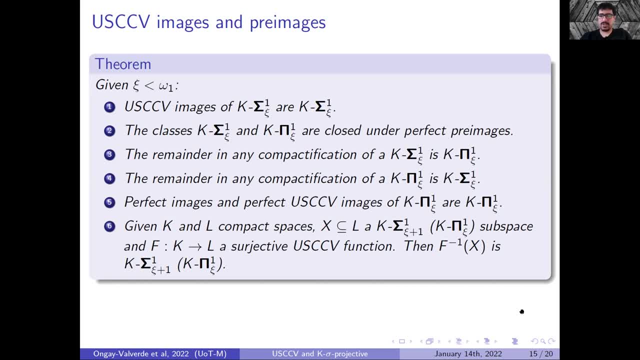 but that is like going a little too much. okay, And most of these proofs use, as I was saying, the stone check extension, and the first one uses the lemma about the graph of USCCB functions. And to finish the talk, 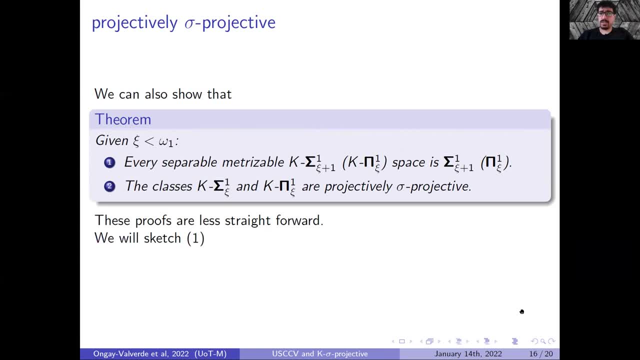 I will show that whenever a K one, I mean whenever one of these K spaces is separable and divisible, it's actually the same level of just projective, of usual projective one. So they are just like subsets of the reals. 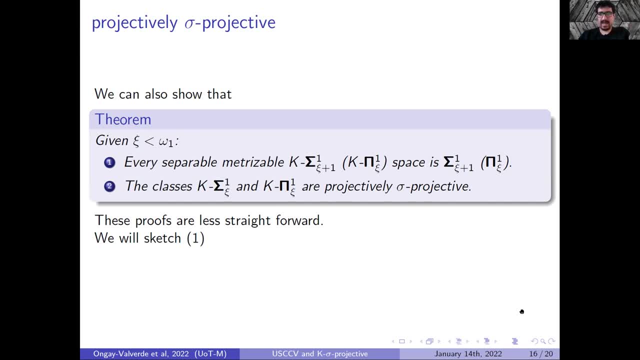 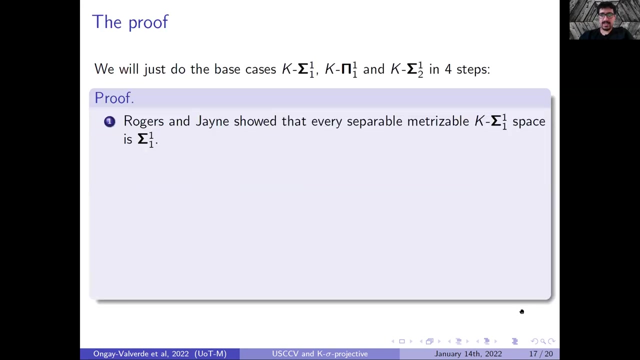 And this implies that the classes are projectively sigma-projective, which was really important for Frank's result. So we will sketch one and then two. just uses that, the closure of these sigma classes under continuous images. So how do we do this? 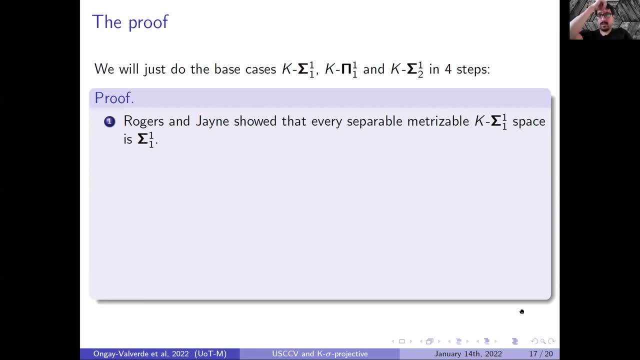 Just to: this is already published, so for for care, analytic, Rogers and Gain already did it, So nothing to do there. Now for the pi ones, and I will just do the base cases, and then everything is going to be clear how to continue. 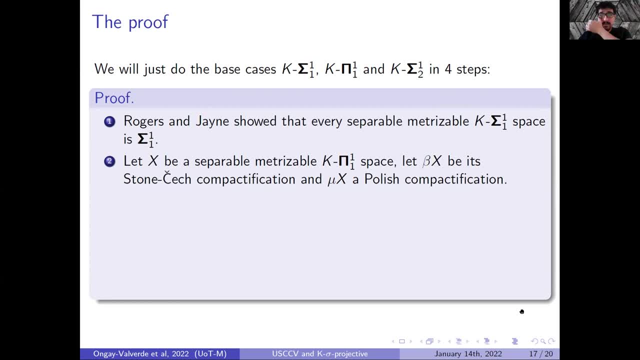 For the pi ones, if one is matriciable, you can look at two compactifications: a stone check one and a polish one. okay, And using again this same property, universal property of the stone check compactification, you get that the complement is care analytic. 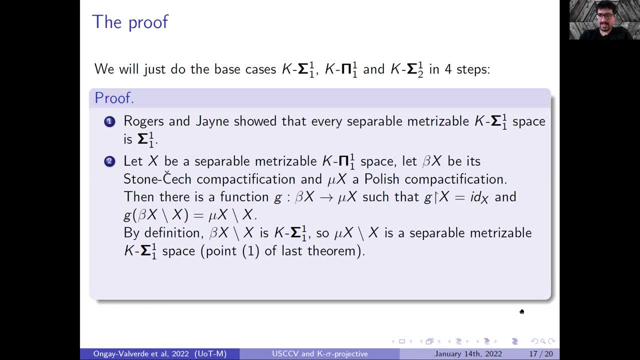 But using point one, if it's care analytic, it's actually analytic, which means that the complement is co-analytic, okay, Which is just pi one one. So we are going to do it. Everything's going well, So now the next step is going to be weird. 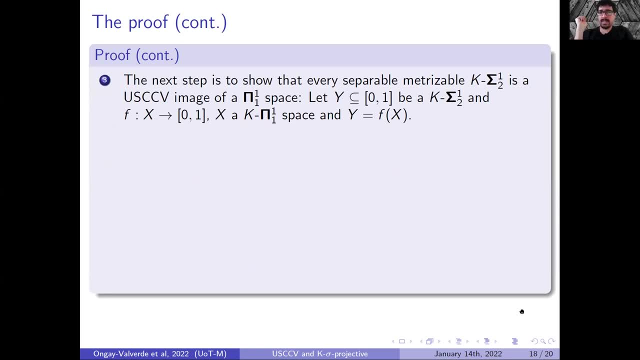 but we're going to do a diagram chase to show that every separable matriciable k sigma one, two space is a USCCB image of a co-analytic space. okay, So we get all the participants of the show with the properties that we want. 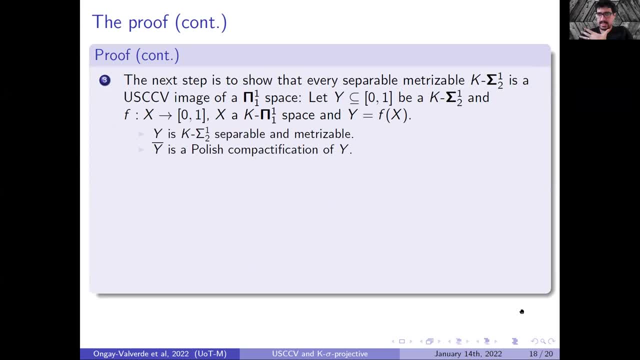 And we start doing the same. We take a polish compactification of y and we extend the function And then we notice that f to the minus one is a perfect USCCB function, from this polish space to beta, to the stone. check. compactification of x. 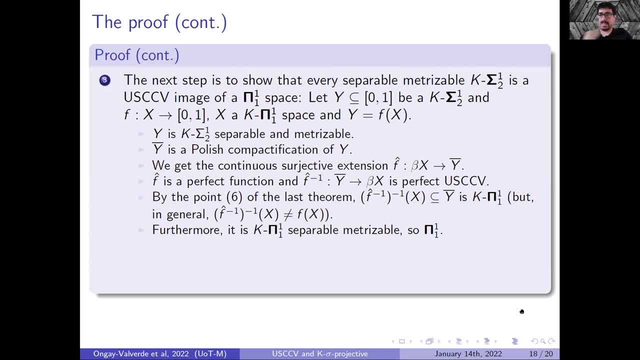 So by 0.6, we get this. So that's the box, And then we have this, so we have x. of the last theorem, like the one about pre-images, The pre-image of x is k, pi, one one, And that pre-image may not be the same as f of x. 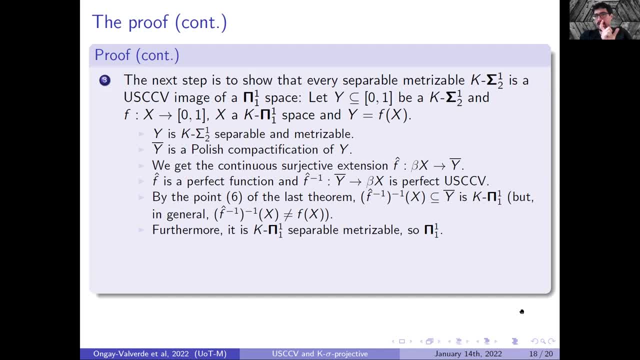 because, remember, that is the outer inverse, So there can be like more stuff like around. So, furthermore, So this pretty much is going to be K, co-K, analytic, separable, matrixable, So it is co-analytic And again doing the diagram chase. 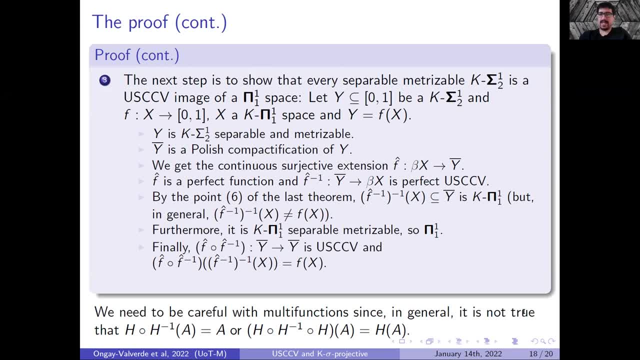 you can notice that this I mean taking the inverse and then the function, the hat function. you take this co-analytic space, So this co-analytic space to the image that is Y. So we're almost done. 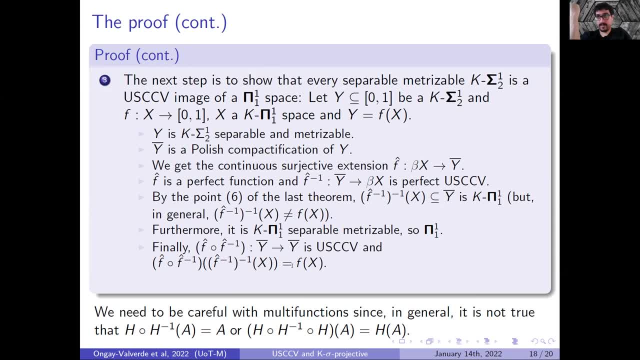 We just need to show that Y is actually an image of a co-analytic, not a USCCB image. Now, in this whole diagram chase, we need to be careful because in general, it is not true that these equalities happen. 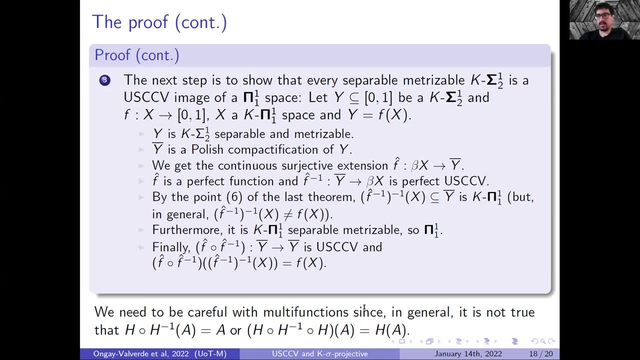 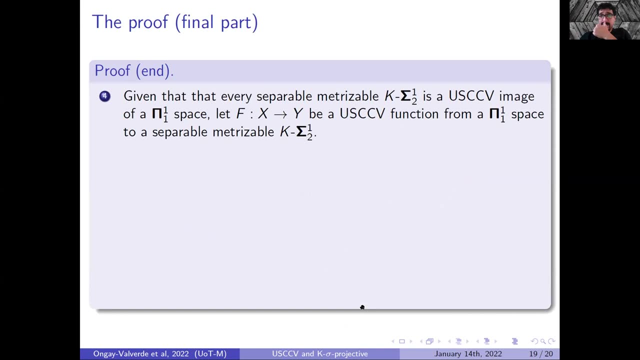 And at least the second one is always true for usual functions. okay, But because the original F hat is a normal function, things work out well. So the final step: we're going to use the graph theorem. So if we have a separable matrixable K, 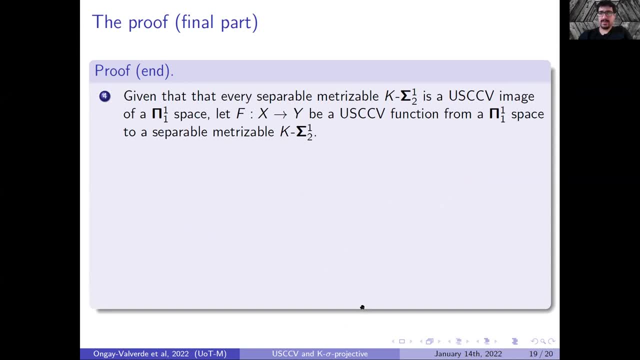 sigma one, two, it is going to be a USCCB image of a co-analytic space. okay, So we take the function, that multi-function, and we know that the graph is going to be a perfect pre-image of this pi one. one thing. 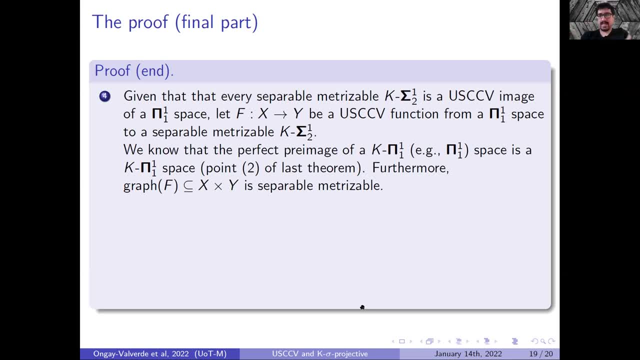 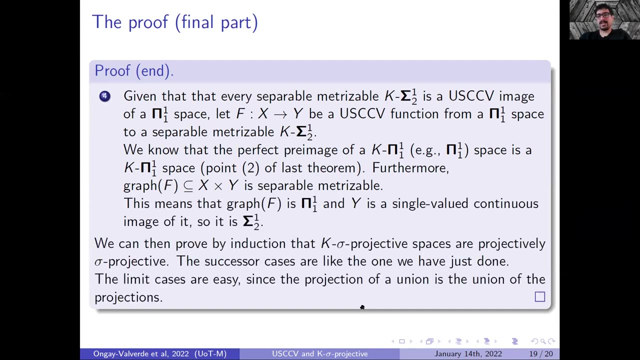 And, furthermore, the graph is going to be inside X times Y. that is matrixable times matrixable. So the image is a K pi one, one space that is separable and traceable. So it is pi one one, which means that Y is the single value. continuous image. 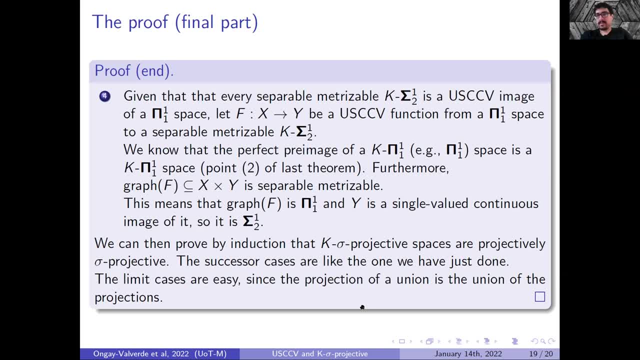 of a co-analytic which make it sigma one, two, And, as you can see, you can from here. then you can repeat the process. You can say: okay, if you have a pi one, two, the complement has to be K, sigma one, two. 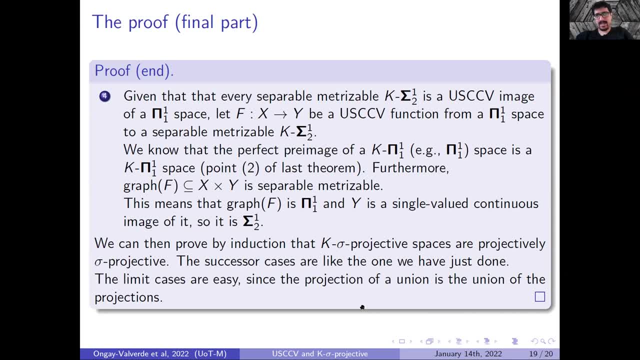 and both of them are matrixable, separable, and so on and on. So the successor cases is just what we did and the limits are easy, because the projection of a union is the union of the predictions. okay, And that will be it. 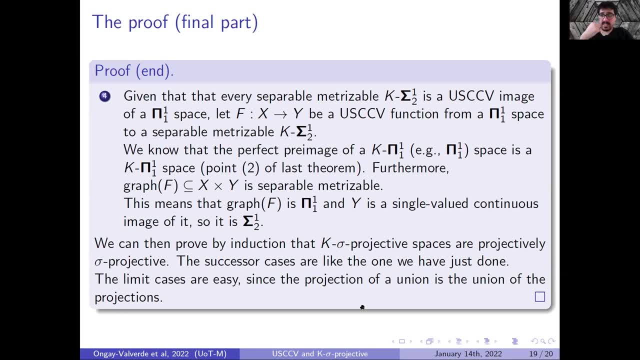 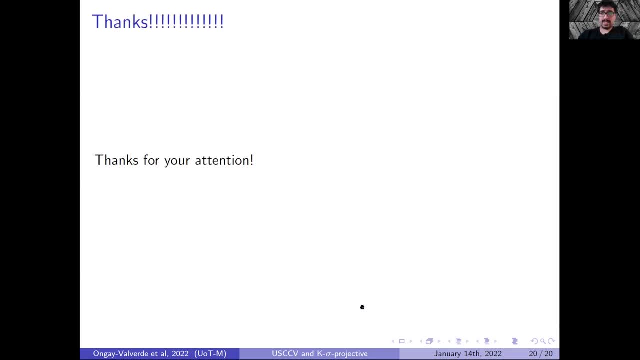 Thank you very much for your attention. Thank you very much, Ivan. Are there any questions for Ivan? I have one. So it seems that you've shown much, much more than Jane and Rogers, but you also said at some point that you 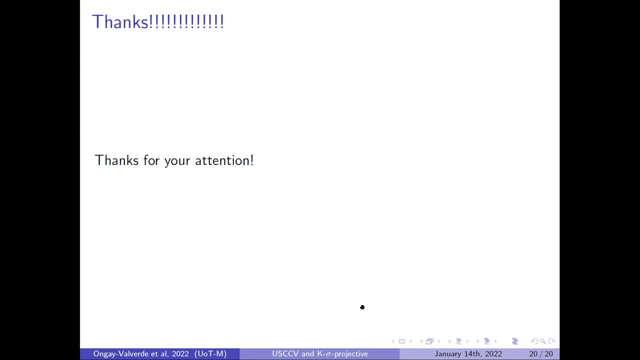 I think you have a simpler proof of some of their theorems. Is that? did I catch that? Yes, Yeah, yeah, yeah, I did mention that Frank and I were talking about it yesterday. Jane and Rogers are analysts. 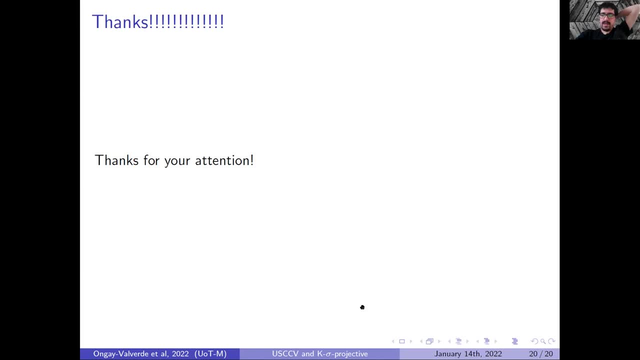 So the way they proved that the graph of a UICCV function with domain omega to the omega is check complete is using the definition of check complete, of having this expression. So it's like a special open set that essentially there are some kinds of convergence, right. 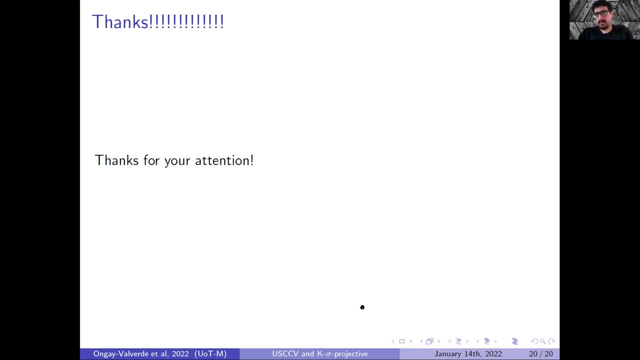 But it would be simpler to use stone-check compactifications and take the perfect pre-image. Are you writing that up somewhere as well? Yeah, Oh, that's great, Okay, Yeah, yeah, Yeah, I'm writing that. I mean in the paper that Frank and I are doing. 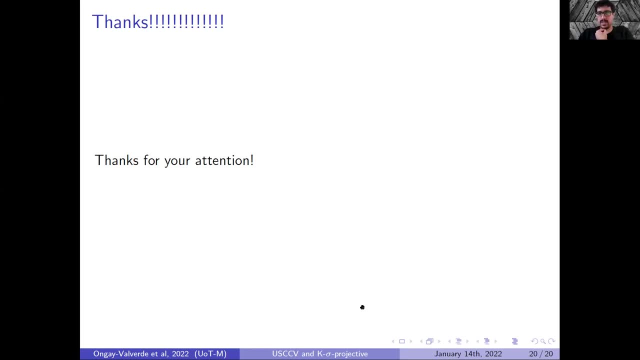 I do want to include that simpler proof. Oh, cool, Nice. And I mean, just as a comment, the way Rogers and Jane show that a K-analytic separable matrixable is just analytic. they use a machinery that is. 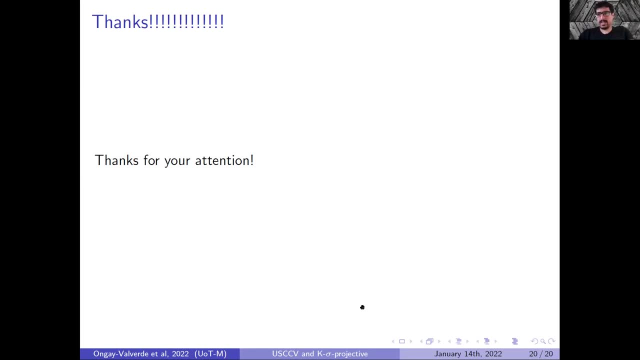 I think it's interesting on its own, but it's kind of complicated. And this same proof the graph works. So it's also a simplification of that. Also, I believe the other one can be used in other contexts, I'm not super sure which ones. 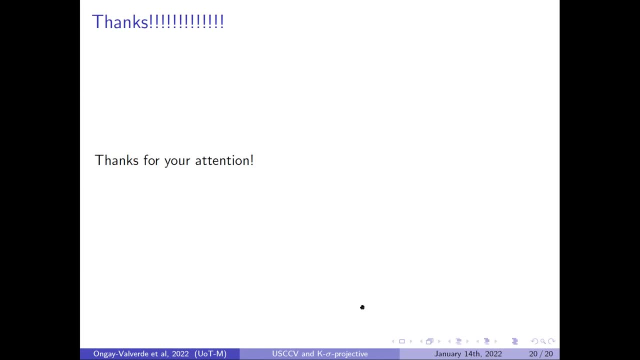 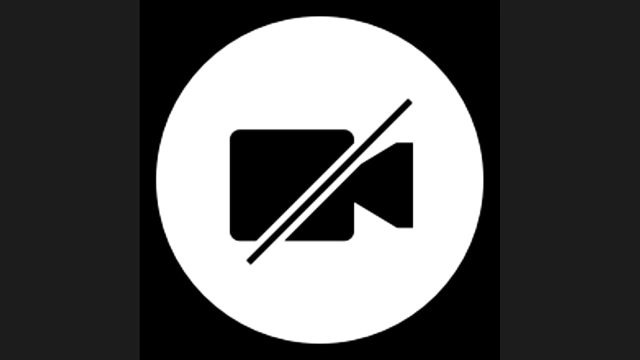 Okay, Thank you. Are there any other questions? All right, Then. thank you again, Ivan, And our next speaker, if I am not mistaken, is Clovis. Is that right? I think so. Yes, Yeah, Then please go ahead and share your screen. 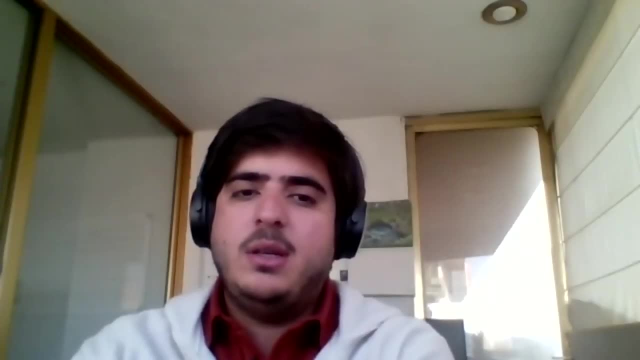 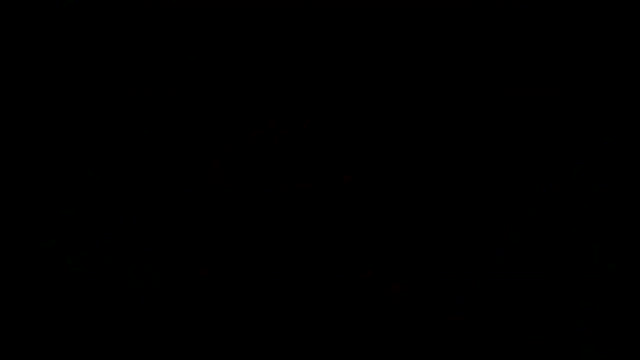 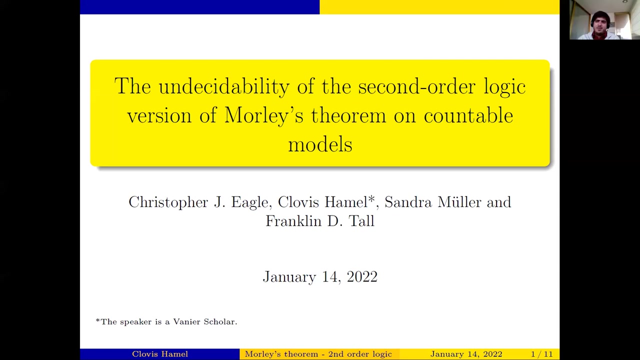 Yeah, The slides are right here, So you should be able to see the slides now. Is that true? They're coming. No, they're not, Just see. Oh, now here they are. Okay, great, Okay, Very good. 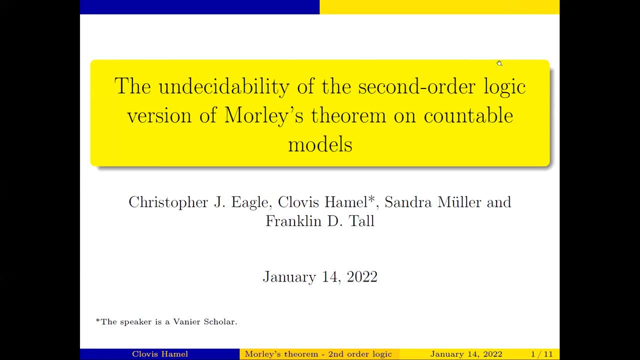 All right, Hi, everyone Go ahead. Yes, Okay, Thanks a lot. So today I'm going to be talking about the undecidability of the second order logic version of Morley's theorem on the number of countable models. 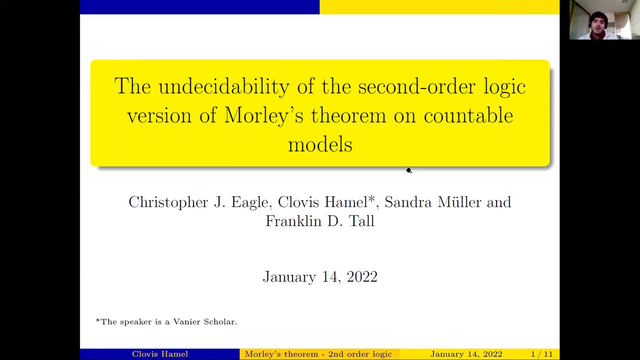 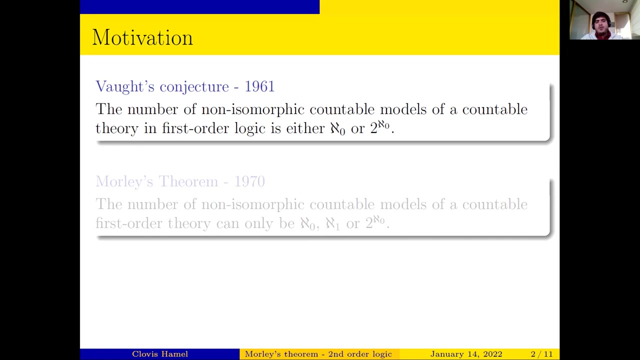 This is joint work with Christopher Eagle, Sandra Mueller and Franklin Toll. Don't mention that Clovis is a graduate student in the seminar. Very good Thanks, All right, So let's get started here. A little bit of motivation. First of all, Voth's conjecture from 1961, which remains one of the main biggest open problems in model theory, claims that the number of non-isomorphic countable models of a countable 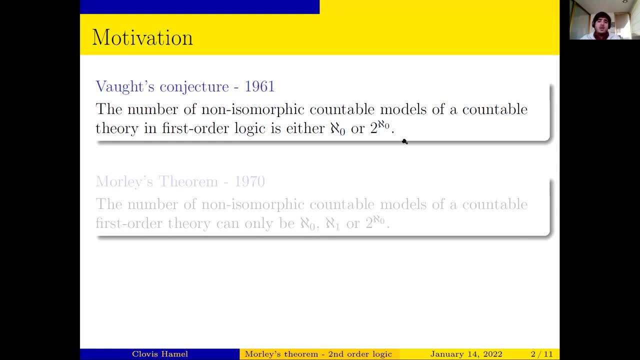 theory, in first order logic is either a left series or a right series, LF0 or the continuum. and now Morley's theorem from 1970 is the best general result known so far, which says that the number of non-isomorphic countable models of a countable first order, 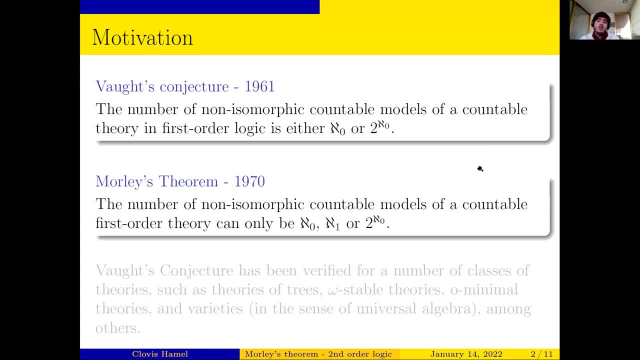 theory can only be LF0, LF1 or 2 to the LF0.. For specific cases, what conjecture has already been verified? and this includes theories like the theories of trees, omega, stable theories or minimal theories, and varieties in the sense of universal algebra, among others, Under CH of. 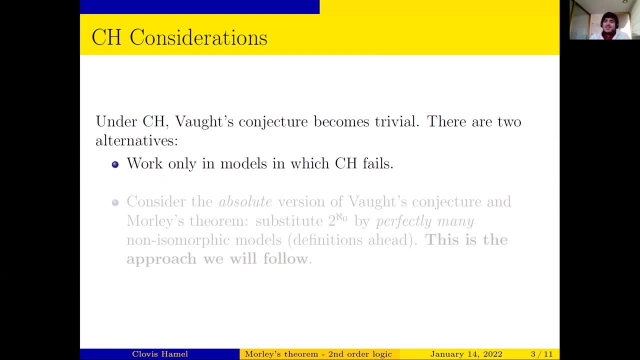 course what conjecture becomes trivial. there is no other option for the number of countable models. so there are two alternatives. the first one is the trivial one, which is only consider what conjecture in Morley's theorem, And the other one, which is the one that we work with, is consider what we call the absolute version. 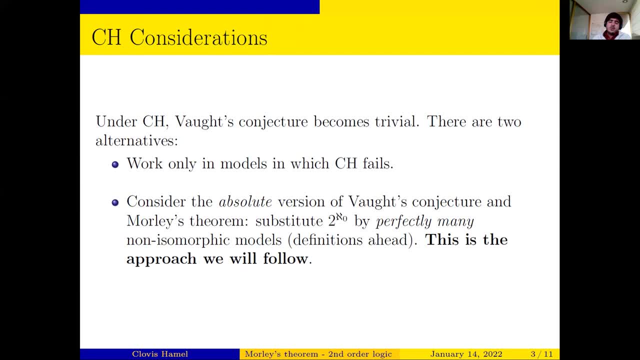 of what's conjecture and Morley's theorem, in which you substitute the continuum by having perfectly many non-isomorphic models. We are going to give the definition in the next slide and this is the approach that we will follow, and we call it absolute because it's independent. 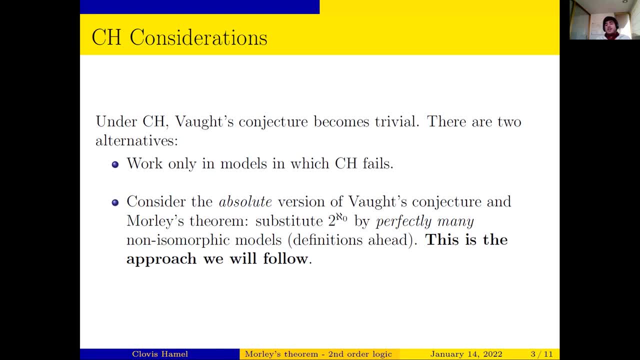 of the truth value of the continuum hypothesis and perhaps originally we wanted to call it the topological vote conjecture, but that that may be mistaken already by people working in descriptive set theory. there is a version for what conjecture with concerns or their equivalence, relations and. 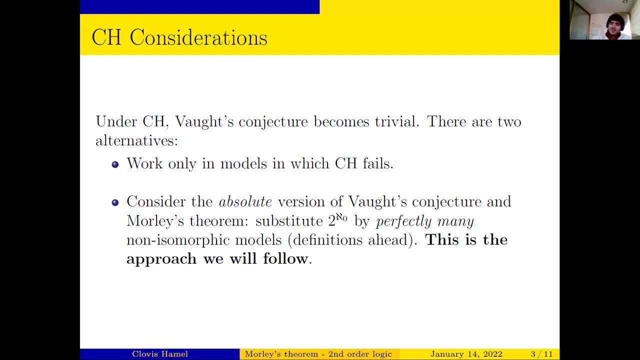 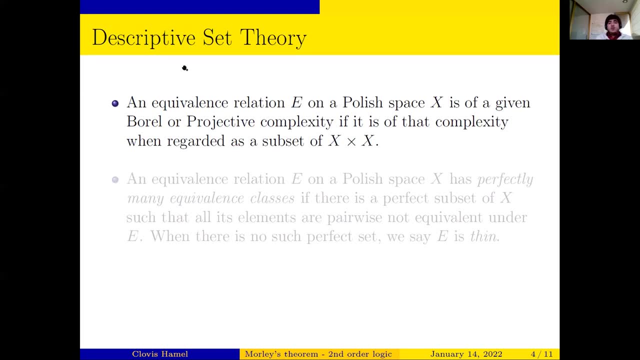 and so we resorted to the absolute name. so a very quick reminder on the descriptive set theory that we are going to be using. we are going to be talking about equivalence relations on the Polish space x, and remember that Polish means separable, completely attriscable, and then such an equivalence relationship is of a given Borel or projective. 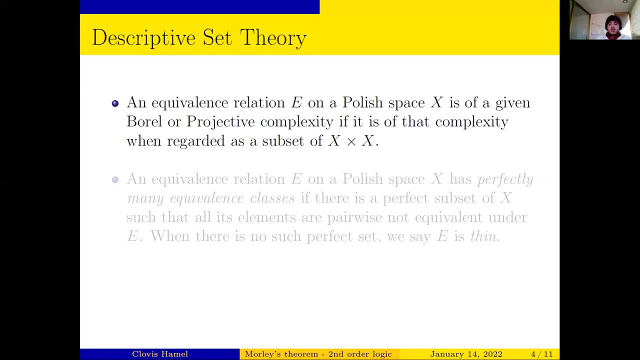 complexity if it is of that complexity when regarded as a subset of x square. and then equivalence relation e on a Polish space x is the derivative of e to the plus x, which is the double part of x squared. Roozbeh Gharakhloo face X has perfectly many equivalence classes. this is the definition that appeared in the previous slide. 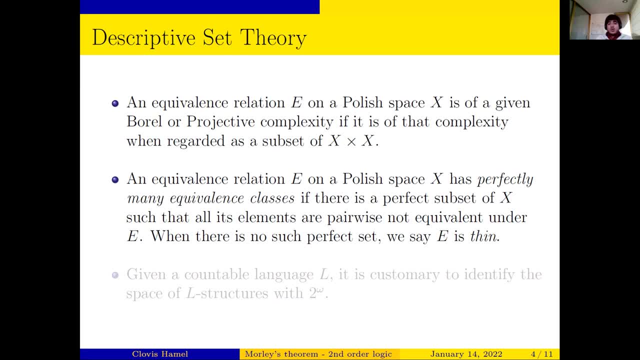 Roozbeh Gharakhloo If there is a perfect subset of X, such that all its elements are pairwise, not equivalent, on their Roozbeh Gharakhloo Such a relation. so when there is no such perfect set, we say that the equivalence relation is thin, and on the other hand, it is something that's very usual in model theory, especially when one is interested in resorting to descriptive set theory to get some results. is that, given a countable language, l? 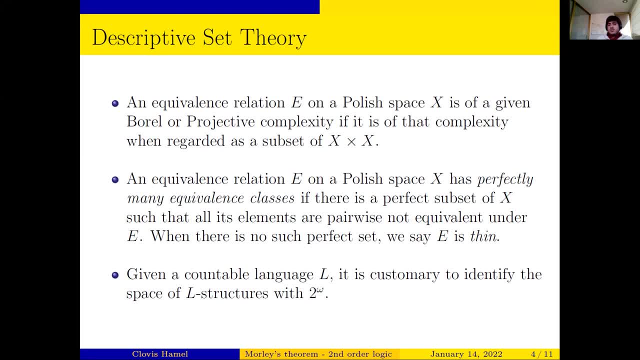 Roozbeh Gharakhloo. It is customary to identify the space of other structures with two terms: Roozbeh Gharakhloo, To be Omega. the way that this is done is by considering to to the product of the artists of the relations in the language. 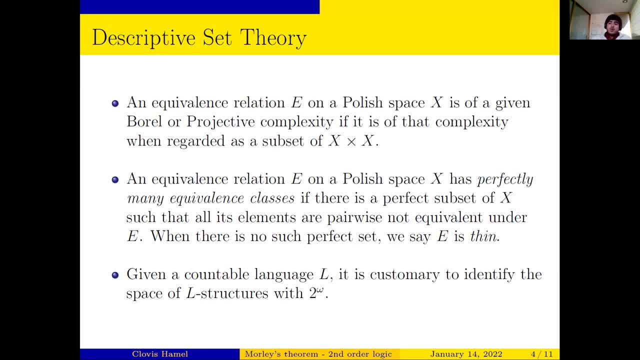 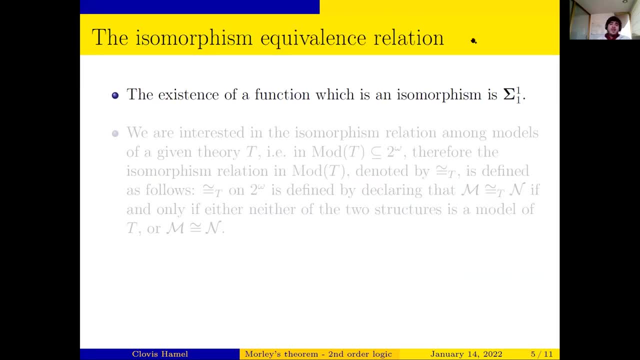 Roozbeh Gharakhloo. We are going to use this identification freely throughout the talk. now let's talk a little bit about the isomorphism relation you're interested in, Roozbeh Gharakhloo, Counting non isomorphic models, both in both conjecture and in Morley's theorem, and the second order version of it that we're going to see. 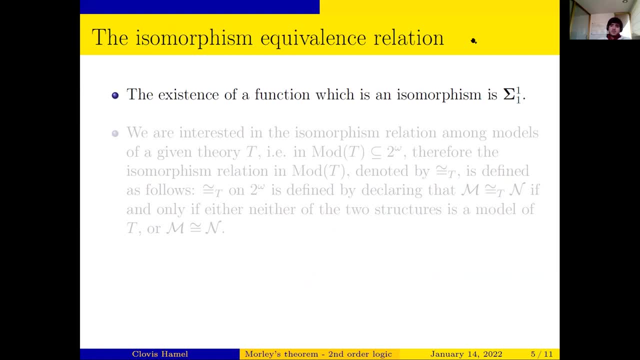 Roozbeh Gharakhloo. That system, Roozbeh Gharakhloo, Of a function which is an isomorphism, is a signal one statement, Roozbeh Gharakhloo. Remember that signal one sets are continuous image of, or else that's. they're also called analytic and 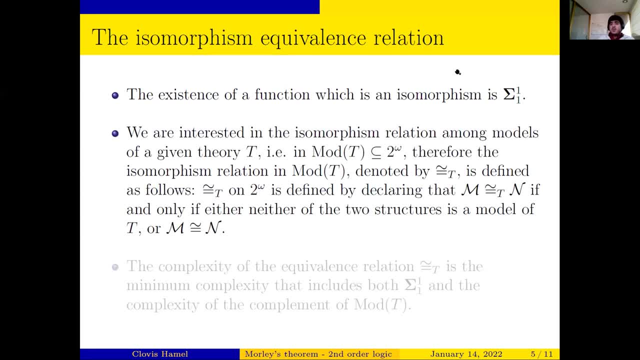 Roozbeh Gharakhloo. This is not precisely what we are interested in. we're interested in the isomorphism relation among models of a glib in theory T, that is to say in the set mod T, which is that of all the models of that theory. 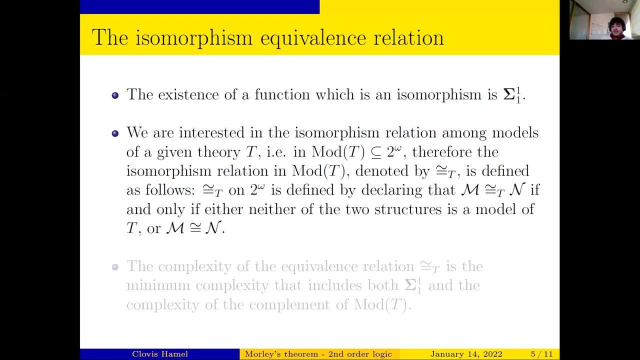 Roozbeh Gharakhloo, Which is, of course, a subset of two to the Omega under the identification in the previous slide, and therefore the isomorphism relation in T, which is denoted like this, is defined as follows: so you declare that two structures are isomorphic with: 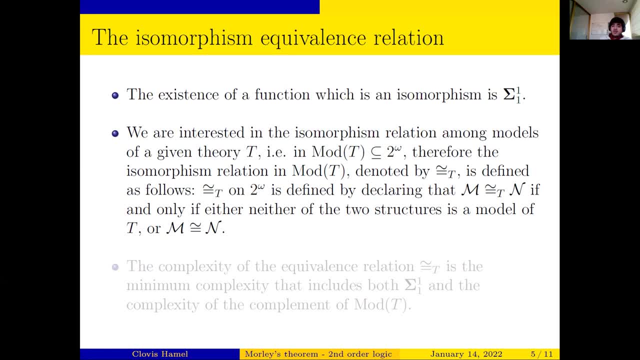 Roozbeh Gharakhloo. Respect to T if, and only if, either neither of the two structures is the model of T or they are simply isomorphic, Roozbeh Gharakhloo. So the idea here, Roozbeh Gharakhloo? The idea here is that we are sending everything that is not a model of T to one equivalence class, and so all we're doing is increasing the number of equivalence classes under this isomorphism relation restricted to T by one, and 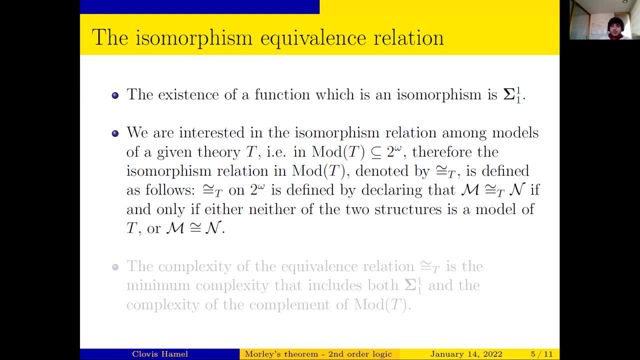 Roozbeh Gharakhloo, On the other hand. well, this is definitely not a problem with this sort of computations of Roozbeh Gharakhloo, The number of countable models that we want to do, but there is a price to pay, and that is to that the definition of this equivalence relation. 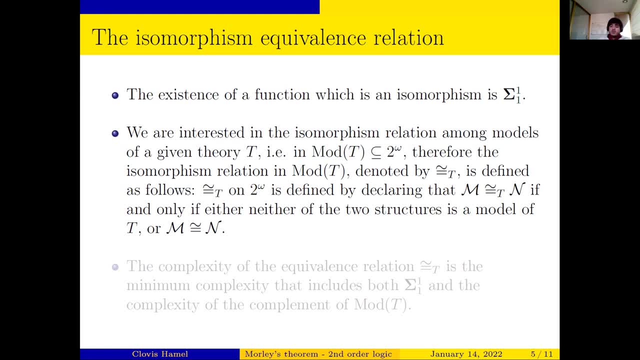 Roozbeh Gharakhloo comes with that of the complement of multi, that is to say, multi appears, a compliment of multi appears, on the definition of this equivalence relation. therefore, the complexity of the equivalence relation that we are interested in is the minimum complexity that includes both Sigma one one. 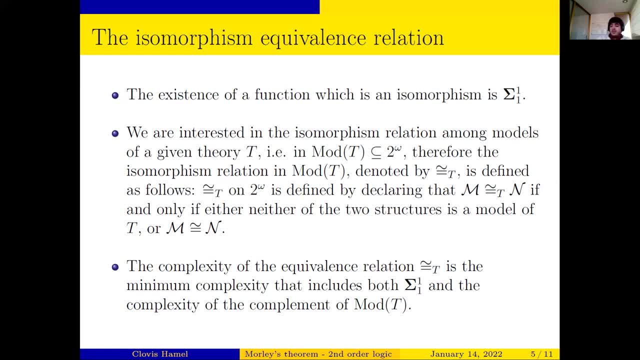 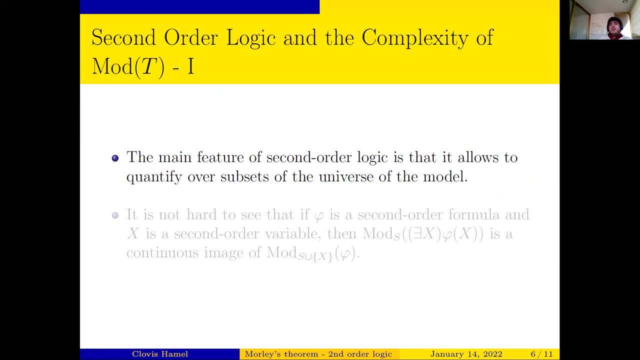 Roozbeh Gharakhloo, And the complexity, Roozbeh Gharakhloo, Of the complement of multi Roozbeh Gharakhloo. So a little bit of what second order logic is about and the complexity of multi is that? well, first of all, the main feature of second order logic is that it allows to quantify over subsets of the universe, of the model. 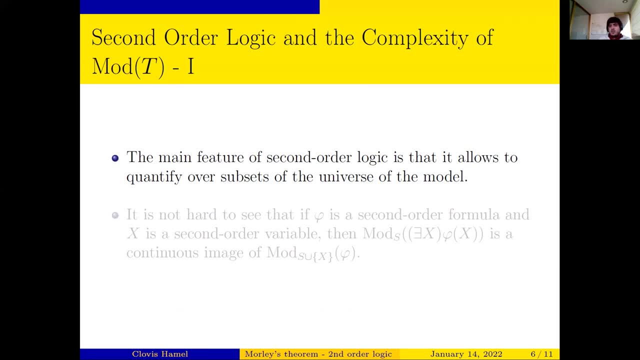 Roozbeh Gharakhloo. Many of us are familiar with this sort of things when we work again in descriptive step theory and we quantify over subsets of Omega Roozbeh Gharakhloo, And there are a few sort of these here that are explaining detail and with examples in the paper I have to link on one of the last slides. 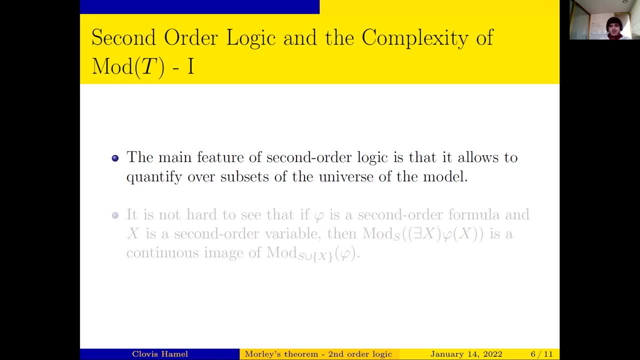 Roozbeh Gharakhloo. But for the purpose of this bridge version of the paper that i'm presenting here, the important part that we know is that what we're working with second order logic and the whole deal is that we can quantify over subsets of the universe. so, having said that, it's not hard to see that, if you have 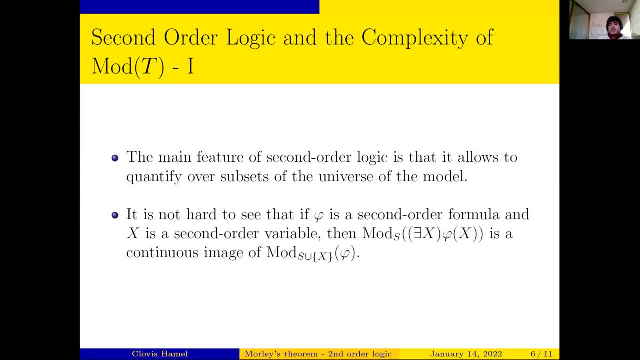 Roozbeh Gharakhloo, A second order formula and X is a second order variable. then when you take a second order existential quantifier in front of the fee that you had, what you're doing in terms of the MOD is taking continuous images. so that's how you come into the projective hierarchy. 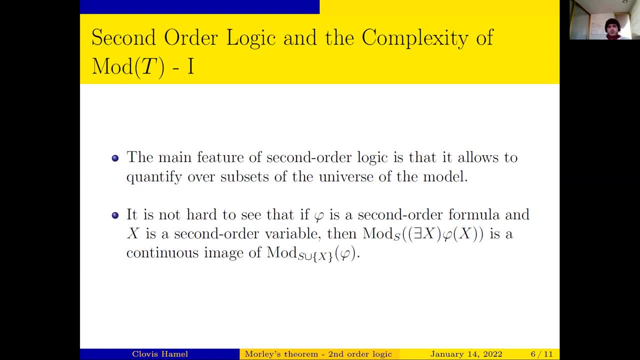 Roozbeh Gharakhloo. In first order logic it's been known for decades- actually that appears also in MOD Roozbeh Gharakhloo Morley's paper- that when you have first order sentences, the models of them are borel. so by taking existential second order quantifiers, we start taking. 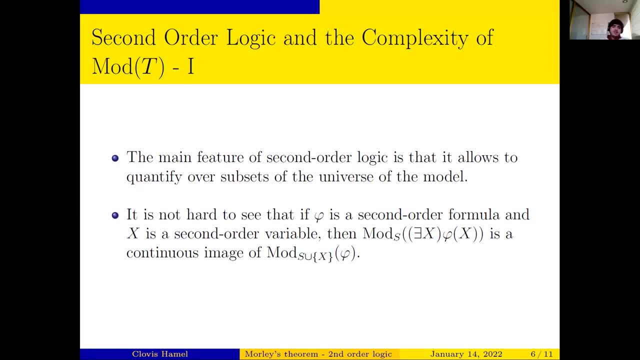 Roozbeh Gharakhloo Images: continuous images. that brings us to analytics, and then, by taking negations, you start moving through the projective hierarchy: Roozbeh Gharakhloo And eventually, if you consider theories, where the Roozbeh Gharakhloo sentences are unbounded in terms of their complexity, you get into the Sigma projective realm that. 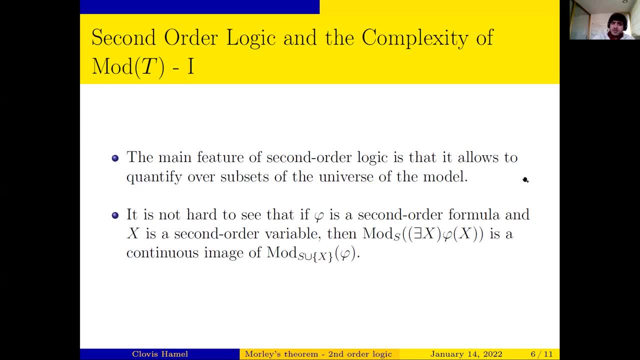 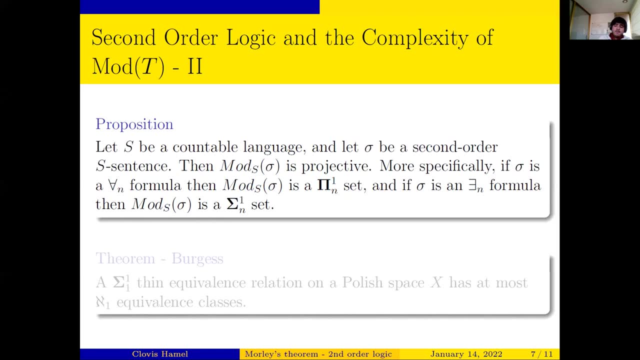 Roozbeh Gharakhloo Even was mentioning Frank were mentioning in the in the previous talks. so Roozbeh Gharakhloo, Having said this, and the main idea is what I just said about second order existential quantification, when you have accountable language and you have second order sentence, then the models of that. 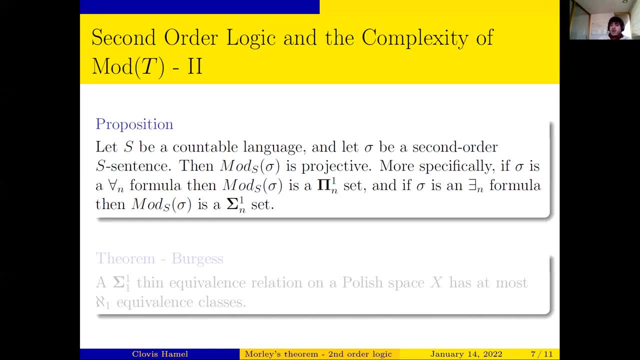 Roozbeh Gharakhloo sentence is a projective set. more specifically, when Sigma is for every end formula, that is to say formula that has n quantifiers and second order quantifiers starting with a universal one, Roozbeh Gharakhloo, Then the models of Sigma is that pi one and send said and you seek mice. there is, and formula that is to say and second order quantifiers starting with an existential one, then mod Sigma is a Sigma one. 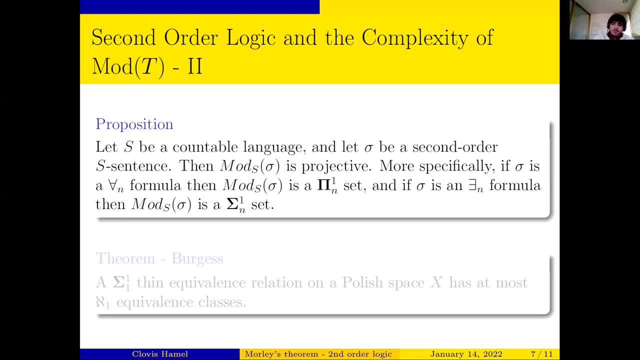 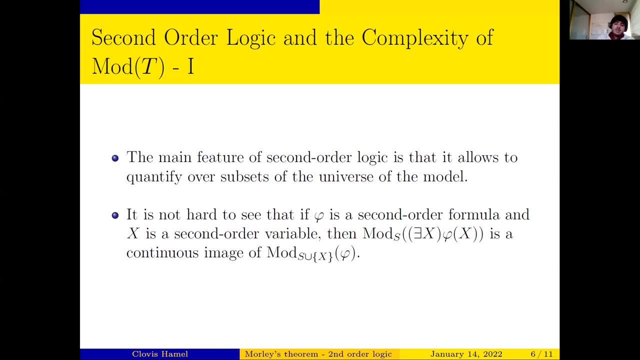 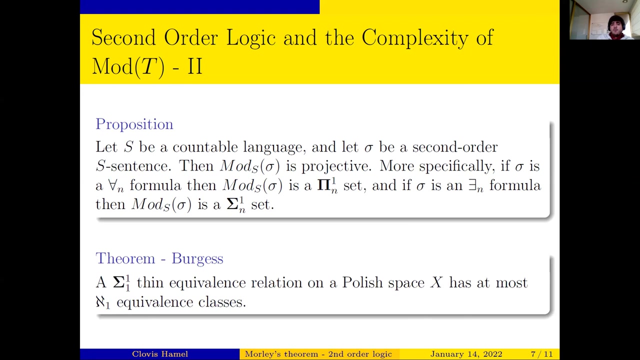 Roozbeh Gharakhloo And said so again. they prove here is induction, the complexity of the formulas, and the only interesting case that's not the same as what happens in first order is the existential second order, Roozbeh Gharakhloo, quantifier, and that's simply taking continuous images once again. that's why you came into the territory of projective sets. so we've been discussing about, we've been discussing equivalence relations. 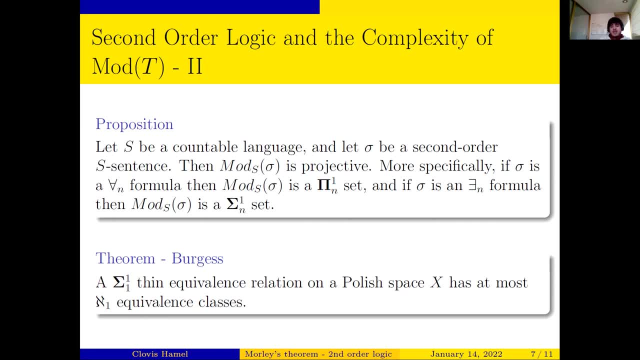 Roozbeh Gharakhloo And the projective sets- and this brings us this to your aim of burgess, which says that a Sigma, one, one thing equal is this relation and a Polish, a space X, Roozbeh Gharakhloo Has it most of one equivalence classes so more sophisticated, although the ideas were already there in the original paper, by morally, 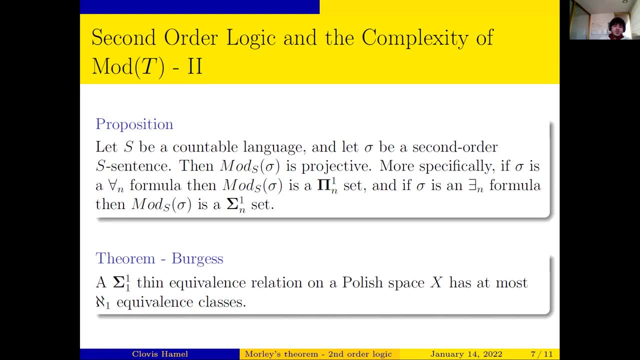 Roozbeh Gharakhloo. More sophisticated proof of hysteria is simply an application of burgess theorem: Roozbeh Gharakhloo And Roozbeh Gharakhloo. Actually, that gives you a little bit more, which is well, if less than or equal to live one or perfectly many. that's, of course, in the context of first order. but, like with many things in descriptive theory, when you go above analytic, then you start. 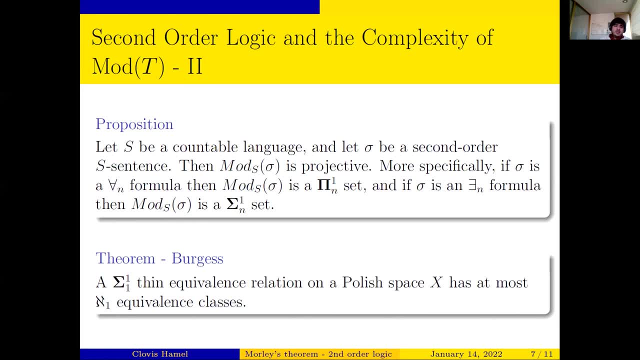 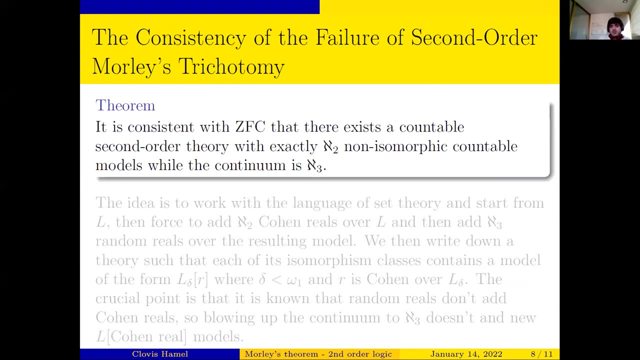 Roozbeh Gharakhloo Getting into independence result, and that's what we're going to be seeing in this case. for this more physical relation restricted to Roozbeh Gharakhloo, A given second Roozbeh Gharakhloo Order theory. so the consistency of the failure of second border of the circle door. there, more mystery, cotton me. 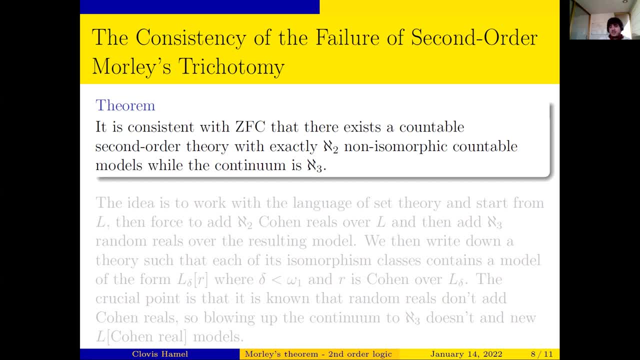 Roozbeh Gharakhloo goes as follow: it is consistent with set of see that there exists accountable second order theory with exactly Roozbeh Gharakhloo, All if two non isomorphic countable models, while the continuous I left three. so I have a sketch here, the idea of the proof, which is to work with the language of theory and start from l, then forced. 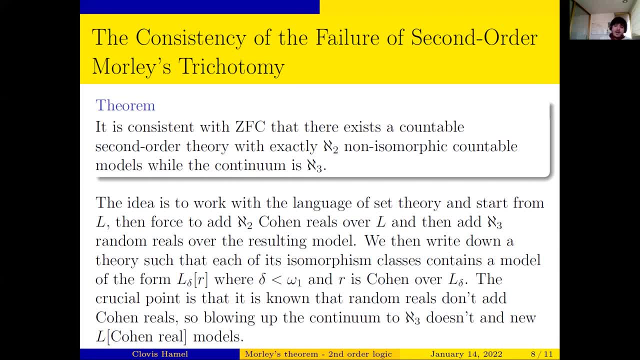 Roozbeh Gharakhloo. To add Roozbeh Gharakhloo, I left to go and reels over l and then I left three random reels over the resulting model. we didn't write down a theory, which is a little bit complicated. there are some long formulas there, but they're in the paper, if you. 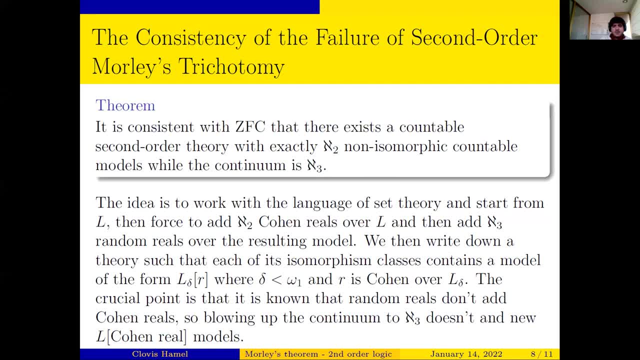 Roozbeh Gharakhloo are interested in reading about it. it's already an archive and that theory, such that the isomorphism classes Roozbeh Gharakhloo contain a model of the formula Roozbeh Gharakhloo are. 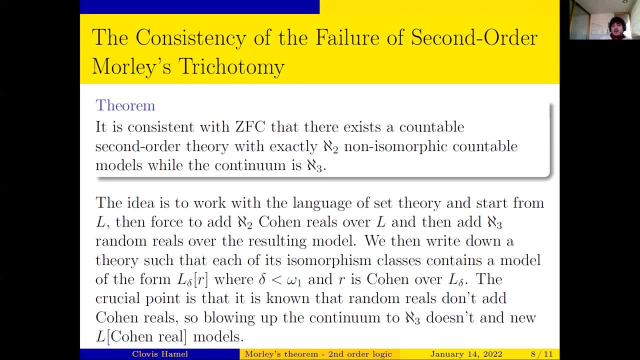 Roozbeh Gharakhloo, Where delta is less than one and our is that go henry all over l delta. and the crucial point in this proof is that it is known that Roozbeh Gharakhloo random reels don't add code and real, so blowing up the continuum to a left tree. 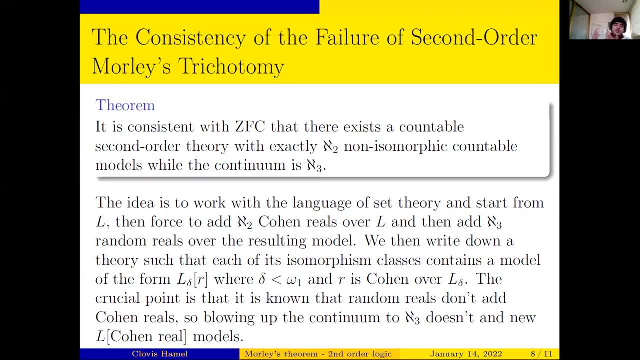 Roozbeh Gharakhloo doesn't add new models of the form l of a code real or l delta of a code real, which are the ones that we are using to count each of the equivalence classes. now, Roozbeh Gharakhloo For the. 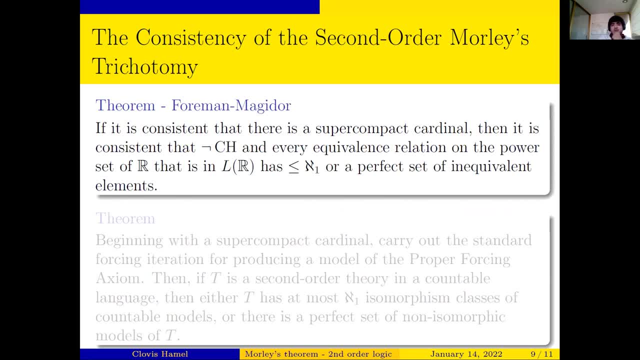 Roozbeh Gharakhloo. Consistency of the second order, more or less straight call to me. I want to start with the form, a magnet or a theorem which says, Roozbeh Gharakhloo, That if it is consistent that there is a super compact cardinal, then it is consistent that, see, it fails and every equivalence relation on the power set of our, that is in l of our, has less than or equal to live, one equivalent in equivalent elements or a perfect set of in equivalent elements. so our 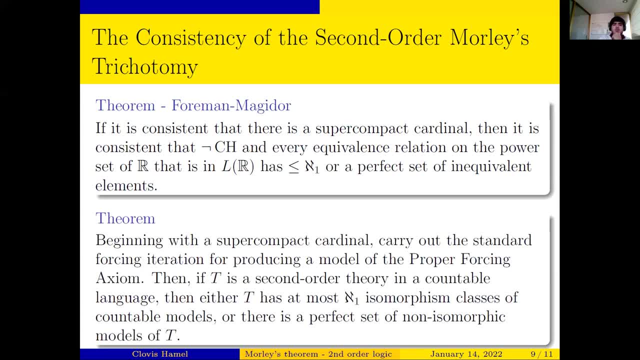 Roozbeh Gharakhloo. result follows: Roozbeh Gharakhloo From Roozbeh Gharakhloo From the yes of form and Maggie were, and you start with a super compact cardinal and you carry out the standard forcing iteration for producing a model of PFA. 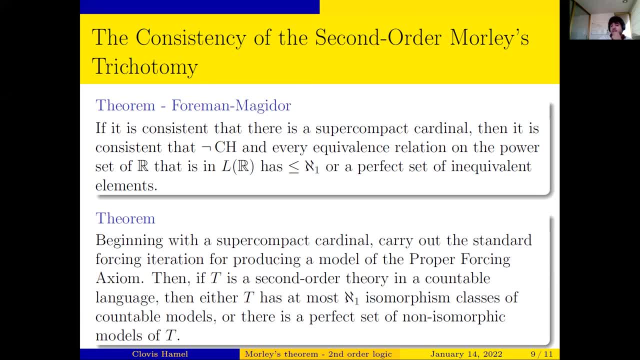 Roozbeh Gharakhloo, Then if he is a second order theory in a kind of language, then it either has, at most of the one is, amorphous classes of kind of models, or there is a perfect set of new and isomorphic models of the. the ideas here are that: 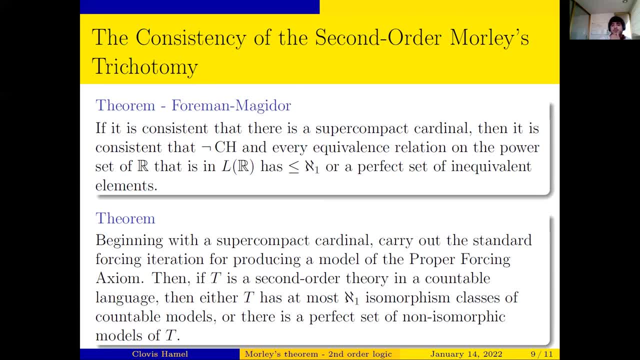 Roozbeh Gharakhloo. When you start with the sense that are the final Roozbeh Gharakhloo From the real, the real itself in smaller and super compact, then you can see that it remains. it appears at the, at the initial stage of the iteration, and ch happens cofinally, many cofinally often. so you can assume 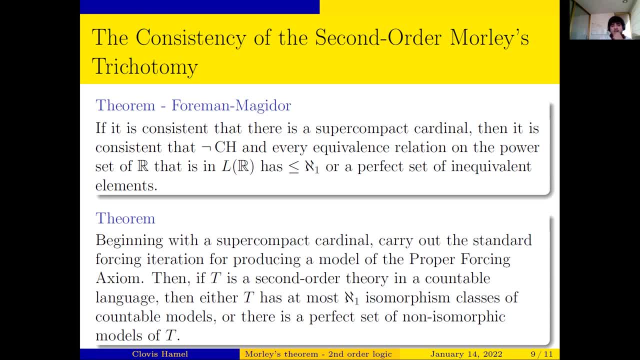 Roozbeh Gharakhloo, That ch holes at that stage without a loss of generality, and therefore you have, at most I live. one is amorphous in classes and by absoluteness, you, if it was Roozbeh Gharakhloo, seen it. 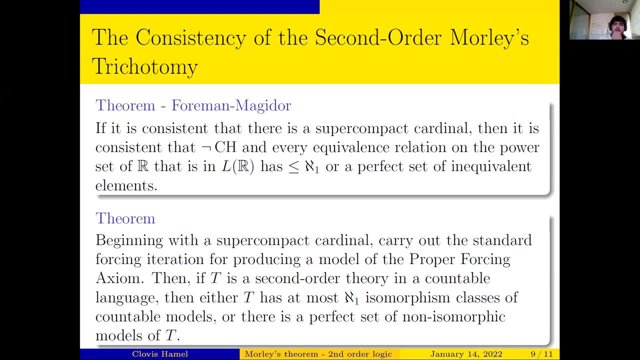 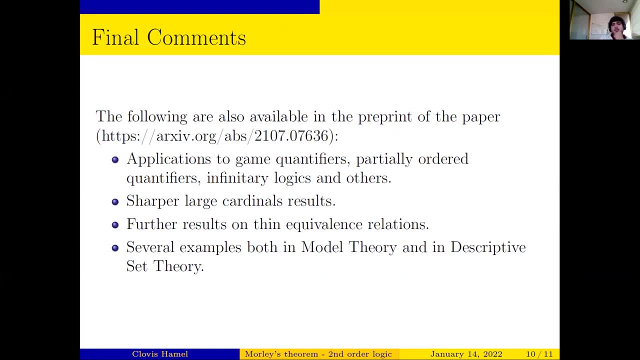 Roozbeh Gharakhloo remains 10. So those are the ideas behind this one, and then what I was mentioning before is that in the paper there are a few more things. it's the paper is Roozbeh Gharakhloo- Much longer than what I can cover in a 20 minute talk, but there are applications to gain quantifiers, to partially order quantifiers to infinity logics and others. there are much sharper. 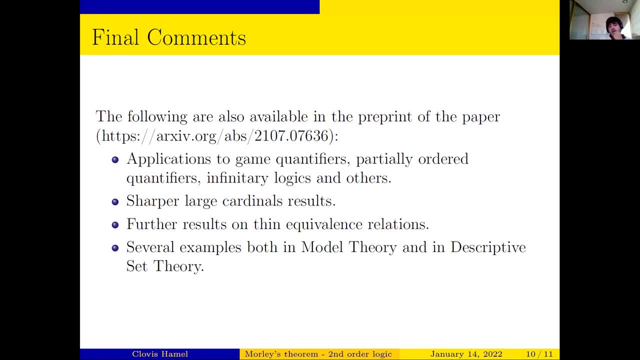 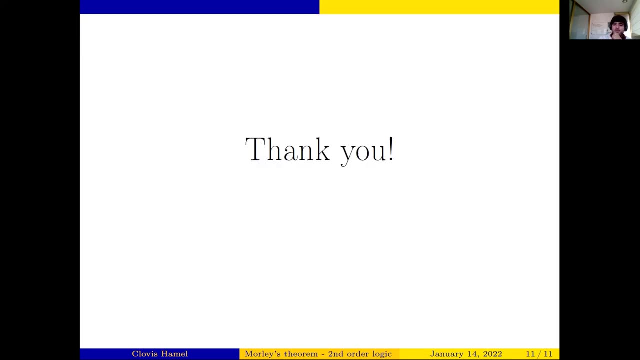 Roozbeh Gharakhloo And very interesting large cardinal results. you also have further results and thin equivalence relations, more on the descriptive set theoretic side and you also have several examples both in model theory and in descriptive set theory- Roozbeh Gharakhloo. So thank you very much. that is it for now. 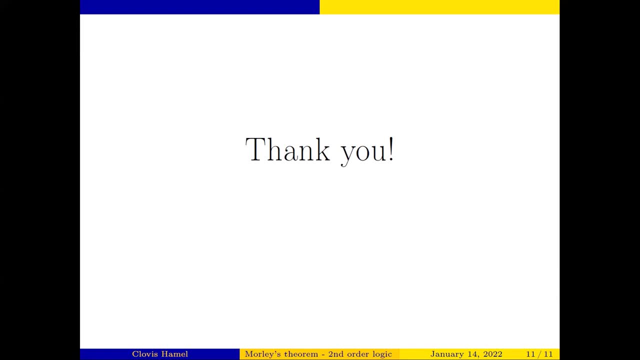 Christian Lebierello. Thank you, clovis, for the very nice talk um Christian Lebierello. Are there any questions? Roozbeh Gharakhloo? yeah, hi, clovis, I I do have a question. so, Roozbeh Gharakhloo, So I mean in this example that you made with the coin reals and the 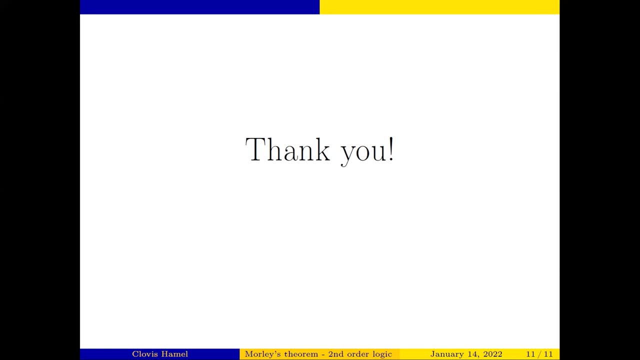 Roozbeh Gharakhloo And the random reals. Roozbeh Gharakhloo. How complex is the? is like the theory Christian Lebierello: Complete. oh yeah, it's a delta one two. Roozbeh Gharakhloo, delta one two. yeah, okay, so like the theory of each else. 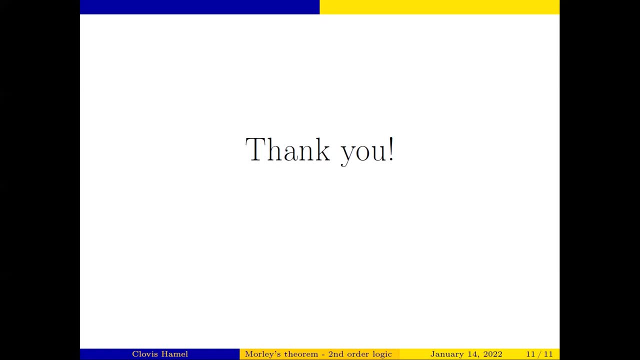 Roozbeh Gharakhloo. delta R is a delta one two. Christian Lebierello. No, it's a theory that we can that not fear of them. that theory, in which extra equivalence class you have a model which is of that form, is what's built. I want to that. the theory itself is rather complicated. it has some very long formulas, but we we're we have a very careful computation of the complexity of it. 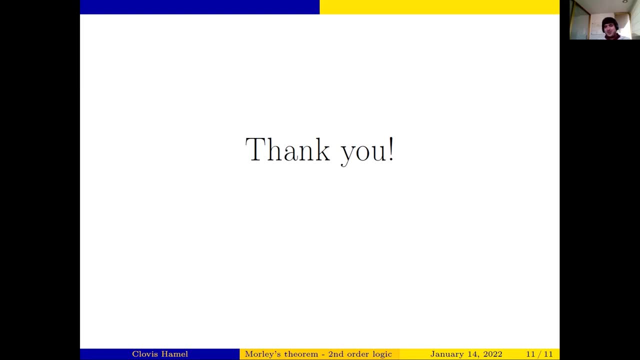 Christian Lebierello In the paper Roozbeh Gharakhloo, And I think it will be just another 20 minute talk to show the the theory and compute the complexity and do the details. but yeah, it's a delta one, two. 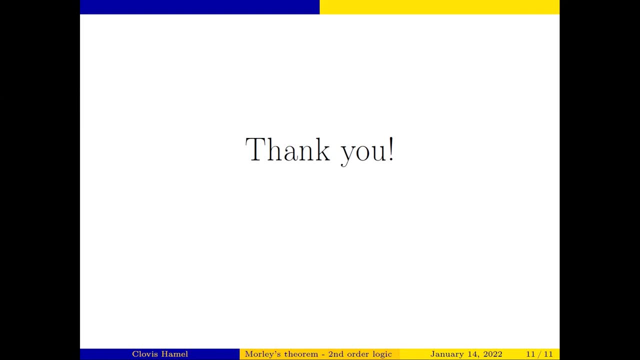 Christian Lebierello. So so, just to like re, so like the theory is probably just like Omega projective or something like that. but you're able to, Christian Lebierello, Like bring it down to the complexity of the collection of all the models. 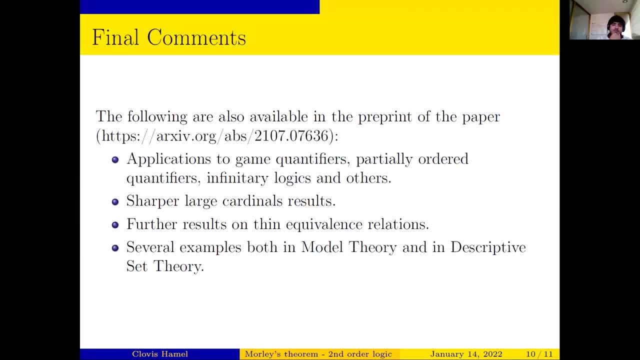 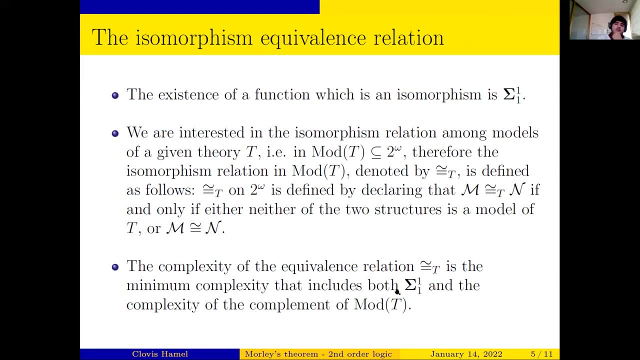 Roozbeh Gharakhloo. What? what i'm talking about is the complexity of the isomorphism relation. remember, that's the end. what matters is this one that's in this slide that one is still don't want to. Christian Lebierello. Okay, yeah, thanks. 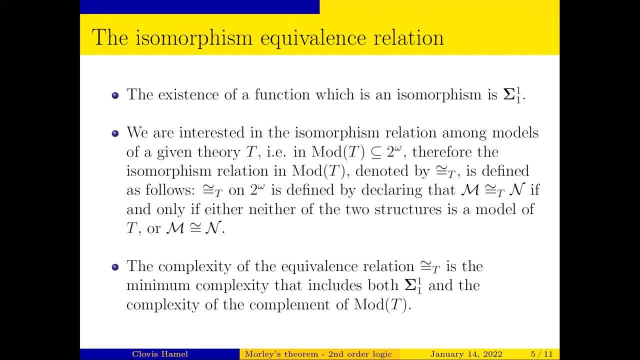 Roozbeh Gharakhloo. you're welcome, Christian Lebierello. I also have a question, Roozbeh Gharakhloo. Yes, um, so does PFA imply the trichotomy, the proper forcing axiom? Roozbeh Gharakhloo, Because, because you said it holds in the standard model. 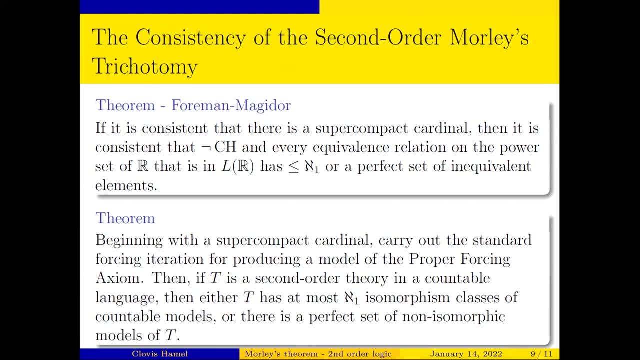 Roozbeh Gharakhloo For the proper forcing axiom: Roozbeh Gharakhloo, But you didn't say that the proper forcing axiom implies it Roozbeh Gharakhloo, One ready, Christian Lebierello. Sorry, can you repeat? David, it got out. 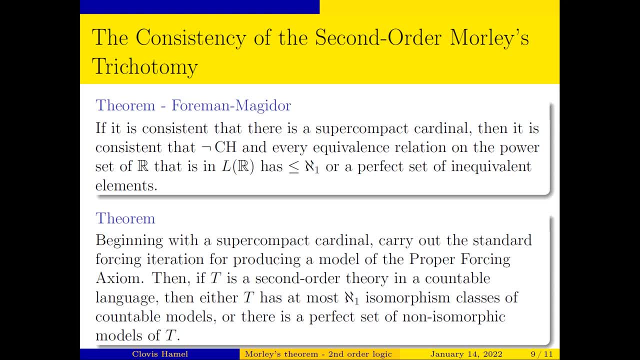 Roozbeh Gharakhloo. yeah, so your, your serum here. says that are your proof, says that in the standard model for the model that one usually builds for the proper forcing axiom, Roozbeh Gharakhloo, The Christian Lebierello, The. 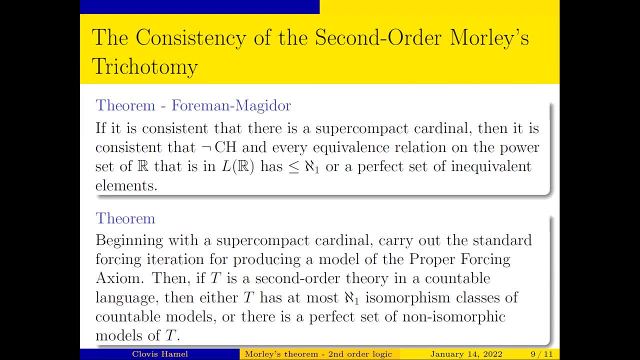 Roozbeh Gharakhloo, The trichotomy holes. but you didn't say that the proper forcing axiom implies more or less trichotomy. second order: more or less trichotomy, Roozbeh Gharakhloo. Okay, i'm. 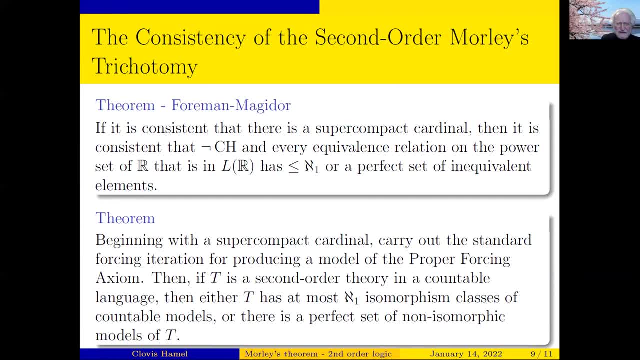 Roozbeh Gharakhloo, Interesting David Martin. um, maybe I can answer that, Roozbeh Gharakhloo. Yes, David Martin. yeah, this was. we use the model PFA because that was David Martin. It was convenient. 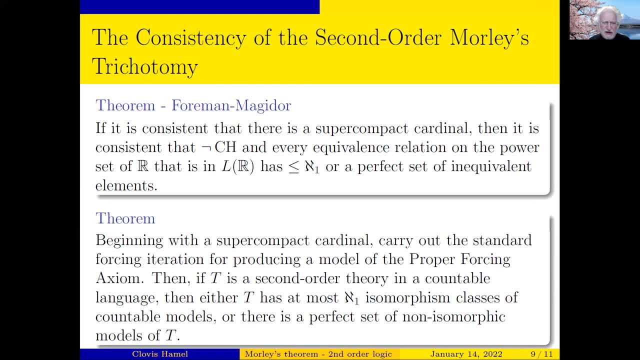 David Martin To David Martin. quote: form and maga doors theorem. David Martin, You can get much stronger David Martin results by looking at more carefully. and David Martin. So you don't in fact need a super compact, you basically need. 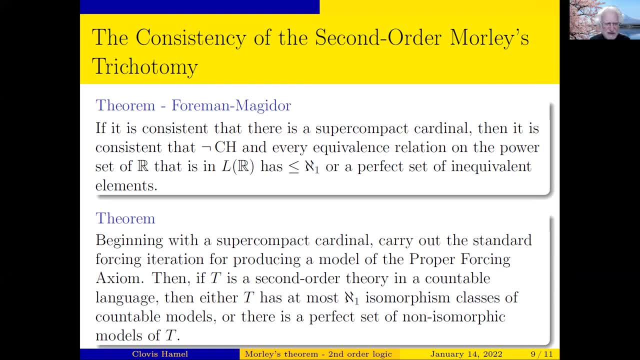 David Martin. Just a bunch of wooden cardinals to get this and David Martin, PFA implies David Martin. There are wooden cardinals, am I right? and so that would David Martin? Yes question: Roozbeh Gharakhloo. Right? no, it actually doesn't answer my question, although it's a very interesting answer because I asked if PFA outright implies it, so that I don't think this is really. I mean. so you're saying actually you could force it from much less. 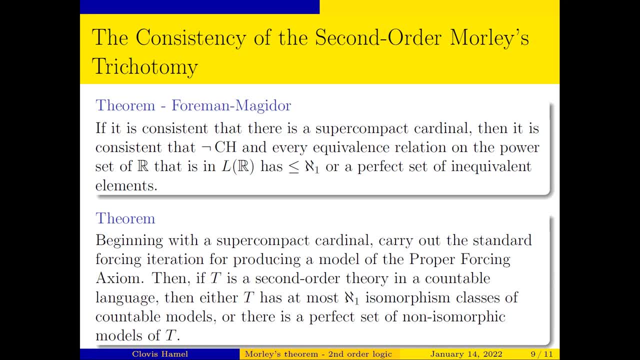 David Martin. Yes, Roozbeh Gharakhloo, You could force it directly, but that still doesn't tell you that just assuming PFA will imply Roozbeh Gharakhloo, That this Roozbeh Gharakhloo Second order trichotomy would hold. 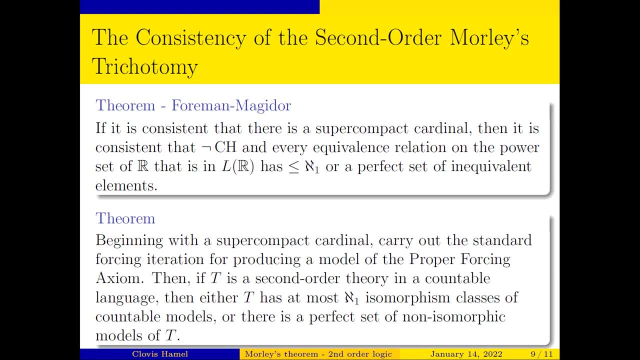 Roozbeh Gharakhloo Without going through forcing. just you know, apply, apply the proper forcing axiom and work in the round model. Roozbeh Gharakhloo. Probably, yeah, I don't know it. some, David Miller, It probably does, but i'll have to think about that. 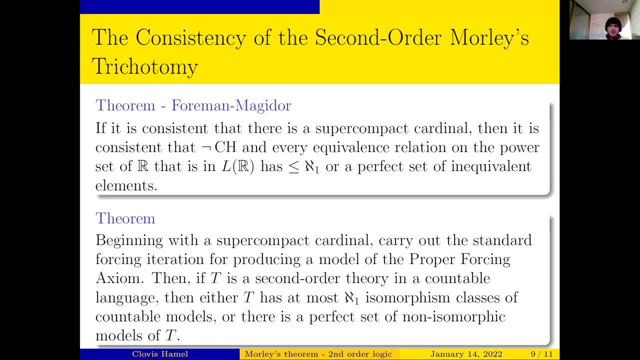 David Miller. yeah, I, David Miller, it's a Roozbeh Gharakhloo. it's a very good question, but we don't. I don't think we have an answer right and Roozbeh Gharakhloo, Whether PFA, as David is saying, straight up in place, that's right caught me. that's an interesting question you need. 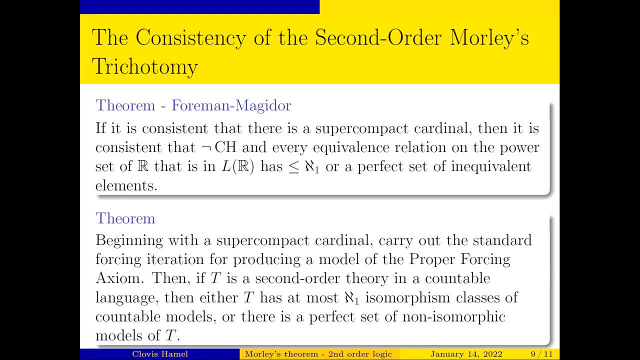 David Miller. cool, that's, i'm glad, David Miller. Alright, Okay, so thank you again, unless there are any further questions, any other questions where we should actually probably go on because of David Miller, Because we're running really late. so, um, let's see. Thank you again. the next speaker is Spencer under. 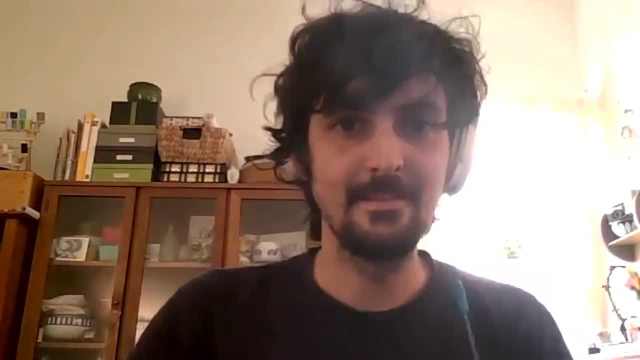 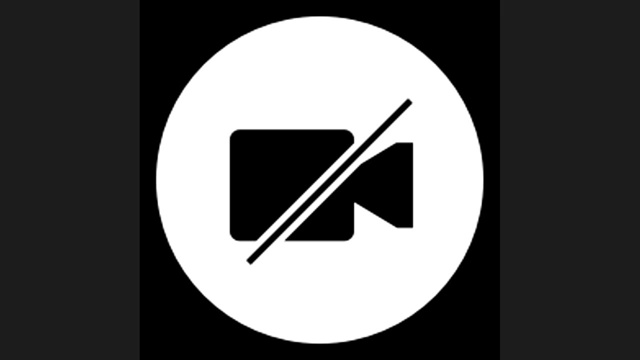 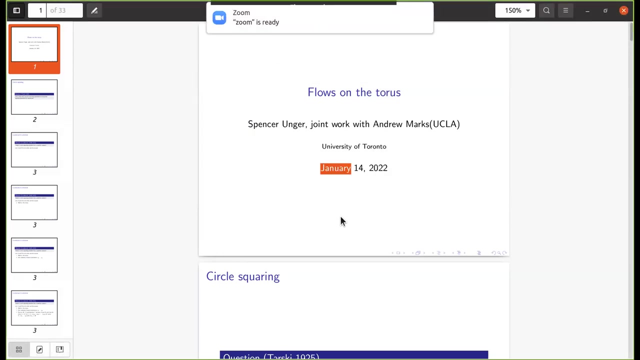 David Miller, Not mistaken. yeah, hi, cool hi, Spencer, um, David Miller, You share your screen please? yeah, one moment, David Miller. One Roozbeh Gharakhloo, I can see it. David Miller, Okay, great, let me make a big. 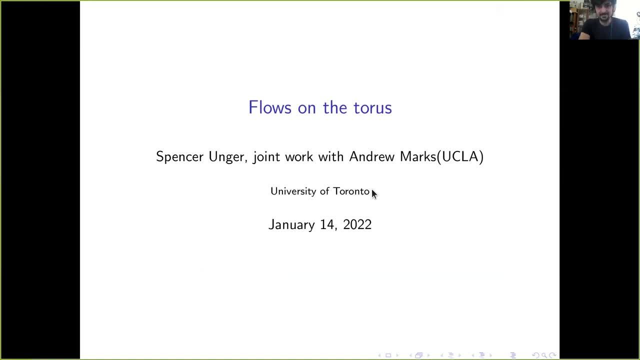 Roozbeh Gharakhloo. All right, so I guess i'll start. great thanks, um. so this is going to be a real change of pace from the previous talks. i'm going to talk about flows in the tourists, so let me explain. I guess I should also say, in order to do this, in 20 minutes, i'm going to not mention quite a lot of history and we're just going to go straight at the argument, which I think is understandable. 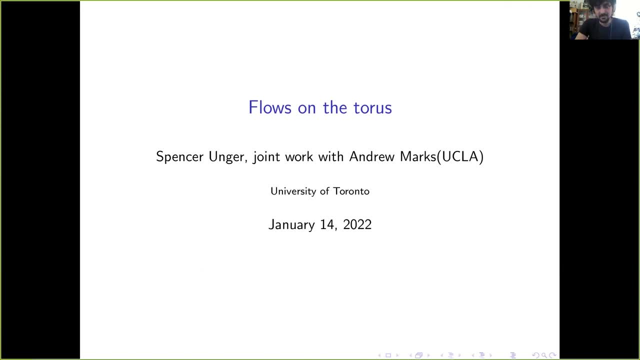 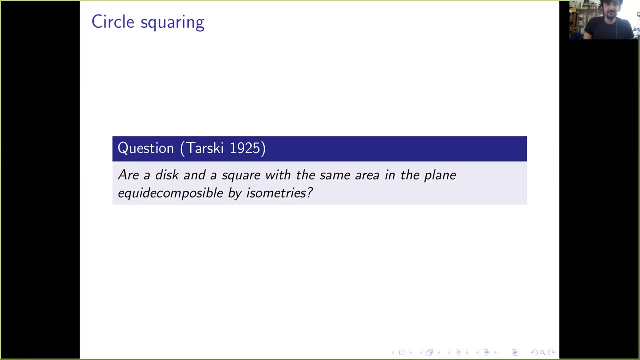 Roozbeh Gharakhloo. I think is understandable. Roozbeh Gharakhloo, Without a lot of background, Roozbeh Gharakhloo, And so there's a famous question of tarski, Roozbeh Gharakhloo, which asks whether a disk and a square with the same area in the plane, or equity composable by isometry. 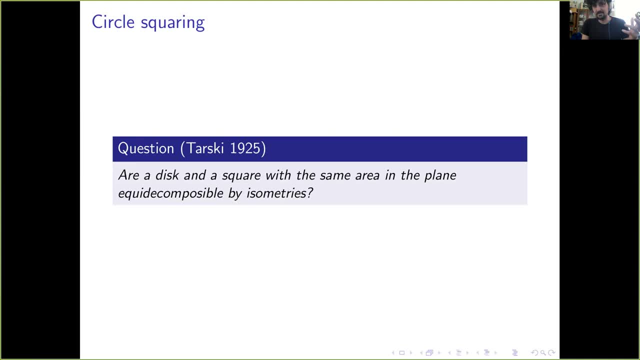 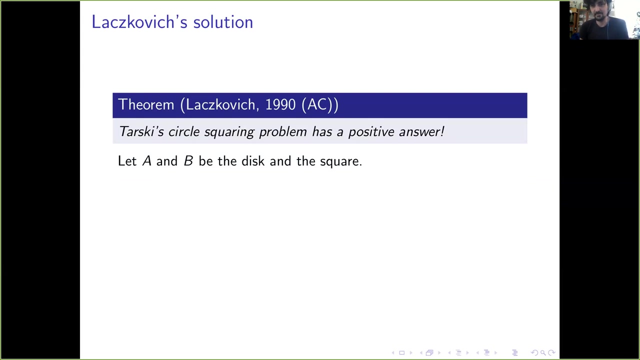 Roozbeh Gharakhloo. So what that means is you take the disk, for example, and you partition it into finitely many pieces and you move those by. isometry is different. isometry is to partition the square. Okay, Roozbeh Gharakhloo, And in the spirit of skipping quite a lot of history, this was solved positively by lascavitch in 1990. so it was open for a long time and that's going to choose the axiom of choice in his answer. i'm 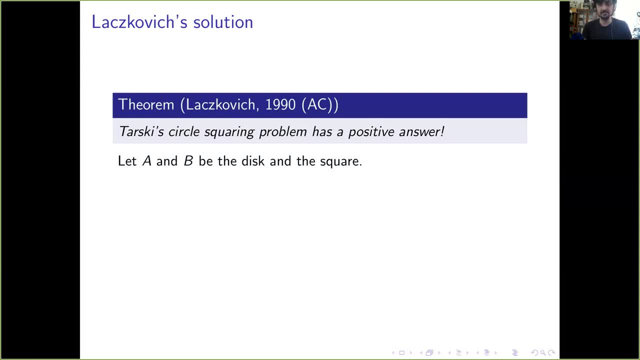 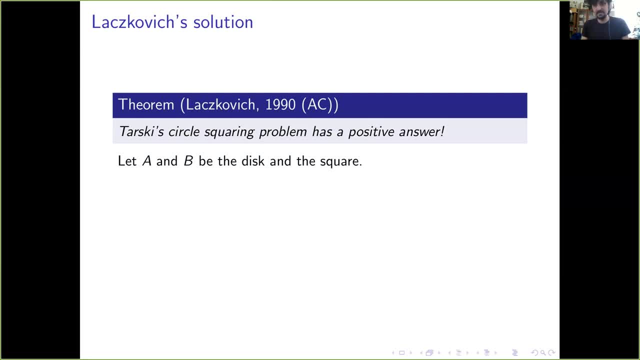 Roozbeh Gharakhloo. So, Roozbeh Gharakhloo, Tarski circle squaring problem. so this, this assumption that they have the same area, is necessary, Roozbeh Gharakhloo, But it was still open whether you could do this in any kind of constructible way. 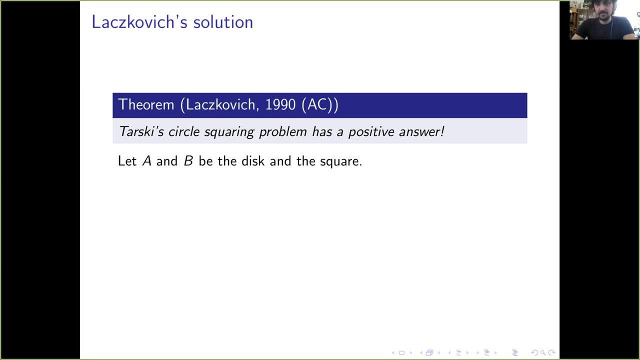 Roozbeh Gharakhloo. So just briefly, let me say what the the idea of the proof was. so you take a disk and a square A and B in the plane and the first thing you're going to do is you're going to change setting to the Taurus. 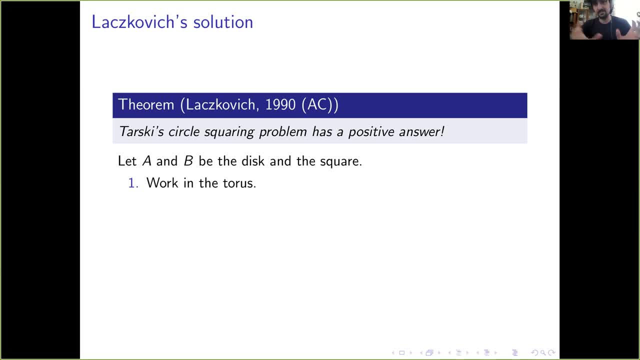 Roozbeh Gharakhloo. Okay so, Roozbeh Gharakhloo. So if you take this disk and square and you translate and scale them down to live in a Roozbeh Gharakhloo, A power of the interval. 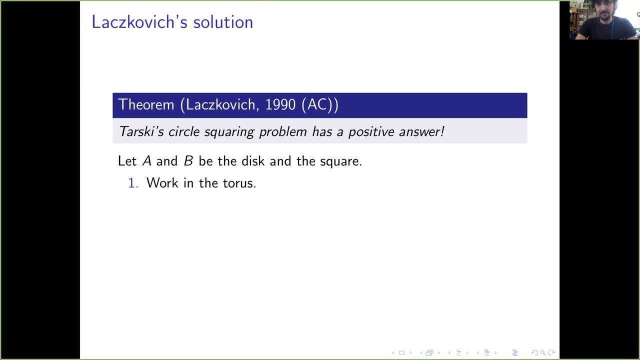 Roozbeh Gharakhloo, Inside the Taurus. Roozbeh Gharakhloo, Then you, this equity composition result is going to hold in the Taurus, if, and only if, it holds in Roozbeh Gharakhloo In the plane. okay, so we're taking our whole big space, are squared and we're just going to focus down on this, this little compact thing. so the action we're going to use is the action of 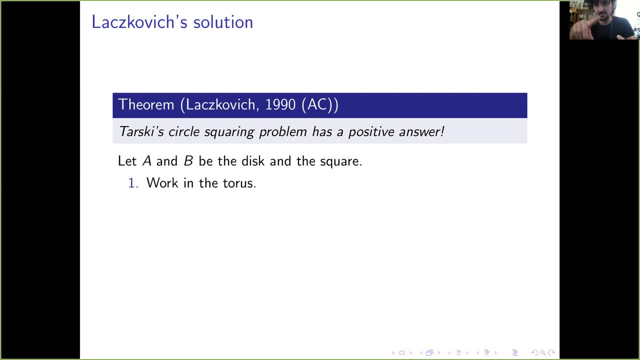 Roozbeh Gharakhloo. Translating: Roozbeh Gharakhloo. Translation on the Taurus. so this is the action and sort of addition, modular one: Roozbeh Gharakhloo. Okay, so another feature of the result is that, since we're working in this nice compact space, there's a probability measure and we can choose things randomly. so select things from some fixed measure, one set in the Taurus. 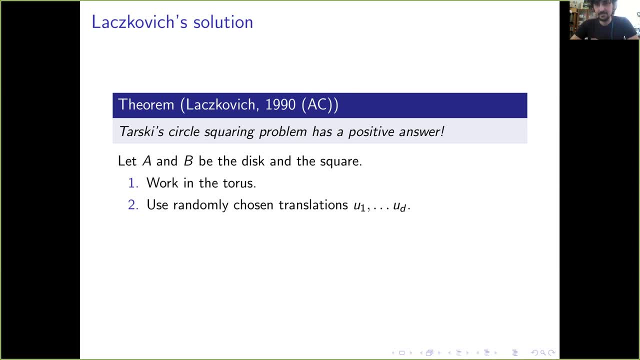 Roozbeh Gharakhloo. And so these translations, you one through you D, are going to give rise to an action of Z to the D: Roozbeh Gharakhloo On the Taurus. Roozbeh Gharakhloo. Okay, and then? 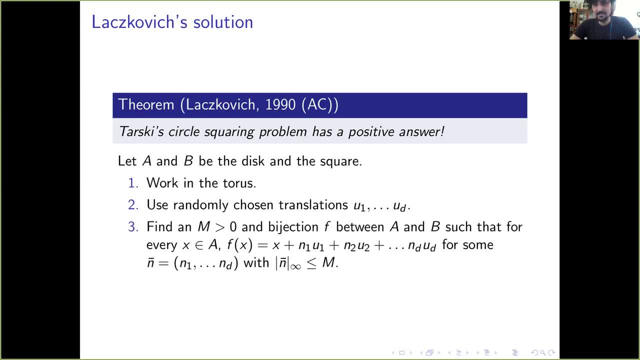 Roozbeh Gharakhloo. skipping, oh, so many details. Roozbeh Gharakhloo. This is the. this is third point is how you find the equity composition. so you find a, an M, which is some bound, and you find a bijection between A and B. 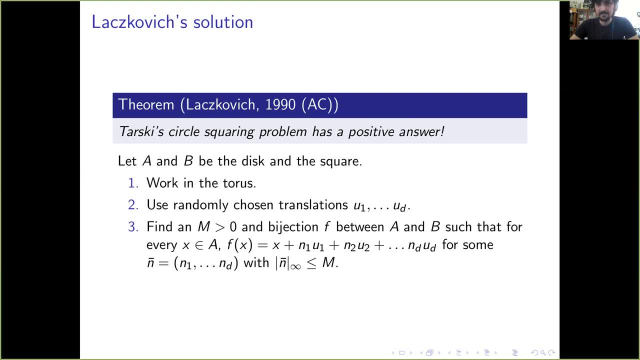 Roozbeh Gharakhloo, So that every for every X, F of X has this form that i've written down here. so it's just a shift of X by Roozbeh Gharakhloo, You know, and one times the first factor- you one, and then and two times the second vector, you to, etc. um, but the crucial point here is that you've- you've actually only allowed yourself finitely many possibilities for how you're going to shift each X. okay, so that's the point of bounding the soup norm of this. 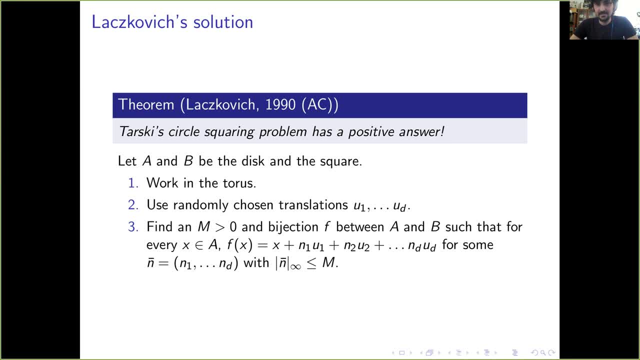 Roozbeh Gharakhloo Of this vector and bar by your bound capital, M. Roozbeh Gharakhloo. Okay, so, that's. that's. that's, Roozbeh Gharakhloo. Okay so, Roozbeh Gharakhloo, Okay so. 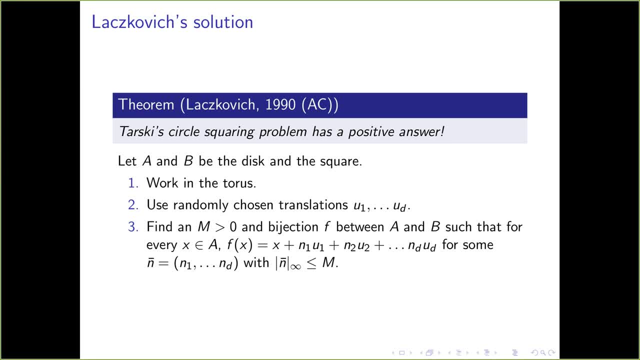 Roozbeh Gharakhloo. So these are natural numbers: Roozbeh Gharakhloo. Correct integers, if you'd like, Roozbeh Gharakhloo. um, yeah, in it we should call them integers that'll. that'll make it nicer. 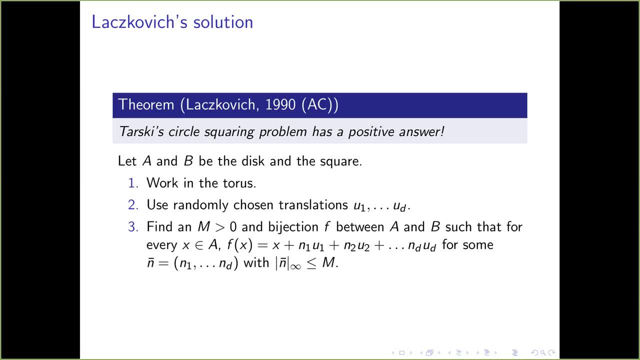 Roozbeh Gharakhloo. Oh right, um, Roozbeh Gharakhloo. Okay, so, using this bijection, what is the equity composition? Roozbeh Gharakhloo. The equity composition is: the pieces correspond to these end bars. okay, 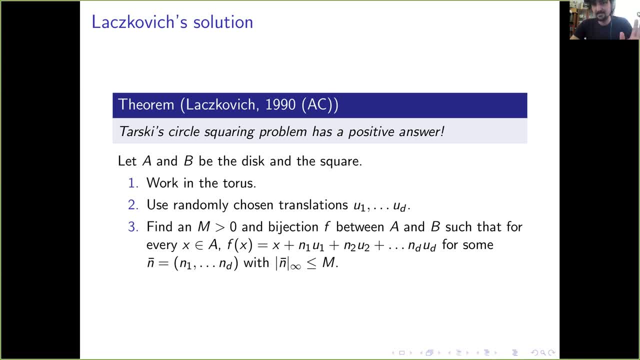 Roozbeh Gharakhloo. So there's a, there's a piece we will call a end bar, which is just the set of the set of X, where F acts like Roozbeh Gharakhloo, Shifting using this end bar. okay, and that's a partition of a, and then the isometry is: are exactly applying this. 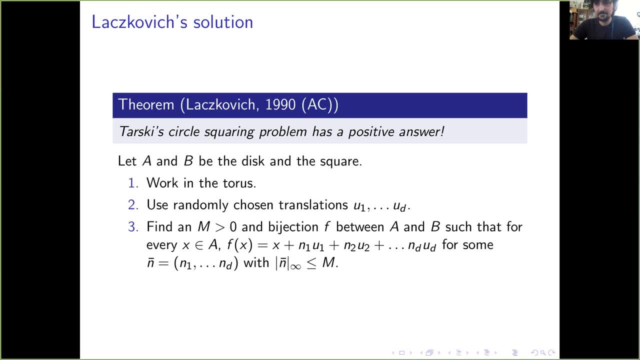 Roozbeh Gharakhloo. Appropriate vector of translations: Roozbeh Gharakhloo, Corresponding to end bar: Roozbeh Gharakhloo. Okay, so this is. this is some kind of extremely rough outline of the proof. so 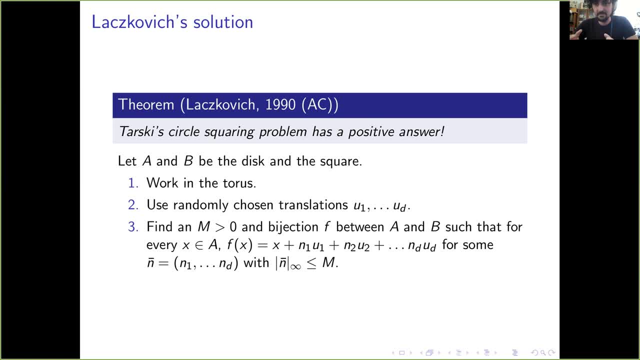 Roozbeh Gharakhloo. The disk and the square are going to be equity composable by translations, Roozbeh Gharakhloo. we're going to find those translations by working in the tourists and choosing some random ones, Roozbeh Gharakhloo. But then the translations we need, our are generated by the random ones. okay, under this action of Z to the D, 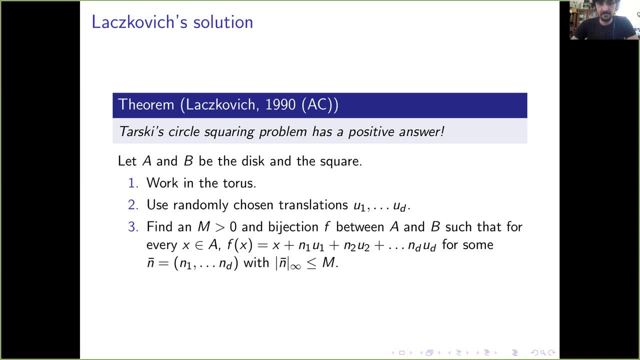 Roozbeh Gharakhloo, Alright. so what I want to talk about is: is this one aspect of this circle squaring thing? Roozbeh Gharakhloo, Okay, Roozbeh Gharakhloo, Okay. before, maybe a little bit more history. so 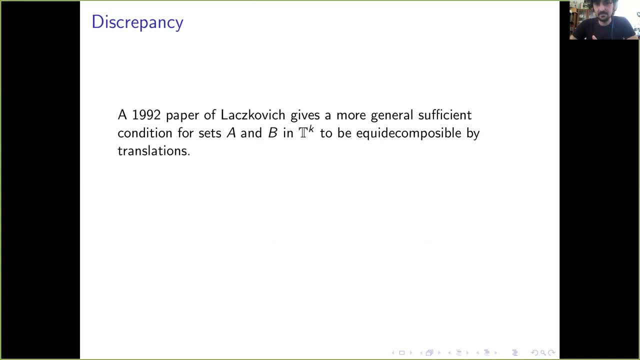 Roozbeh Gharakhloo In a 1992 paper, laska, which gives them much more general, sufficient condition for equity composability by translations. Roozbeh Gharakhloo, It turns out the important condition on A and B is that they have 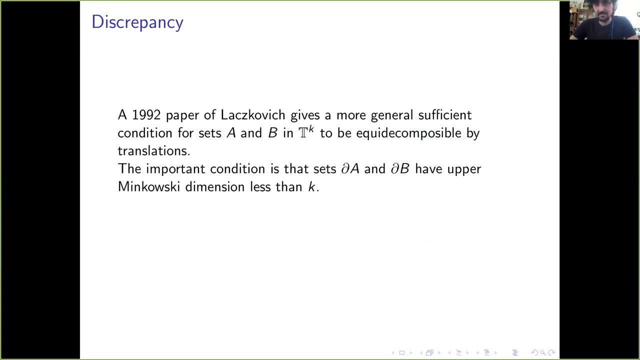 Roozbeh Gharakhloo. Their boundaries, sorry, have upper minkowski dimension less than K Roozbeh Gharakhloo, And for the purpose of this talk it's not going to be important what the definition of upper minkowski dimension is. 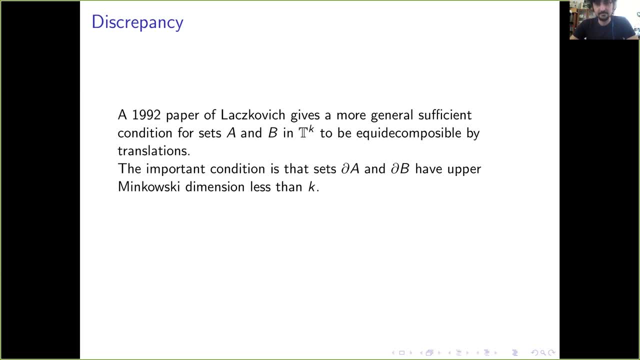 Roozbeh Gharakhloo. it's also sometimes called box dimension. it has something to do with covering the boundaries of A and B by boxes- Roozbeh Gharakhloo, of smaller and smaller side length, and watching what happens to the number of boxes that you need. 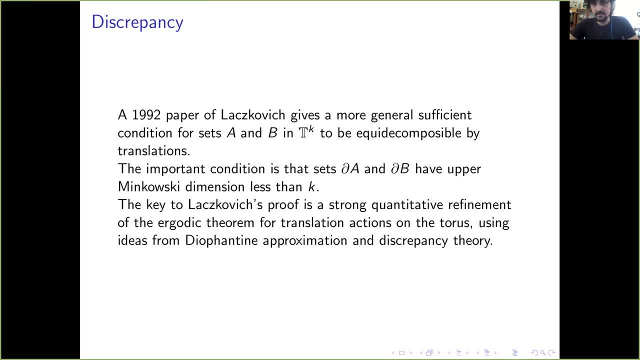 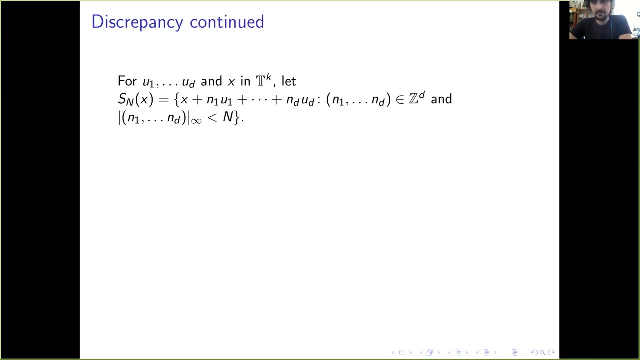 Roozbeh Gharakhloo, Something like this. Okay, and the key to Alaska, which is proof, is some kind of quantitative refinement of their God theorem for these actions of of translations, Roozbeh Gharakhloo, And I think it's very interesting to see this kind of. 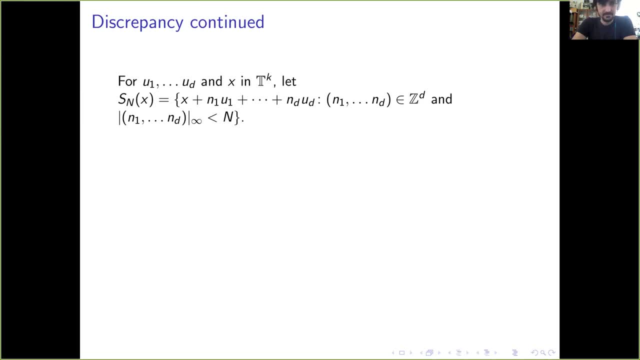 Roozbeh Gharakhloo. And I'll say more specifically what this. Roozbeh Gharakhloo, The so called discrepancy estimates. Roozbeh Gharakhloo. Okay, so we'll do that now. actually, I'm going to define a set Sn of x. This is just all of the things that you can get to by. 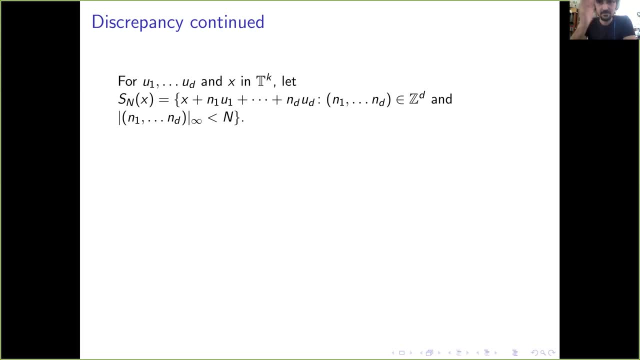 shifting by what I want to say. you know, n1 times u1 and n2 times u2, etc. okay, but under this bound on the soup norm. So this is just a finite subset of the torus. and here I guess actually I want these n1 through nds to be natural numbers. 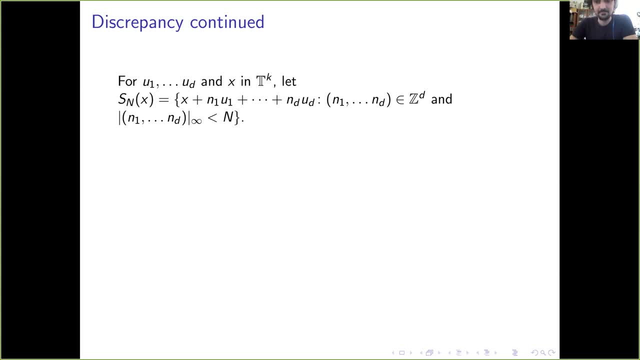 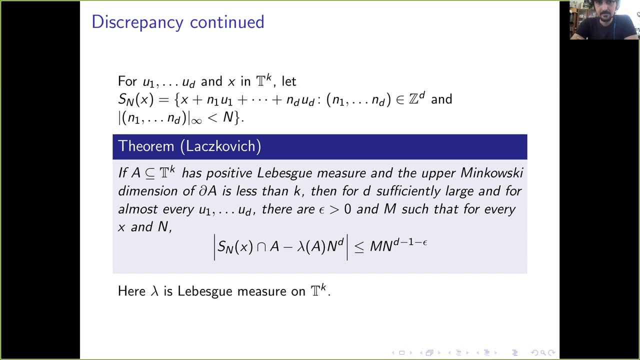 That's a typo. okay, so that's not a big deal for the statement of this theorem. So the size of this set, Sn of x, should be capital N to the d. Okay, so what are these descriptions? So, for the frequency estimates, suppose that A is just a subset of a torus. 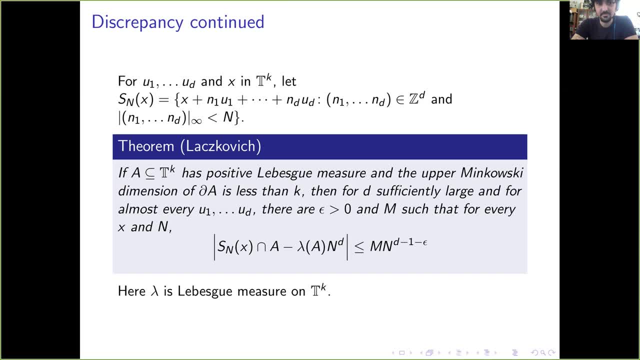 It has positive Lebesgue measure and it satisfies this condition that the upper Minkowski dimension of its boundary is less than k. Then if I take d large enough, so that just means I'm going to take enough randomly chosen translations, then for almost every u1 through ud I have this inequality. 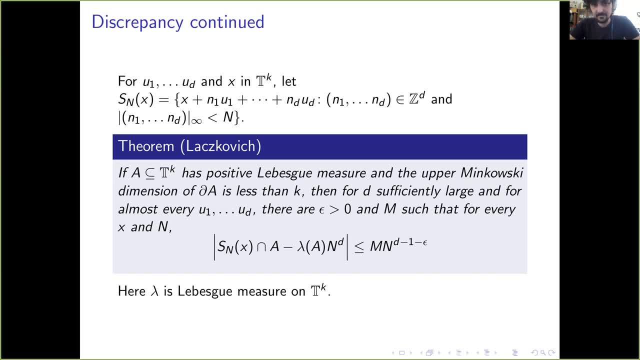 down here, So let's just focus on the left-hand side of the inequality. What is this saying? I'm looking at this set Sn of x, which is like some kind of square, If you view the action of these translations as giving you a lattice inside the torus. 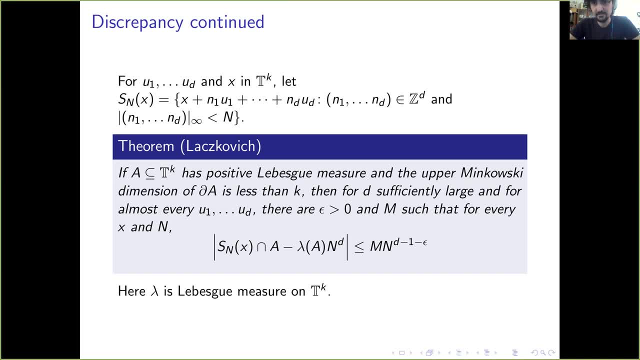 then this Sn of x is like a square subset of that lattice with a. Thank you, the base point at x. okay, and so I'm asking: how many points of a do I see inside this finite square and the? the inequality is telling me roughly. I see the. 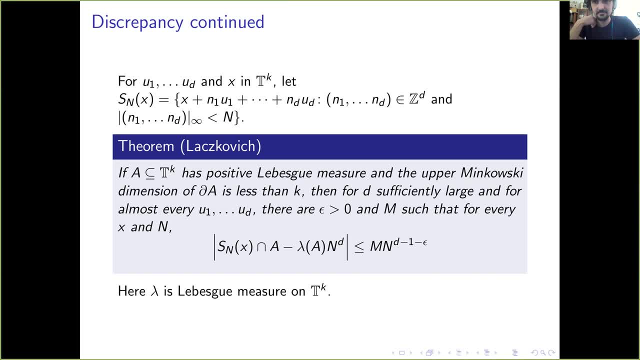 the Lebesgue measure of a times the number of points in the square. okay, so this is a an important point and we'll pause here for a second to make sure that this makes sense. so, um, there's some kind of action by translations inside this action you have. 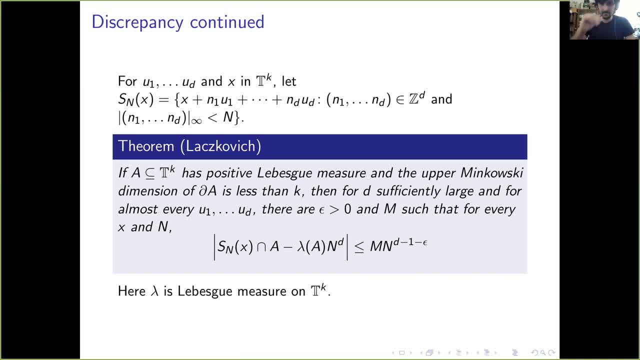 these very natural sets, which are squares, and this theorem is telling you that if you have one of these extremely nice sets, where its boundary is not too crazy, then inside each one of these squares, literally every square that you draw like this, you see roughly the number of points. 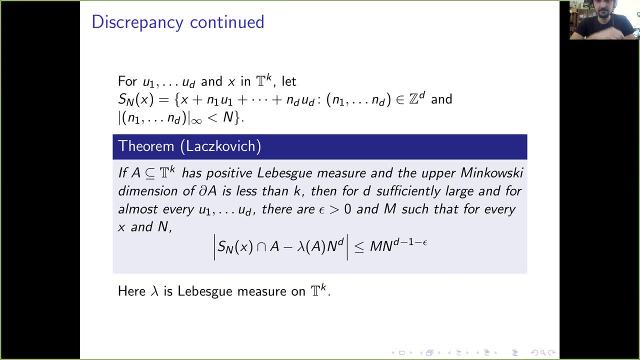 you expect, based on the Lebesgue measure of A. So sorry, Spencer, Maybe I'm reading something wrong, But isn't m times n to the d minus 1 minus epsilon like a really big number? Yes, OK, so this is a good point. 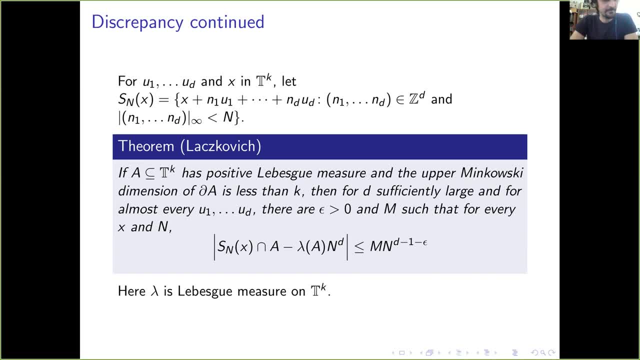 So the way I've written this, this is like a sort of un-normalized version. So the quantity that's going to be small or approach to 0 is, if you divide all of this through by capital, N to the d, Oh, OK, 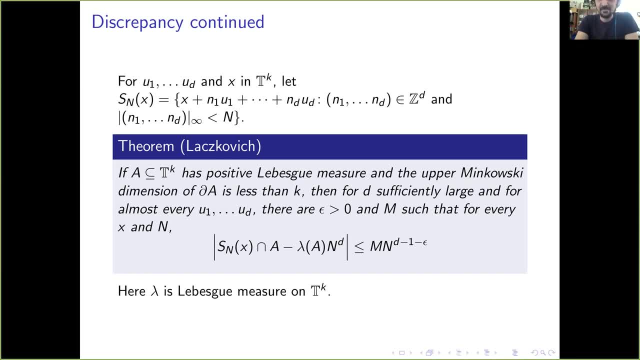 So in that case, what you're saying is the fraction of the points of A that you see inside the square is roughly the Lebesgue measure, And that estimate goes to 0 quite quickly. OK, Yeah, that's a very good point. 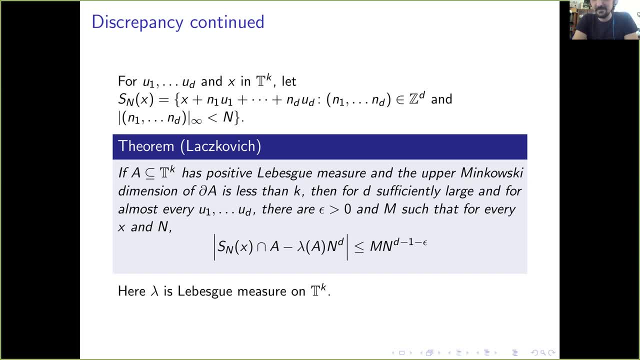 So whenever you write these discrepancy estimates, you have the choice of whether you normalize them by the number of points inside this square or not. So I agree that the normalized version is maybe a more intuitive thing to say here. Yeah, so the right. so if you're looking in terms, 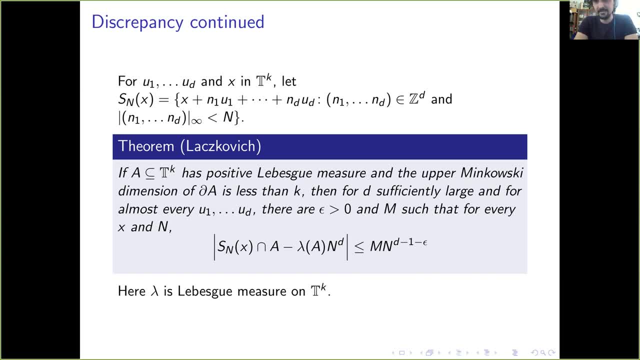 of an absolute number of points. you just end up with some error, But the error is bounded in some nice way. OK, but then if you divide by this capital N to the d, then you actually get two quantities that are converging to each other. 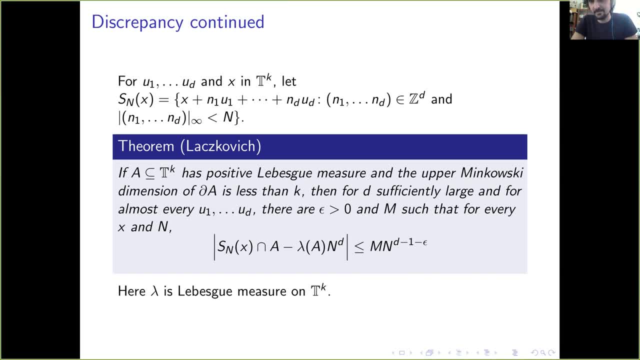 Why isn't it just enough to say that the number of points that are converging to each other is just the number of points, Yeah, Yeah. Why is it just enough to say that it goes to 0 as N over minus 2?? 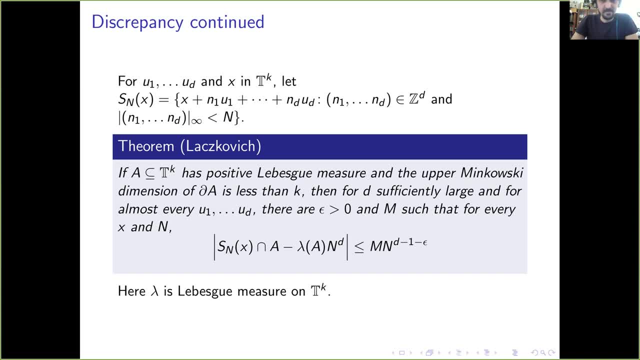 Let me think Probably, because in general it's not true. Ah oh, thank you. Oh, that's good. What about N over minus 1?? I mean 1 over N. Yeah, OK, good, This is a very good point. 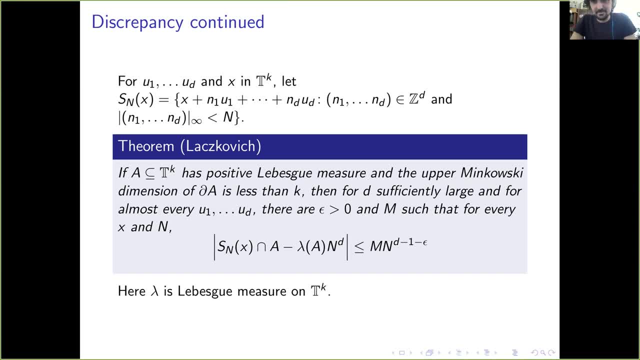 So the crucial thing: I really should have written the normalized version. If you normalize this, you get this N to the minus 1 minus epsilon. That N to the minus 1 minus epsilon is summable in N. Ah, OK, that's what you want. 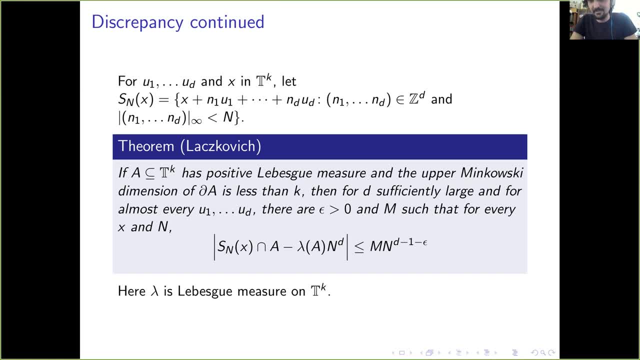 I see. So if you erase the epsilon, then you no longer get something that's summable And that actually reduces the power of your theorem. Right, thanks, Yeah, so that's another extremely good point. OK, OK, The summability. 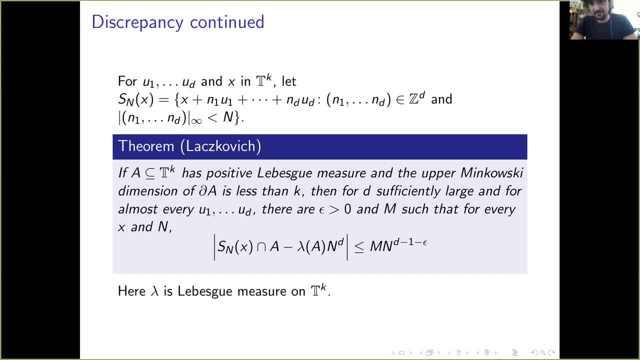 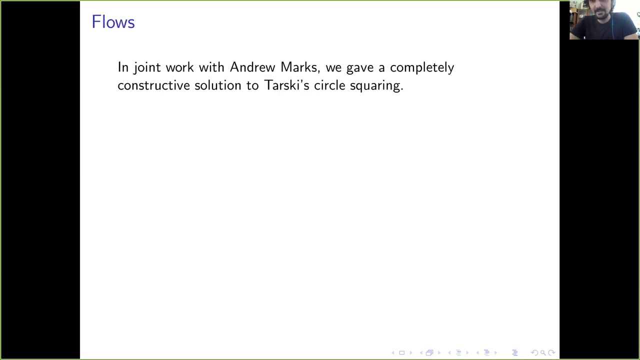 The summability of this term on the right-hand side, once you've divided, is a crucial piece of the argument. OK, so this is the discrepancy theorem that we need. What am I going to say next? OK, yeah, so Andrew and I gave this constructive solution. 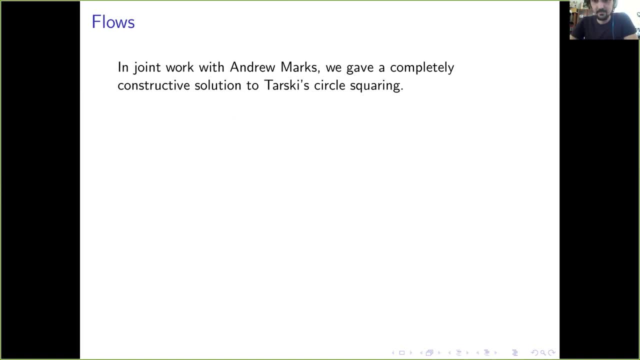 to the circle-squaring problem, And one of the key features of that that I want to talk about is the notion of a flow. OK, And the flow acts as a kind of continuous analog of an equity composition. So this was the reason that it was kind of crucial. 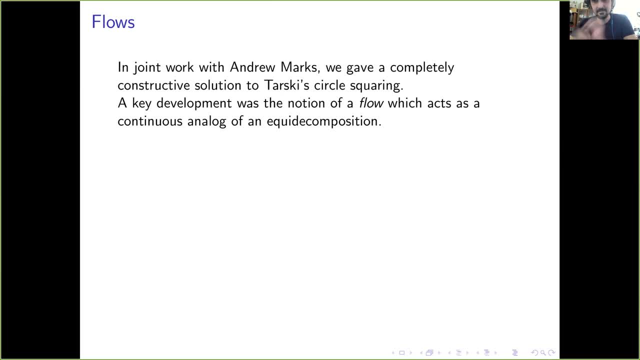 And the proof is that, instead of just trying to construct an equity composition from scratch, we first constructed this continuous analog, And then we somehow fixed the continuous analog to be a real one. OK, so let me tell you just briefly what a flow is. 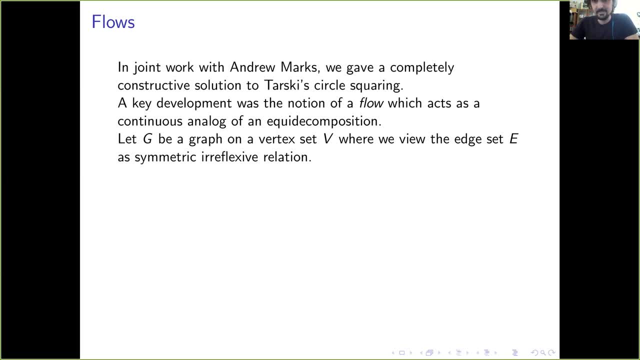 So let's take a graph g That's on a vertex set v, And we're going to view the edge set as symmetric and irreflexive relation. OK, so it's really a directed graph, but the relation you get is symmetric. 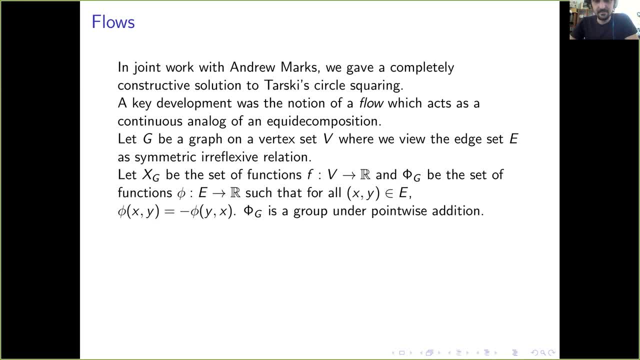 OK, That's convenient for us. OK, Ok, to define two collections. So xg is going to be the set of real valued functions on the vertices and this capital phi g is going to be the set of real valued functions on the edges. 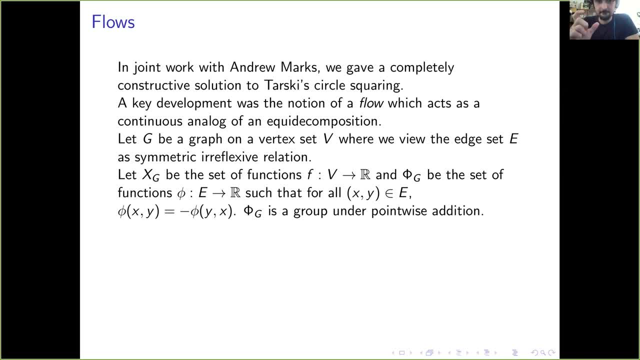 with this additional property that the phi along some edge is negative phi along the reverse edge. Okay, and we'll see why we have this restriction in just a second. Both of these sets are groups under pointwise addition. It's just a kind of natural comment. 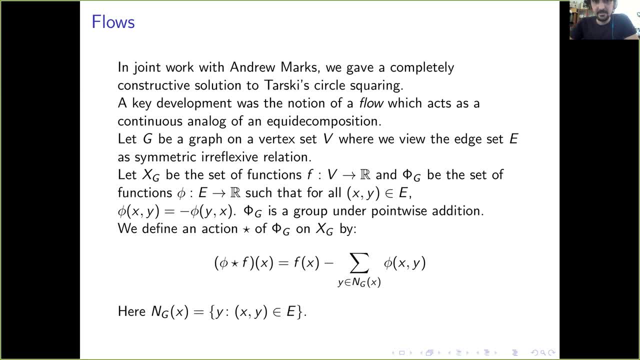 So we're going to define an action of phi g on xg by this formula here. Okay, so maybe instead of reading the formula, I can try to tell you what the action is doing. So we're thinking of the function f of xg. 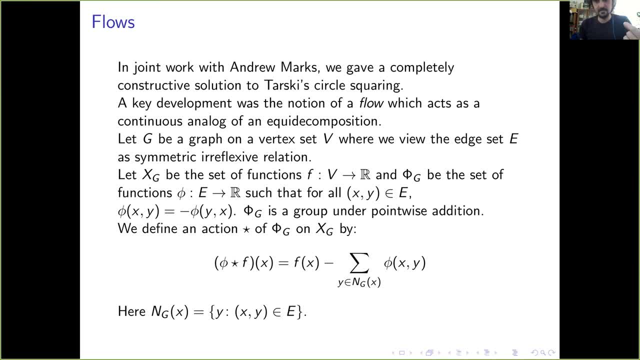 So the function f is assigning a mass to every vertex and then the function phi is going to tell us how to move mass around. Okay, and the condition that if I move mass along an edge 5xy, mass along the edge xy, that should correspond to moving like negative mass in the other direction. 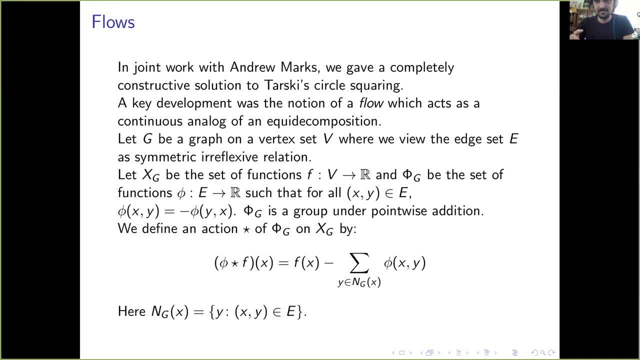 That's why we have this kind of anti-symmetry condition. Okay, and so this, this action of phi on f. this is exactly the function that you get after you move the mass of f according to phi. Okay, so the new value at x is just the old value f of x. 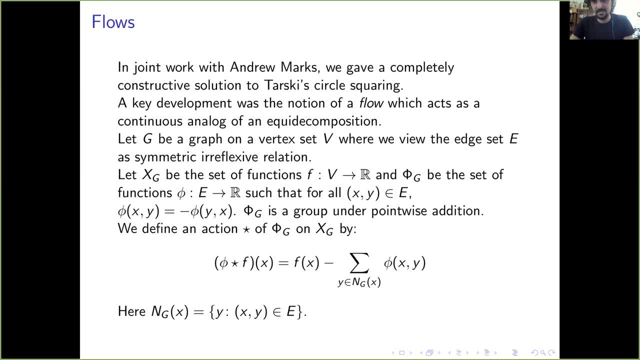 minus all of the contributions of moving the mass, according to phi. Okay, so this is actually not how we phrased it in the original circle squaring paper, but this is a kind of nice way of thinking about what's going on in the background. 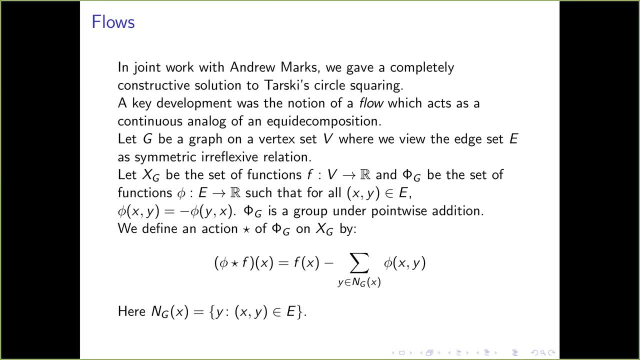 So you have some sort of mass distribution which is stable under starring weight, Storing with phi or what. So I'll explain, maybe in a slide or two, how this is going to be related to this segue decomposition problem. Okay, So just the thing to think of is we have a function which represents sort of putting 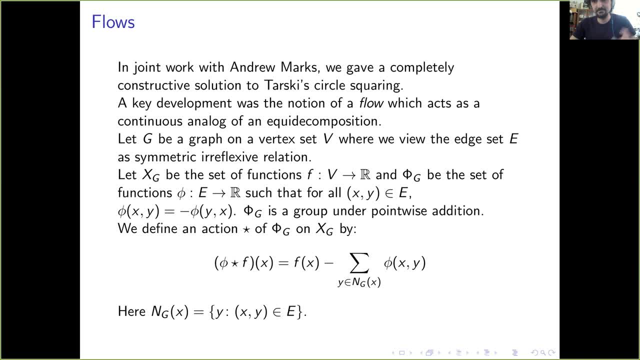 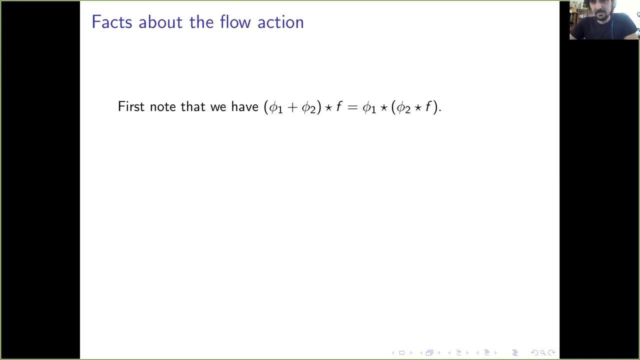 a mass at every vertex and we have these possibly different flows, phi, that are moving the mass around in some way, And this action tells us us how to move the mass according to phi. So this action has a number of kind of weird properties. 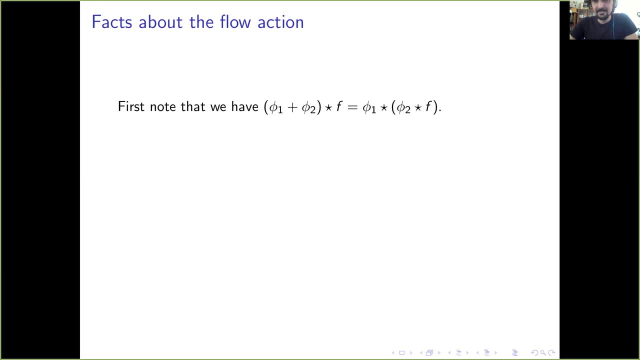 So this is the first one. If you think about the definition of the action, you'll see that this is true. So the point in this definition of the flow action is that there's like a conservation of mass going on. The mass of f just gets redistributed by phi. So there's this weird phenomenon that acting by the sum of phi1 and phi2 is like acting by phi2 and then acting by phi1.. 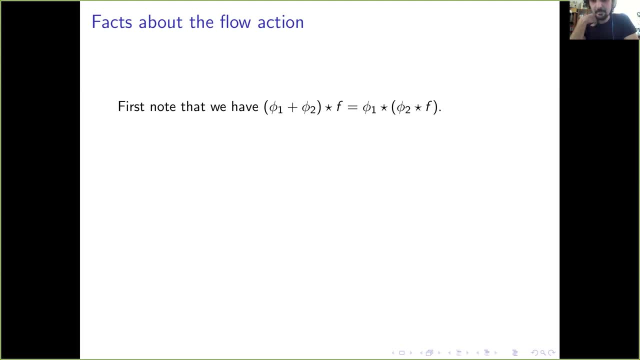 Okay, Maybe even weirder, is a relatively easy lemma that we won't prove, but I wanted to state for you: is that actually, if I have some sums of both functions and flows that are both absolutely convergent, then I can interchange the limit and the sum? 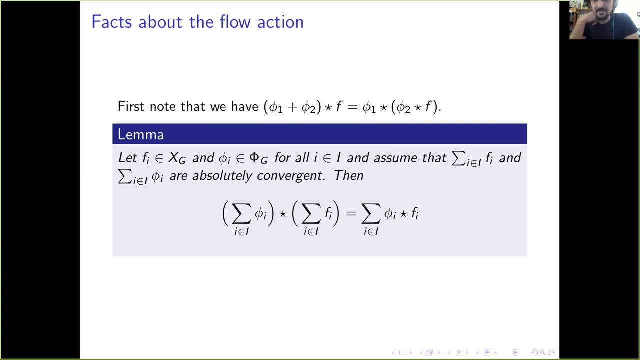 I'm sorry, the star and the sum in a way that you might think is true. You might not expect. So again, this, this formula from the lemma, is reflecting a kind of conservation of mass that happens because of this star action. But the moral of the story is that all of the kind of like distributive 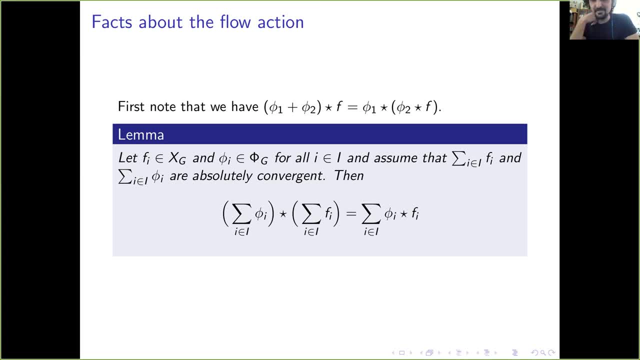 But the moral of the story is that all of the kind of like distributive laws that you might expect about this star action are not true. OK, so we're going to, kind of crucially, use this lemma in a quick sketch of the argument. 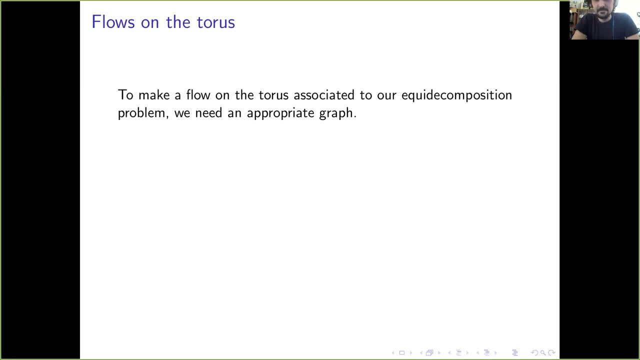 OK. so to make a flow that's related to our equity decomposition problem, we're going to define a graph, OK, and the graph is going to be kind of what you expect, right? We've been talking about taking an x and moving it by these translations. 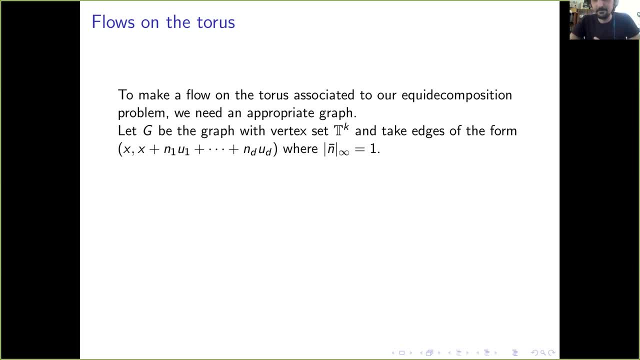 So I'm going to make a graph just by pairing up things that are sort of norm one away from each other. OK, and then what did we prove? What was our continuous approximation to an equity composition? We took translations U1 through UD that satisfied the discrepancy estimates for both A and 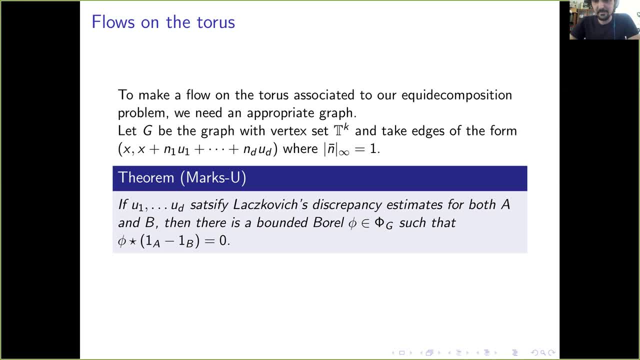 B. and then we found a bounded Borel phi, this function on edges so that under this star action, it takes the difference of the characteristic functions of A and B to zero. So let's maybe this, David, this was the source of your question earlier. 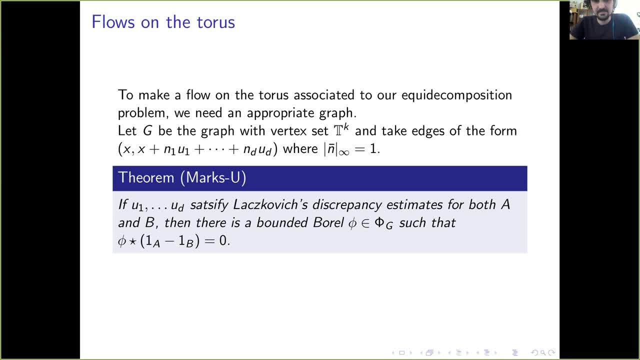 How is this going to be? How is this going to be related to equity compositions? It's this characteristic function of A minus characteristic function of B. So I'm thinking of myself as assigning mass one at points of A and mass negative one at points of B. 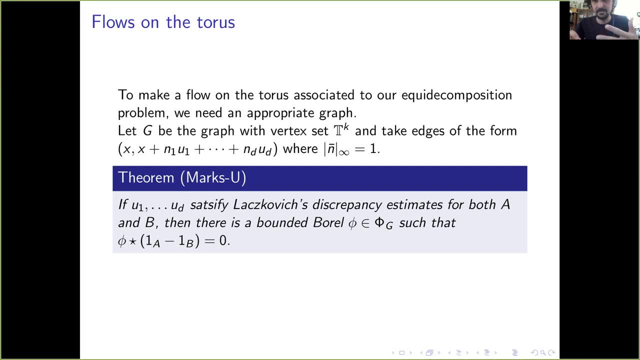 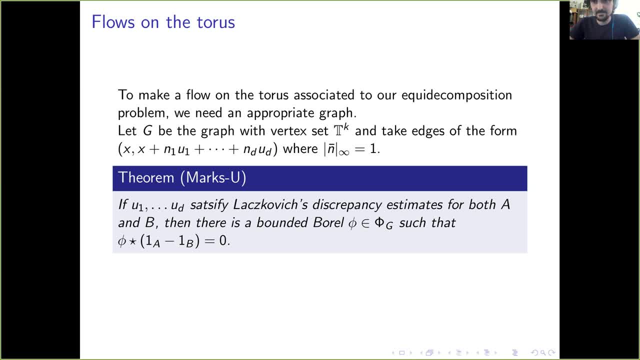 I'm I'm Sending this difference to zero And I'm sort of trying to cancel out the positive mass of A with the negative mass of B. So maybe a clearer way to restate the conclusion here is that actually we can think that when 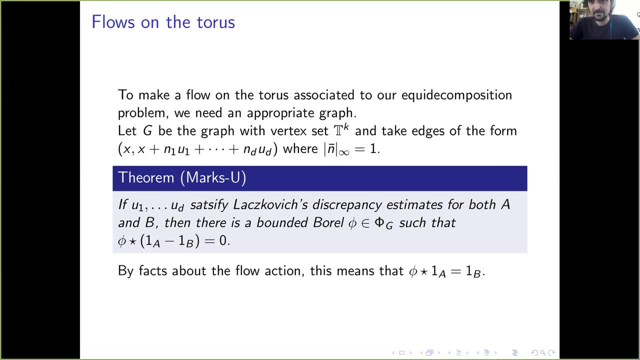 I apply this phi on just the characteristic function of A. it should turn it into the characteristic function of B. I think that that's probably a better way, because phi is telling you somehow how to redistribute the mass of some points, Right? So I have this phi and I apply it to a function that gives mass one to every point in A and then magically, by this rearranging procedure, it produces the characteristic function of B. 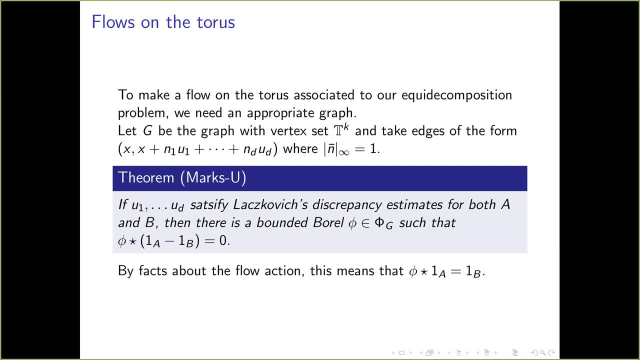 it's been said, just to be super sure, that that equality is like actual equality, is not like up to uh, that's right, that's, it's literal, literal equality, that's right. so, um, yeah, and the thing that's powering this is really those discrepancy estimates, i mean you. you could imagine, um, if you just picked an a and a b and picked some. 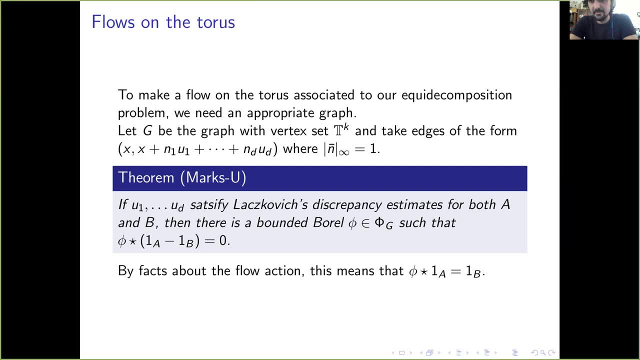 translations. maybe badly. then the points of a and b wouldn't be nearby each other at all in the action. right they, maybe the a and b- are so badly distributed inside this, the orbits of this action, that you, you can't do anything. okay, but the discrepancy estimates tell you that if you 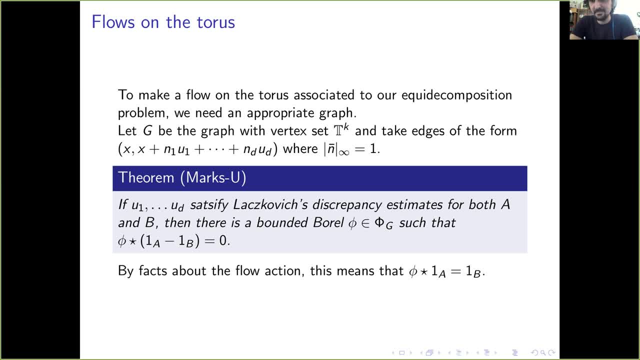 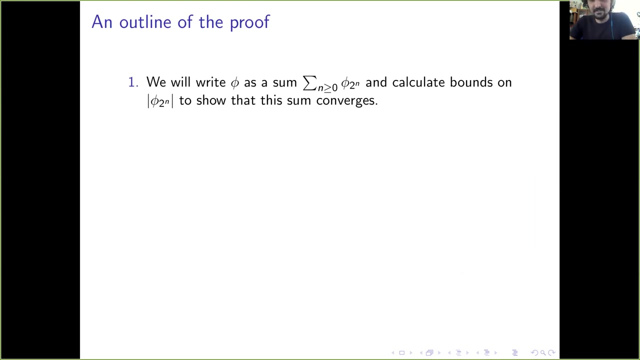 randomly choose enough, enough translations, then actually there are going to be points of a and b close to each other, but not only that. you get this kind of bounded flow between A and B. OK, so I am running out of time, but I think I can tell you just an outline. 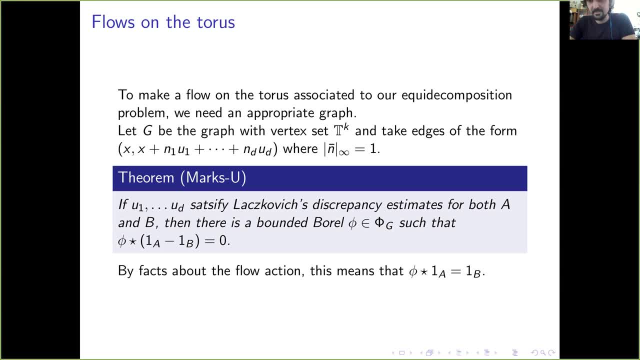 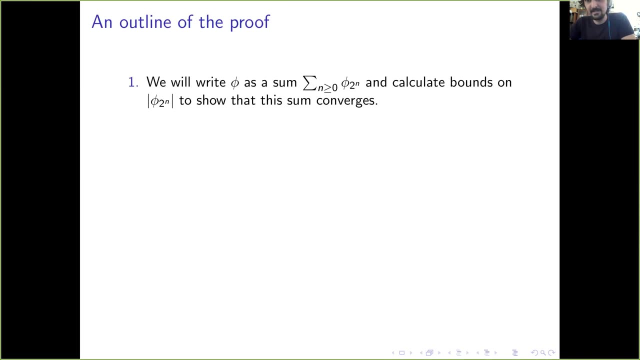 of the proof of this theorem. So in the original paper we had some complicated procedure for making this flow And recently, over the past summer, we found a much simpler one, like extremely, extremely simple. So I will tell you that in the next two slides. 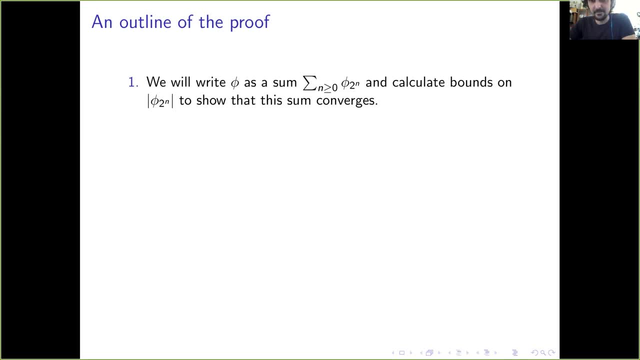 and then I'll be done. So we're going to write the final flow phi as a sum of these phi, 2 to the n's, And we're going to show that this sum converges. absolutely OK, then we're going to define functions- fn. 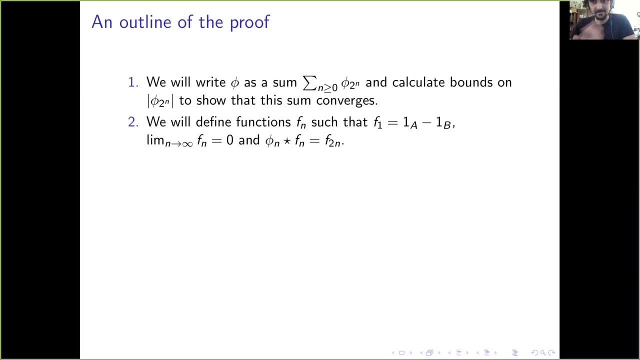 where f1 is the difference of characteristic, So we say f1 is the difference of characteristic function. so that's the starting state. The limit of the functions is going to go to 0 as n goes to infinity And this crucial property is going. 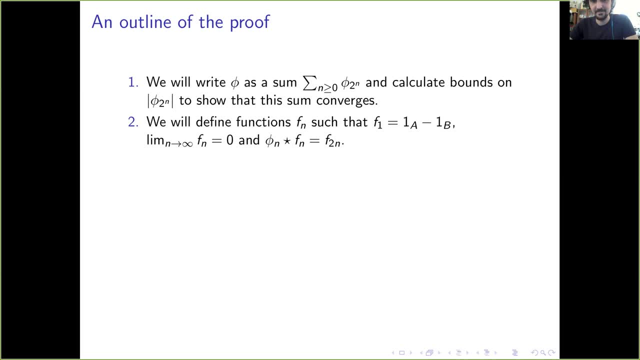 to be that the nth phi. we're using phi 2 to the n in the sum, but whatever. so the n-th phi. if I apply it on fn, I get f2n. OK. phi n's are like transitioning you through the the sequence of f's, okay. so why? why are these two? 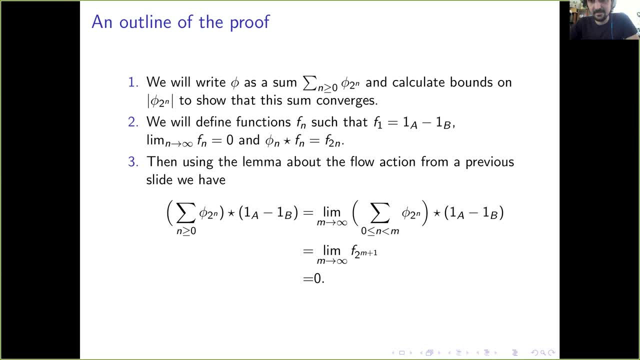 bullet points enough. um, it's this extremely simple calculation using the lemma from a couple of slides ago. so i apply this phi, which is the infinite sum, on the difference of characteristic functions. there's this lemma that says that i can interchange the sum and the limit with the action. 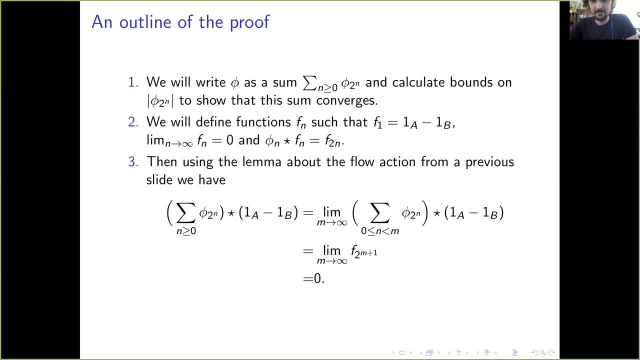 of star. so that's what i did in the first line. and then there's this uh statement at the, just before the lemma that says: um, you know, acting by a sum of flows is like acting by the, acting on them one by one, right. so the characteristic function of a minus the characteristic function. 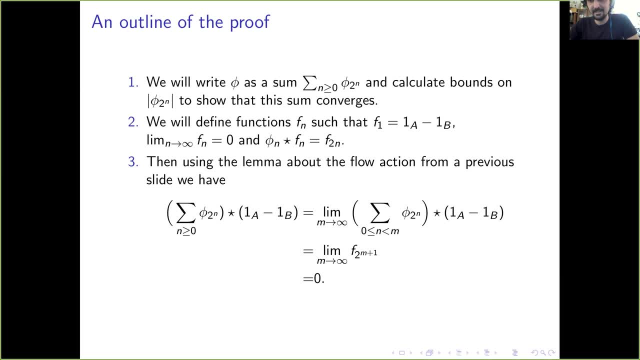 of b, that's f1. and when i apply phi 1 on that, i get f2. and then when i apply- oh dear um, phi 2 on that, i should get f4, etc. okay, and so the the result of iteratively applying these phi 2 to the ends on the difference of the characteristic function of a and b is that i get. 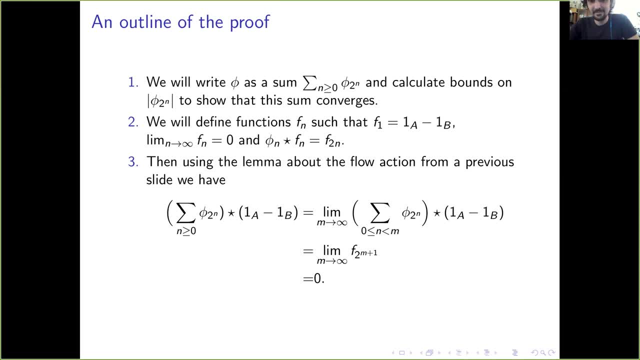 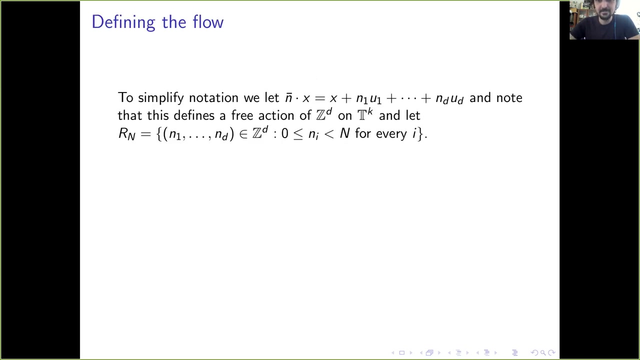 f2m plus one, okay, and those, those functions go to zero as n goes through, and that's it, okay. so it's enough to to construct um functions f and functions cn, uh, like this, all right. and so what are those functions? um, i'm gonna give you a definition of them on this slide. 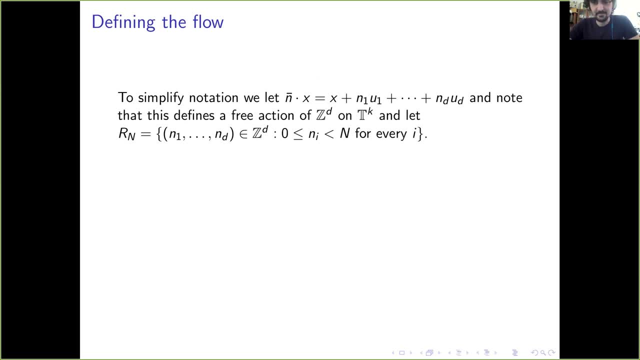 and then we'll stop. uh, sometimes, things really turn out to be much simpler than you make them initially, so this is one of the uh morals of today. so, to simplify this, we're gonna um define an action that we probably should have defined earlier. um so n bar applied on x is just x plus. 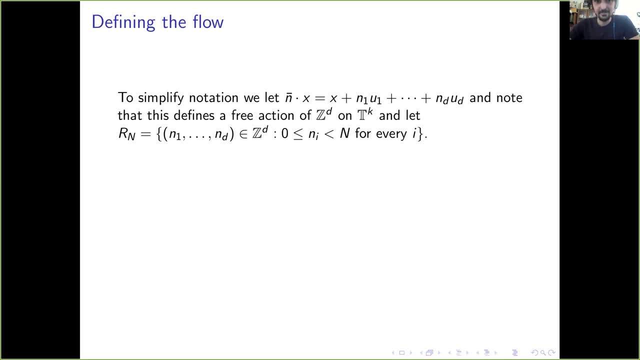 this thing that we've been talking about all along and that defines a free action of z to the d and this rn, um, i guess this is kind of a relative of sn of x from before, but it's just the, the natural number version. so rn is this: uh, square inside z to the d. 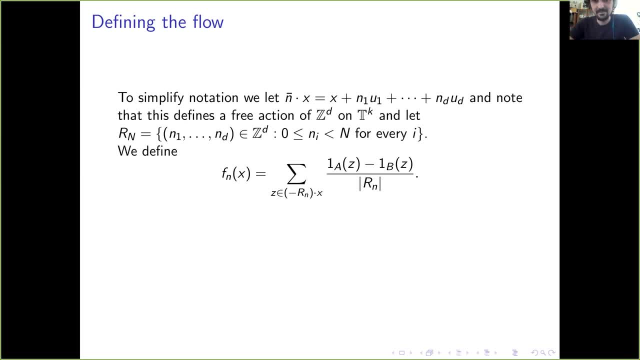 so what's what's fn of x? um, it's some kind of averaging function. it's some kind of averaging function. so fn at x. it returns you the average of the difference of characteristic functions between a and b over this square, which is like down into the left of x inside the action. so that's where the sum is over z in this minus rn. 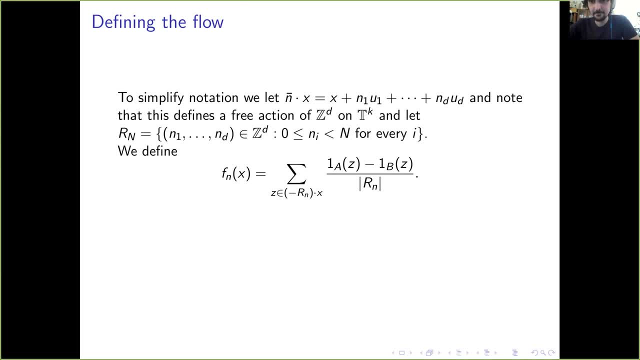 applied on x And then phi n is given by this slightly more complicated formula. But the formula here is motivated by needing to transition between fn and f2n And the proof that the fn's go to zero and that the sum of the phi n's is absolutely. 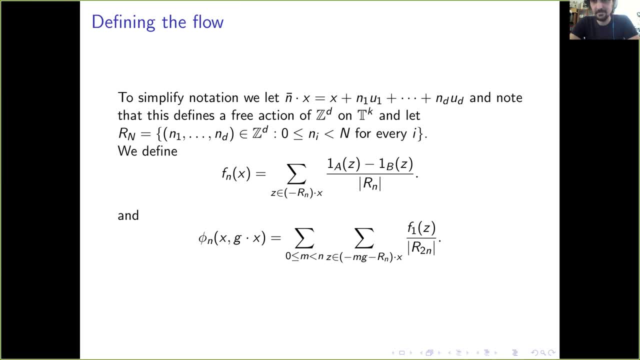 convergent sum of the phi 2n's. whatever you want is absolutely convergent. those precisely use Laskovich's discrepancy estimates. Okay, and it's maybe not too hard to see that the discrepancy estimates should be useful here. So 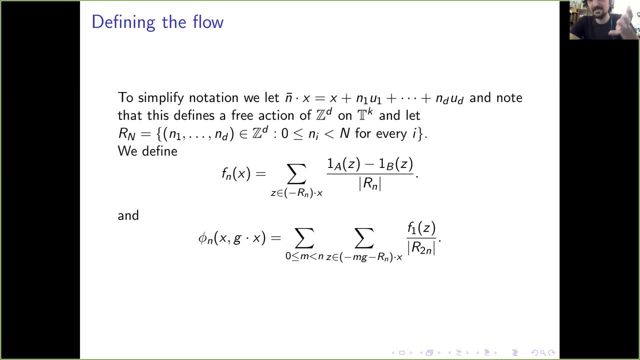 you're using the fact that both a and b satisfy the discrepancy estimates and have the same Lebesgue measure, So inside every square they should have roughly the same number of points. Okay, so I guess maybe we've come all this way. I'll give you one last slide. So, having simplified, 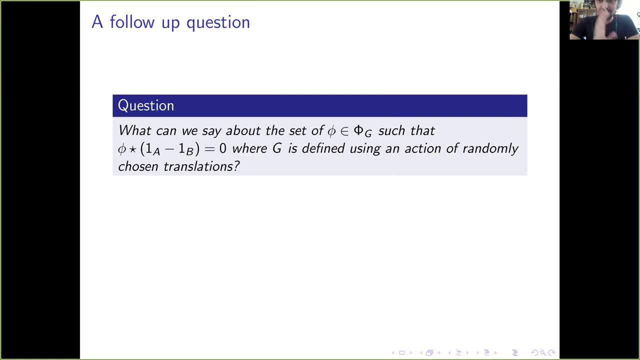 this proof. a question that I had was: what can we say about the collection of phi's that satisfy this, sending this difference of characteristic functions to zero? Right, we constructed this one by a relatively simple formula, So we're going to use this one. So we're going to use this one. 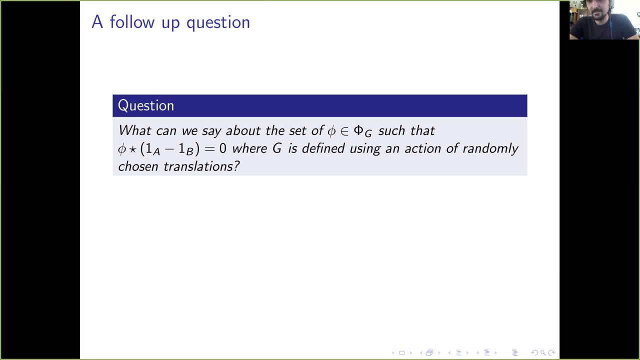 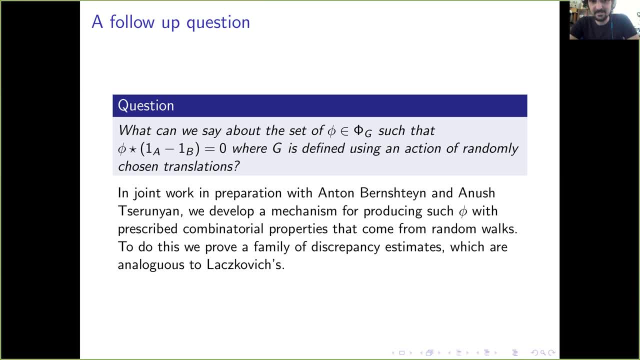 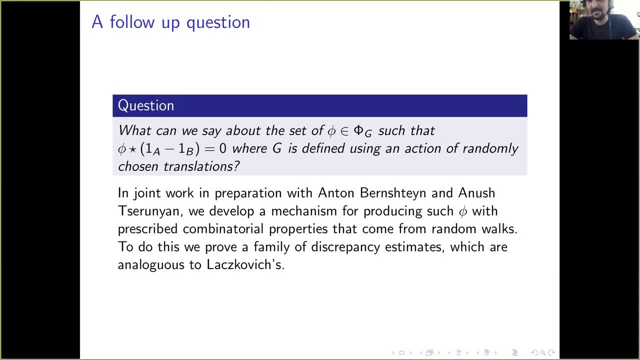 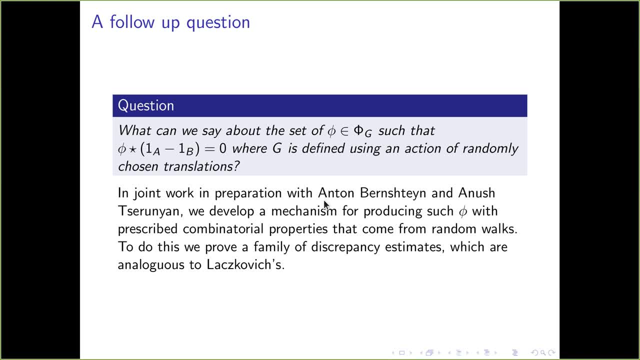 Thank you, Spencer. Actually, I think you're doing great, because you started really late and you caught us up a little bit, So I hope you didn't hurry too much. No, this was great. That's exactly what I hope to say. 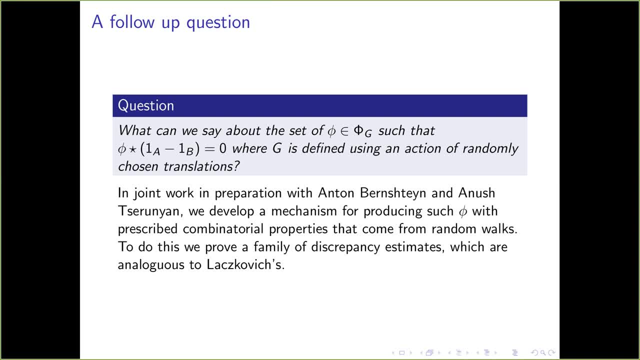 Fascinating talk. Are there any questions? Yeah, I have a question and a half, let's say. The first one is like: so you have been saying about taking these translations randomly, So what is exactly what you are trying to avoid? 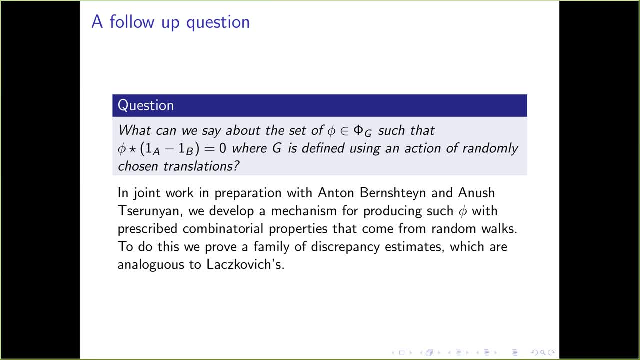 So that measure. one said, what are you taking away? And I'm like, OK, let's see, It's a little bit complicated. So let me think about what I can say in just a sentence or two. So these squares inside the, let's say, the, you know, the. 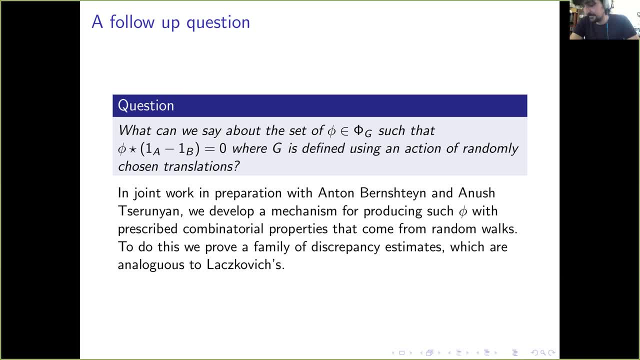 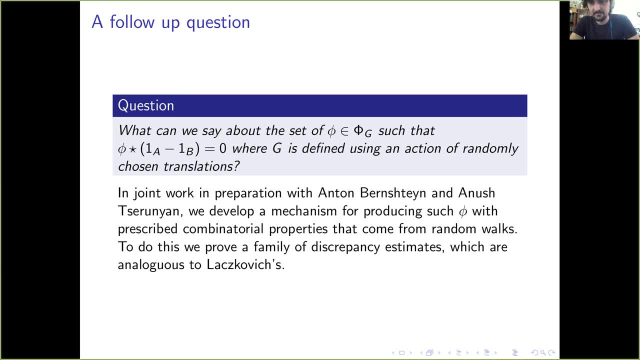 which is just a normalized counting measure right, Which is really in this discrepancy estimate, that term on the left-hand side where we're counting the number of points of a. that's like a normalized counting measure of a inside that for that issues. 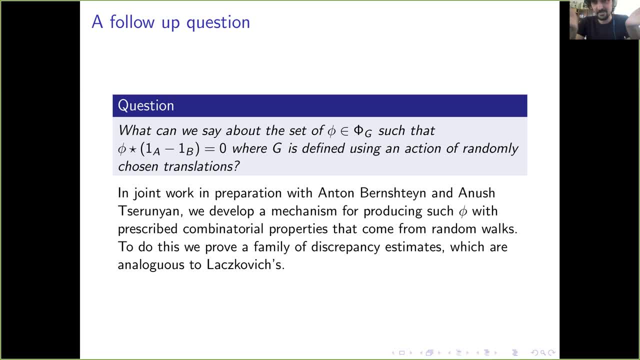 square right. so the the discrepancy is really measuring like discrepancy between Lebesgue measure and the, the, that normalized counting measure for a. okay, so what are we bounding when we, when we randomly choose the translations? what we're bounding actually is um the Fourier coefficients of that measure, of that uniform measure. so it turns out that the, the Fourier. 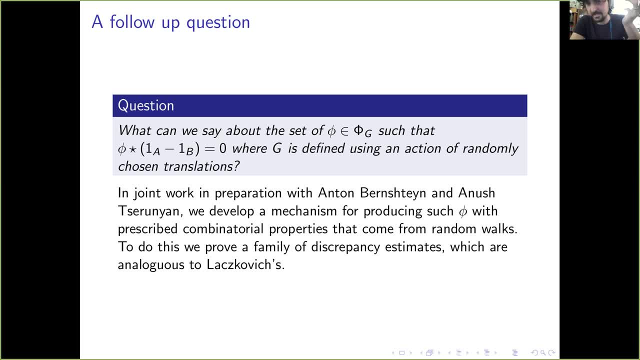 coefficients of that measure are actually independent of which square that you take um and the randomly choosing the translations will improve your bounds on those Fourier coefficients, which is what you need to to prove this discrepancy estimate. okay, okay, so like you're taking away these like Fourier dependencies somehow at each step, let's. 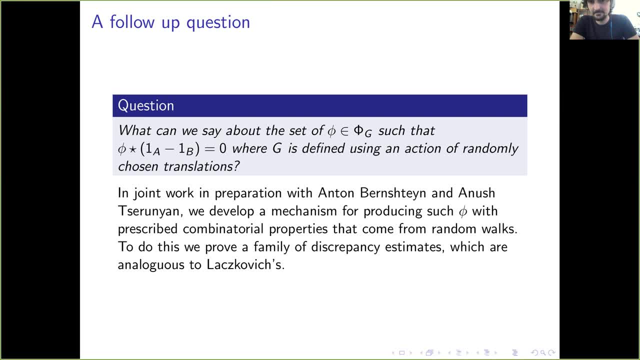 say like, yeah, that's right. yeah, yeah, that's all. that's pretty interesting. yeah, thanks, yeah, and i just realized that my half question was not a question. so yeah, i, i'm done. great. um, i actually have more questions, but in the interest of time, i will ask them i. 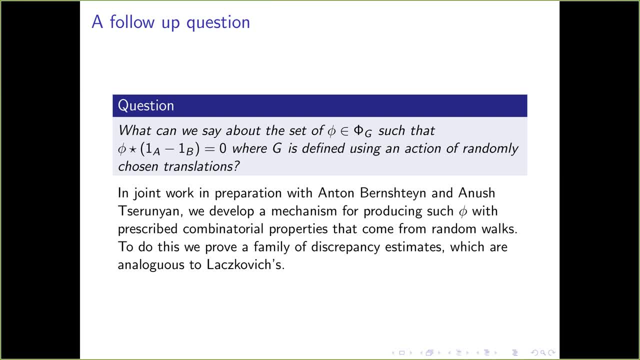 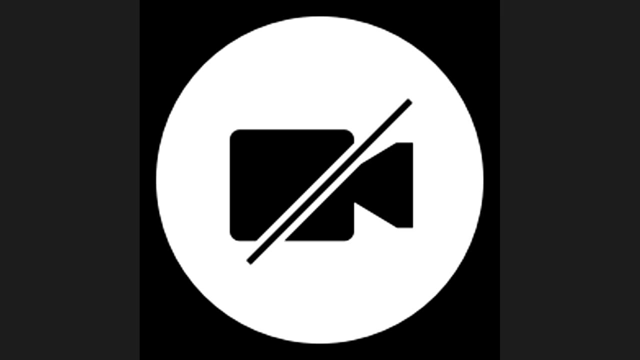 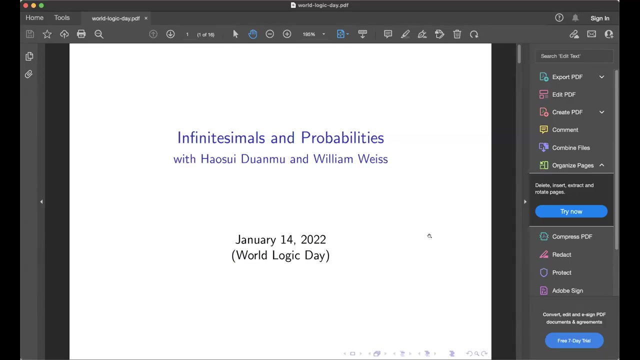 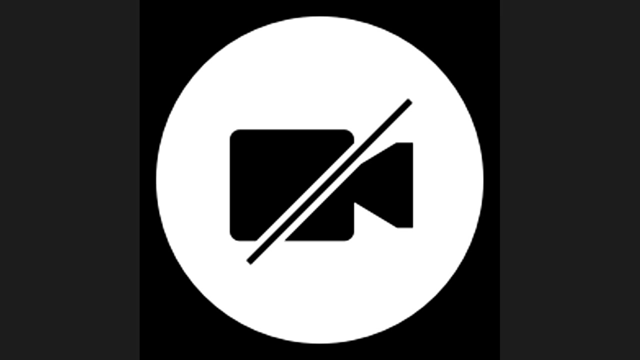 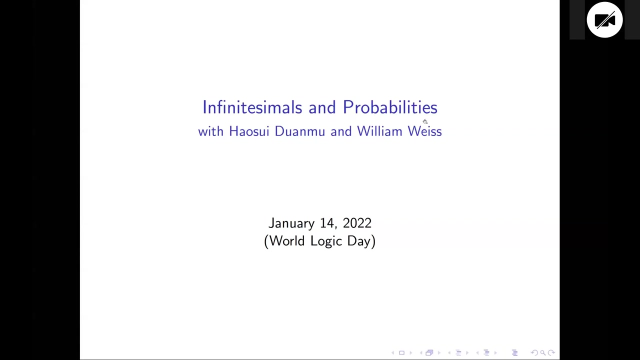 don't know when i, when i get a chance, uh. so, uh that, thank you again, and that's it for today, thank you. that brings us to our last speaker, and that's me, so let me get my slides ready. all right, does this seem to be working? 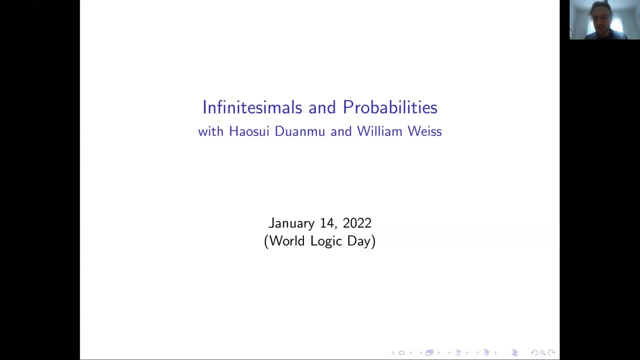 i guess cool, okay, um, oh, so that happened. can you see the slides move as well? yes, okay, good, okay, great, all right, so my title is infinity binoculars at the 思بار, but i'm also a postdoc at u of t and i work with uh bill, uh william weiss and uh who was? 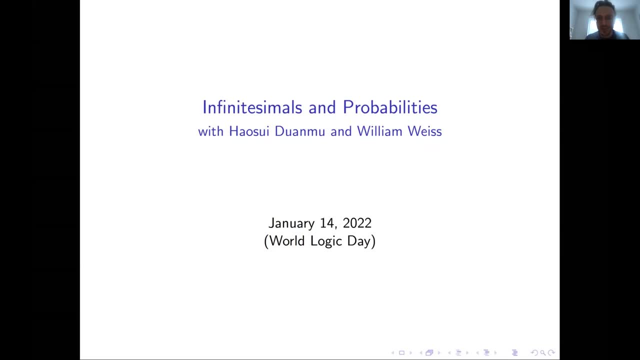 a former postdoc, i guess, here, who just left and is now a professor in china. all right, so my i have an outline here. i will first tell you about non-standard analysis at very high speed and then i will tell you about the non-standard analysis. that's the point. 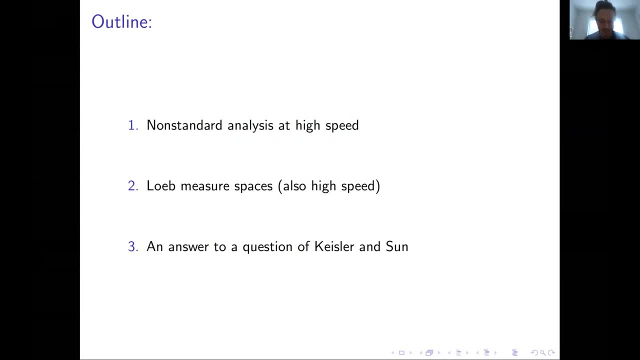 here, because at that point i was already at that point i was already thinking about doing something, about a thing called lobe measure spaces. so this is non-standard measure theory- uh, also at rather high speed, and then maybe i will be able to actually prove something, and 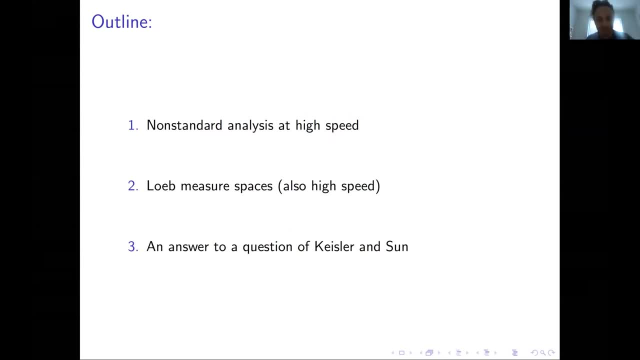 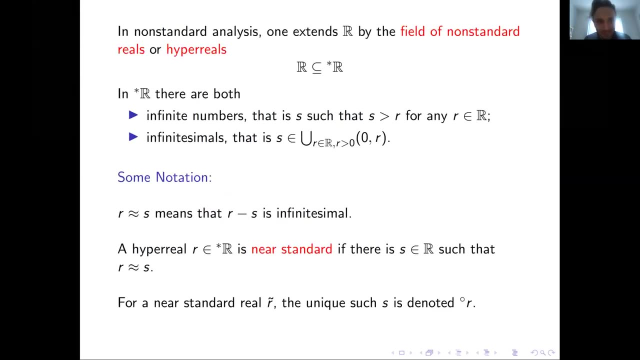 that's an answer to a question of kiesler and sun concerning lobe measures, spaces. all right, so non-standard analysis, um uh, in non-center analysis, you extend the field of real numbers, uh, to a larger field, the field of non-standard reals, also called hyper reals. 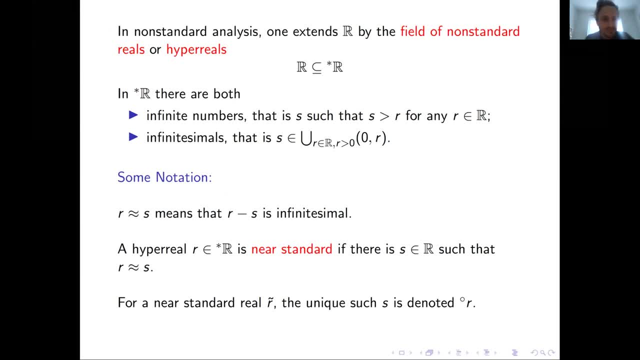 and they've got this star on the left, the star r, and, as you might know, in star r there are both infinite numbers. so numbers s that are bigger for every standard real are bigger than r for any standard real. r and there are also infinitesimal numbers. so 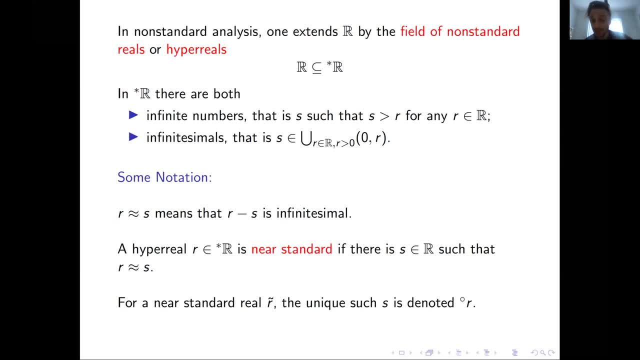 positive numbers, s that are smaller than every positive standard real. so they sit, these non-standard real numbers. they sit very, very densely in the standard real numbers and they also go off to the side. and here's some notation that you hopefully know. you say r is approximately equal to s, to mean that they're, they're infinitesimally close to each other. 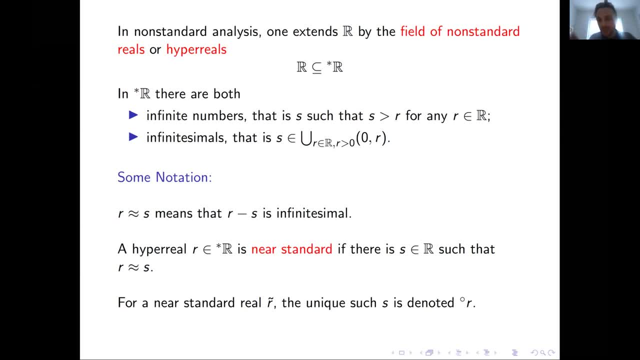 and you call a hyper real near standard if it's infinitesimally close to a standard real, so it's not really far off to the side and infinite. it's also sometimes called a finite hyper real and for every near standard real, one that's infinitesimally close to a standard real, you. 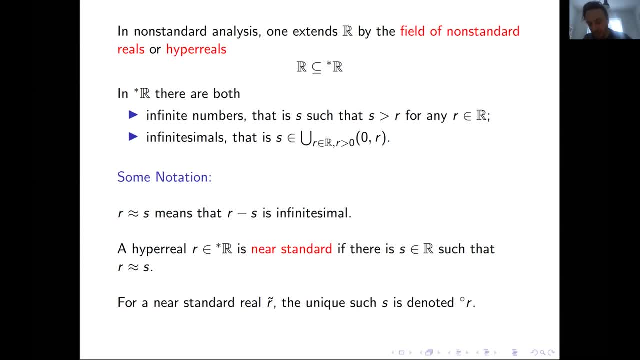 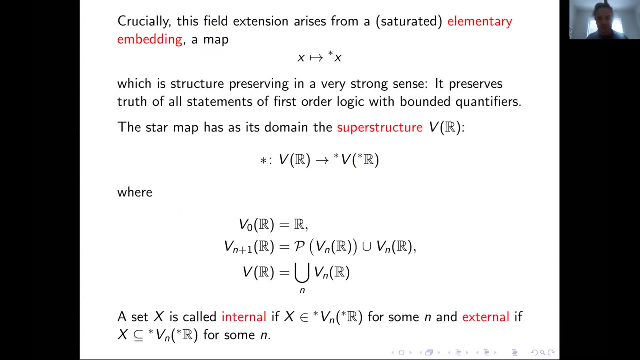 denote that standard real by circ r, upper circ r. so that's the, that's the, that's a standard real that you're infinitesimally close to. it's also called the standard part, and the circ map is called the standard part map. all right, so i mean, so far this is just really notation, the, the. what makes it interesting to? 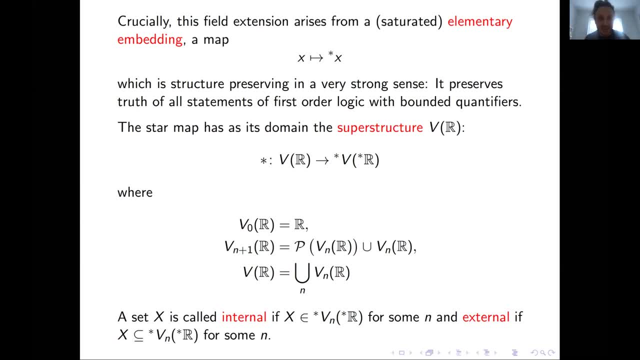 look at this field extension is that it comes from a saturated elementary embedding, so that's a map that assigns to it really more or less any mathematical object, x, its extension called star of x. so you always write the star to the upper left and the the crucial thing is um that this: 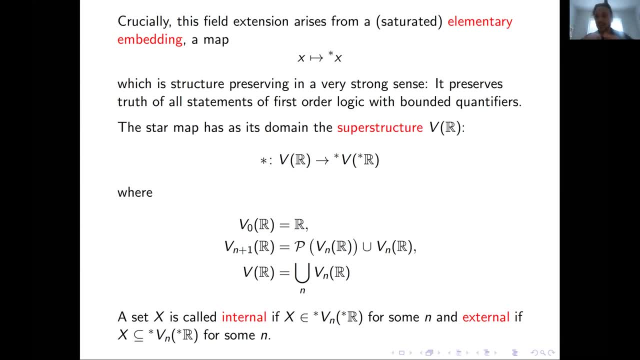 is a structure preserving mapping, it's not just a field, uh homomorphism structure preserving in the strongest possible sense that you can imagine. it preserves truth of all statements of first order logic with bounded quantifiers in some sense. so i mean, uh, i'll just have to gloss over a. 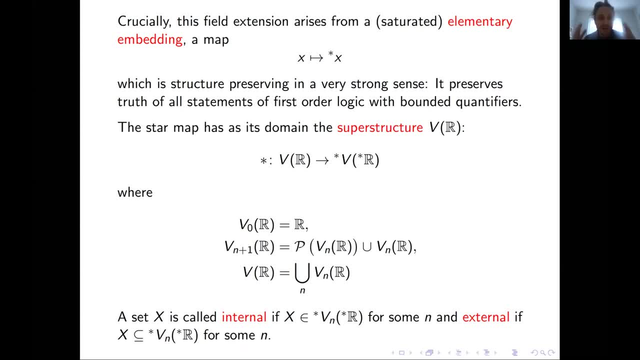 lot of details here because it's a 20 minutes talk, but i can hope you can get some idea out of it. so the star map has as its domain, um, the star map has as its domain, um, the star map has as its domain, uh, what's called a superstructure. that's a little universe built over the real numbers. 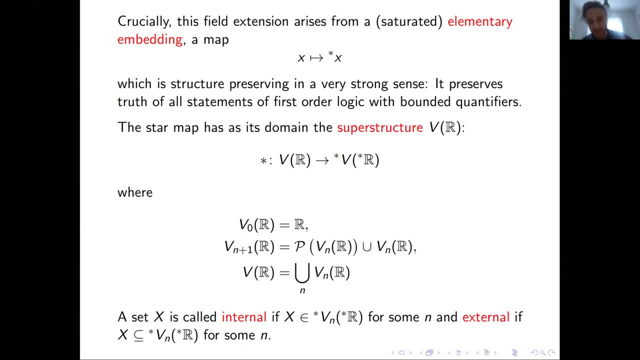 call it v of r, so it goes from v of r into star v of star r, which is just the target model for this map. and um, you know, the super structure is just built by first taking all the fields, then you take all the sets of reels, then you take sets of sets of reels and so on. uh, you go for accountably. 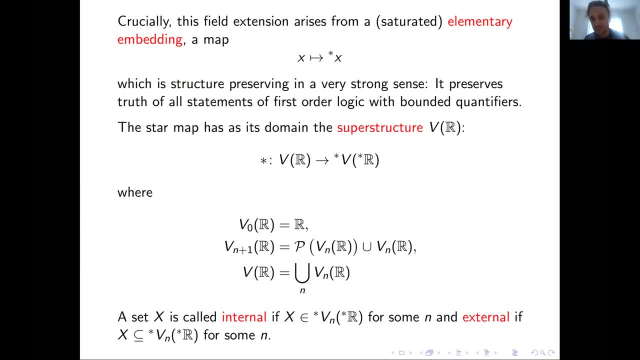 you get this super structure and to anything in this structure you can apply the star map and you will preserve all the properties this this thing has. uh, so the the reason we're doing this is because, if we're doing probability theory, we want to apply the star not just to reels, but also to 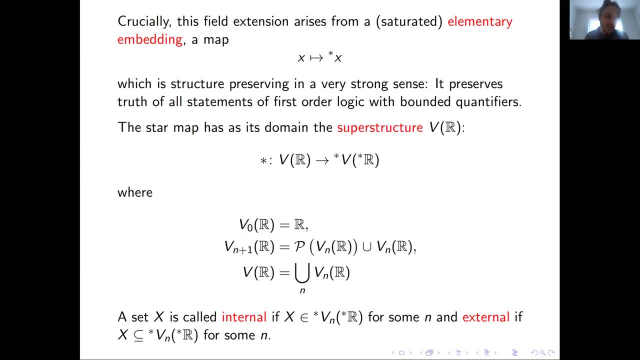 sets of reels, um, and i guess i could have stopped at v1 of r, but you know, i just couldn't help myself, okay. so, um, a set is called internal if it's an element of one of the levels after you've hit it with a star, so it's an element of the target model, uh, and it's external if it's just a subset of. 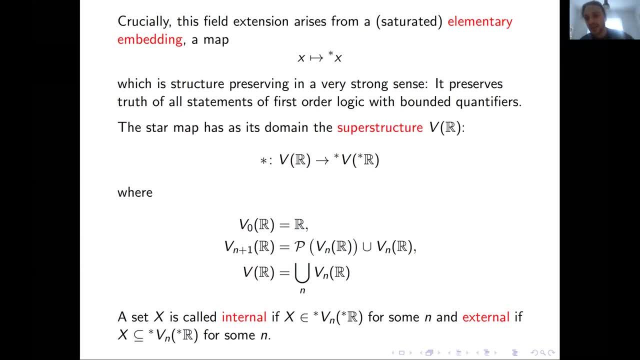 the target model. so the the. the funny thing about this, about non-standard analysis, is that um the, the target model on the on the right side, the star of the superstructure, it doesn't really know about all of the subsets it has. it doesn't really know about all of the subsets it has. it's. 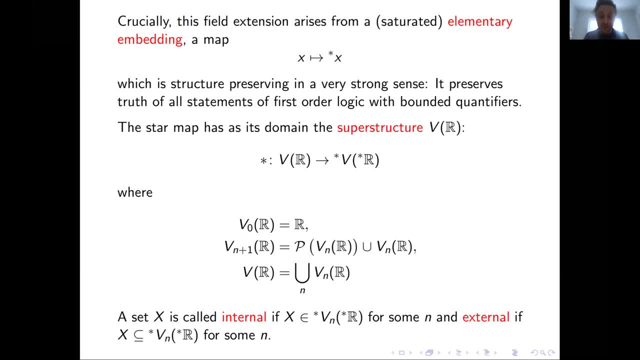 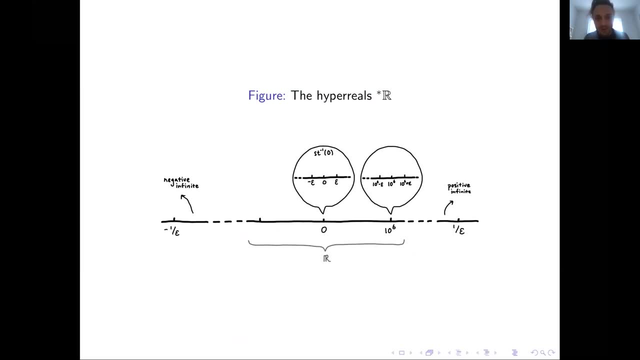 It has internal subsets which it can talk about, and there's also external subsets that it can talk about. All right, so here's something to calm you down. if you thought this was confusing a picture of the hyperreels- They're really not that complicated. 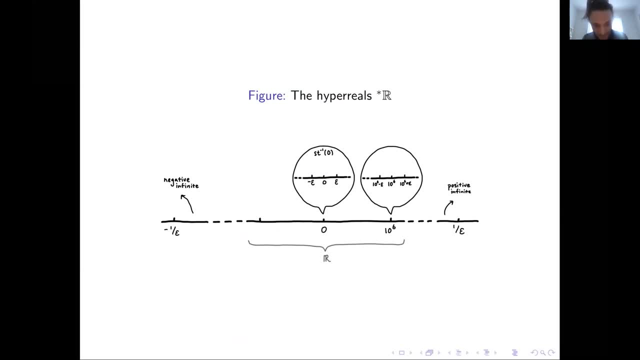 In the middle. here you've got the standard real number line and then off to the side you've got infinite hyperreels and if you zoom in really close to a point like the point zero, you'll see all the hyperreels which have standard part zero, so everything. 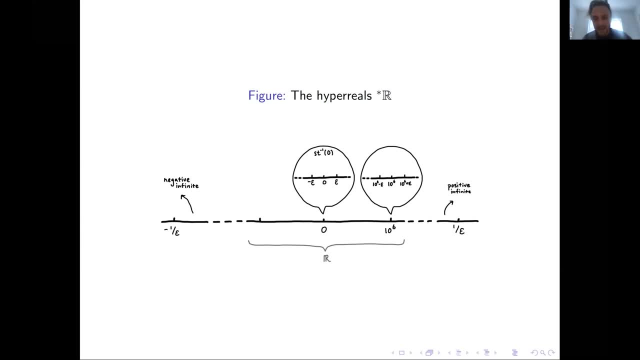 that's infinitesimally close to zero. that's called the monad. Every point has a monad. right Ten to the sixth also has stuff that's infinitesimally close to it and of course, if you take one over an infinitesimal then you land in the infinite. 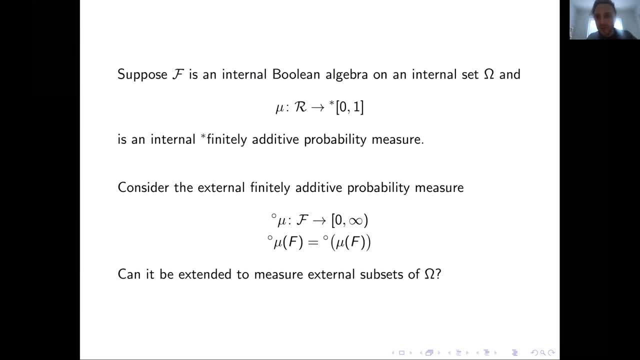 All right, so those are the hyperreels. Okay, now what are lobe measures? We're off to non-standard probability theory. So suppose that F is an internal Boolean algebra on some internal set omega. so now we're in the non-standard part of the universe in this V star and you've got some internal star. 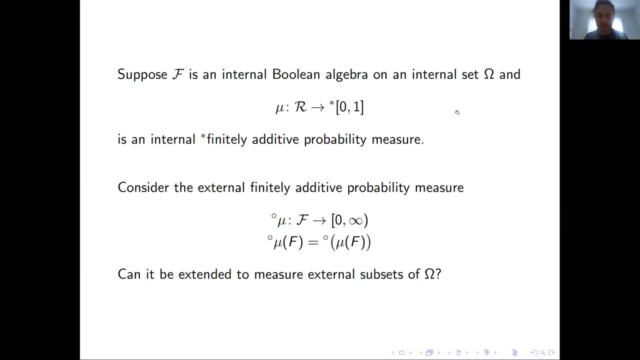 finitely additive probability measure. So you could just say finitely additive here, if you want. that's maybe easier to think about. So the probability measure has values in the star of zero one, so it can take hyperreal values And then you can consider an external finitely additive probability measure with domain F. 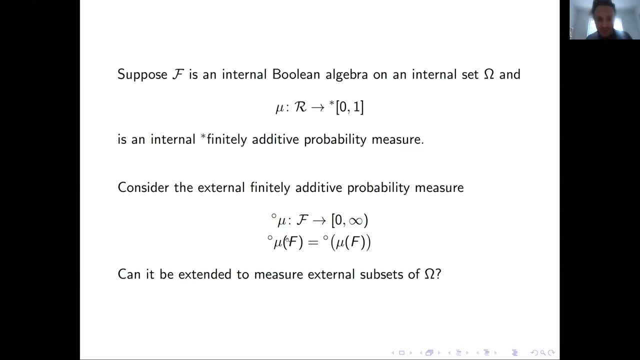 by just taking the standard part of the measure of each set. Okay, So we have a finitely additive probability measure defined on this internal algebra of sets and you could ask: can you extend it to an external measure, to an actual measure? 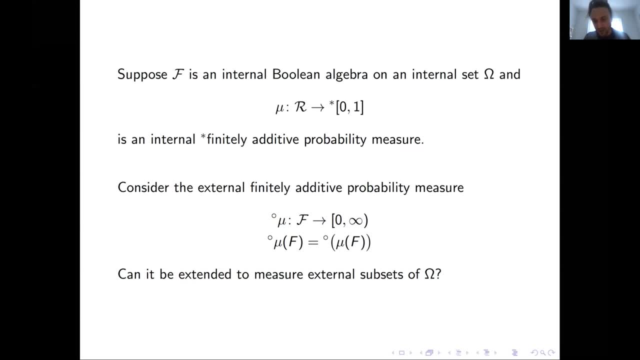 a sigma additive measure on the subsets of omega? And the answer is yes, And although I can't give you too many examples in this short talk, Okay, It's incredibly useful to do so because, actually, a lot of measures that you encounter in your 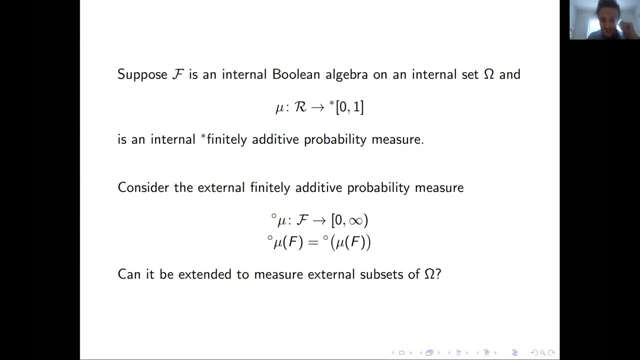 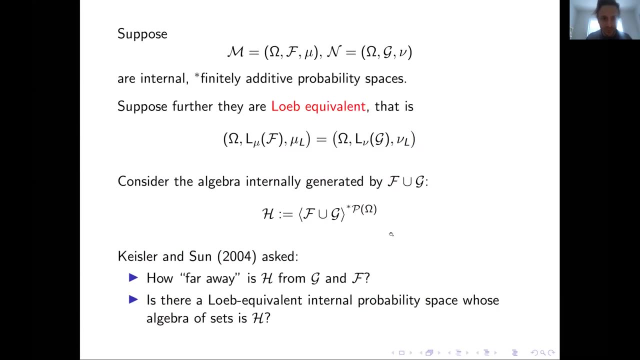 life are of this form. They're extensions. they're extensions of such an internal measure, and that's sometimes very useful. Oopsie, All right. So so can you extend what is going on with my slides? I'm sorry. 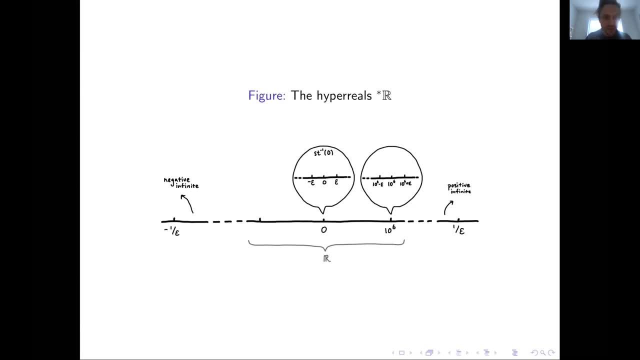 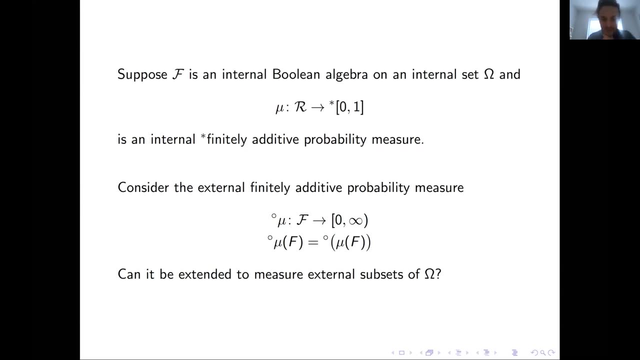 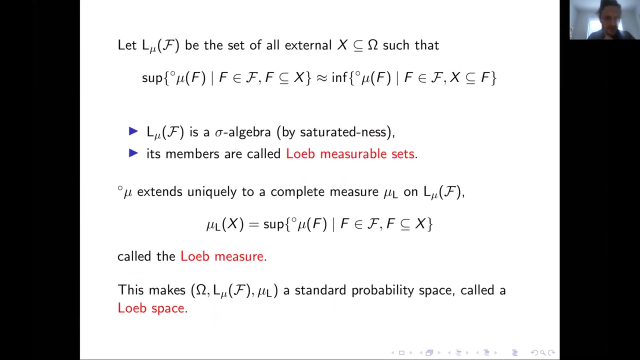 Right, Okay, Okay, All right. So I said: can this CERC measure be extended to an external measure on subsets of omega? And the answer is yes, And this is how you do it. So you look at the set of so-called lobe measurable sets L, mu of F. It's the set of all external. 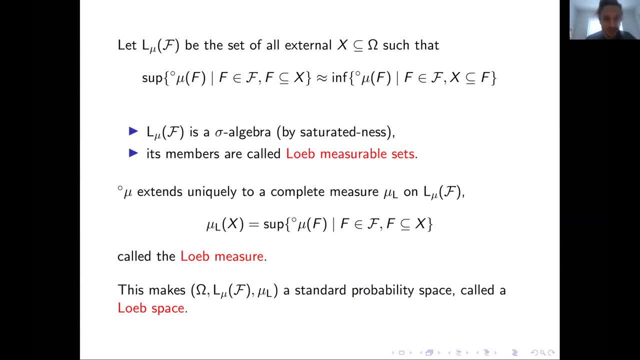 subsets of omega which satisfy this condition here. Okay, And basically you're using a Carathéodory extension theorem. oh, and the approximate sign in the middle should be an equal sign. That's a typo. So you take the Carathéodory extension of the circular measure to the largest possible. 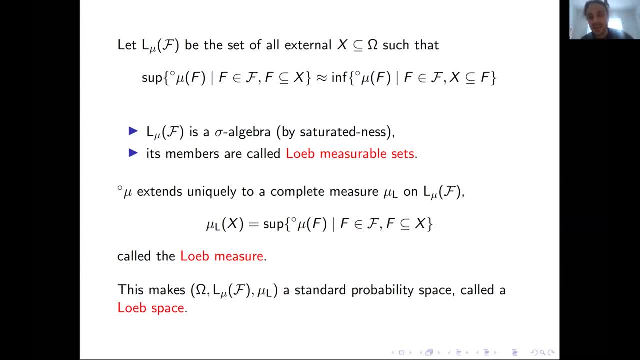 set, or at least the set that's given, that's given to you by this Carathéodory extension procedure And that's the. basically, you're looking at the, at the inner measure and the outer measure And you you call a set lobe measurable if it's inner measure and it's outer measure. 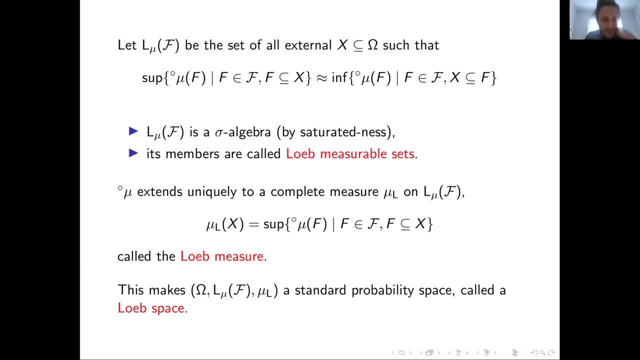 agree. And the funny thing is that this, this set L, mu of F turns out to be a sigma algebra. So that's really nice. And this is by a property of the elementary extension called saturating. And you know, this is the only time we're going to use saturatedness or we need it. 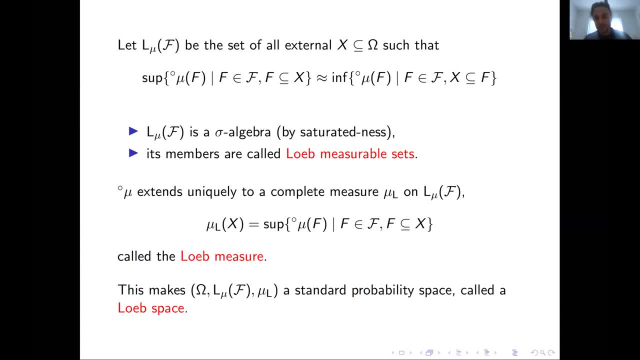 So I will not talk about it at all. but it's just, you know, by a property of this, of this elementary extension, this turns out to be a sigma algebra. It's members are called the lobe measurable sets, and now you can extend the measure uniquely. 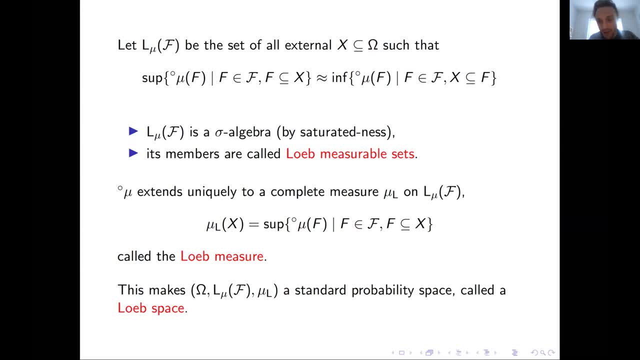 to a complete measure which is called the lobe measure, mu L, on this set of lobe measurable sets, Bye, Of course. So you're equal to this supremum up there where the soup of the CERT inner measure, if you want, or you could also take it to be the info of the CERT outer measure, is the 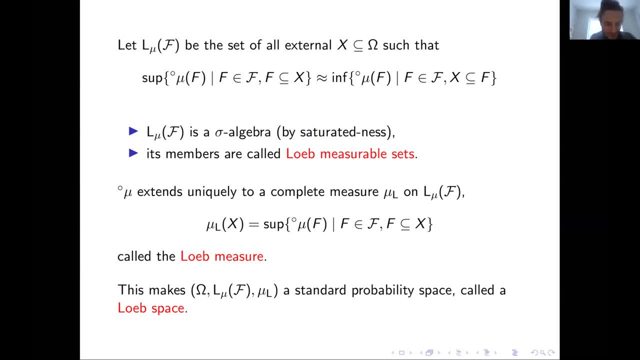 same thing. This is called the lobe measure. So this makes, so you get a standard probability space now, and it's. this is called a lobe space. So it it. the. the underlying set is still your set omega that you started out with, the. 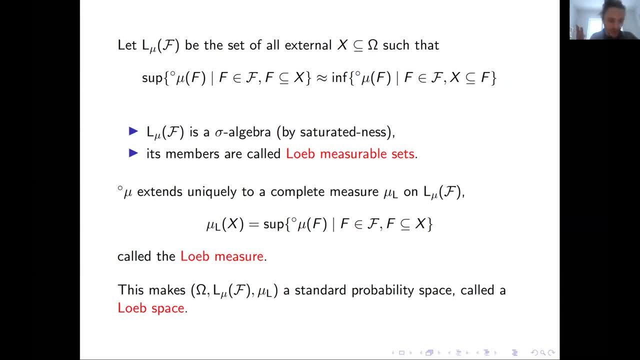 internal set, But the, the, the. Okay, So measurable sets are now a sigma algebra of inter, of external subsets of omega, And you've got an actual sigma additive probability space here. And the funny thing is, and this is why people are interested in this, that a lot of spaces 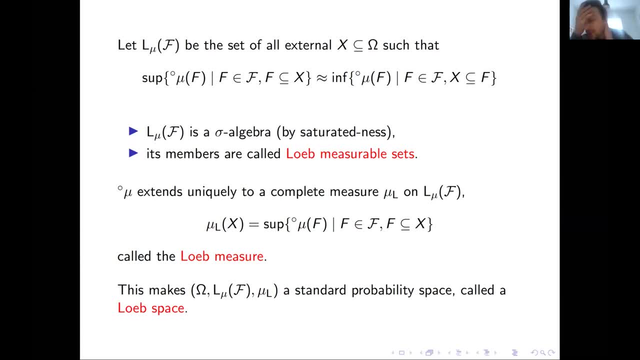 a lot of measures arise in this way. For example, you, the bag measure you can think of As as arising in this way, And and so on, many other uh measures. the wiener process can be constructed in this, random walks can be constructed. 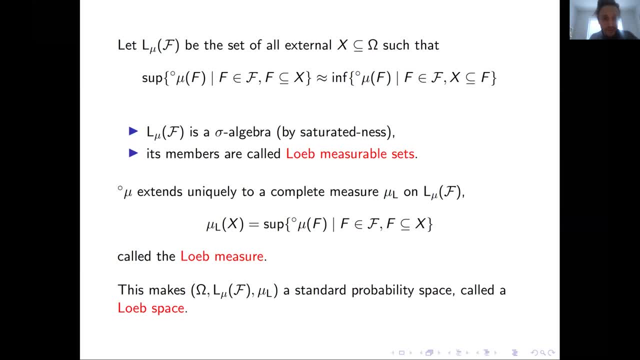 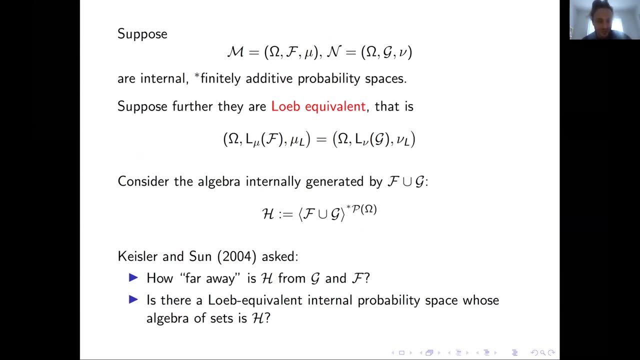 in this in this manner. so this is very useful. uh, the useful thing is i should say that, um, the f can taken to be hyperfinite, uh, most of the time, and that's what makes it what, what makes it really useful. so here is the question of kiesler and sun. that, uh, we answered in our paper and that 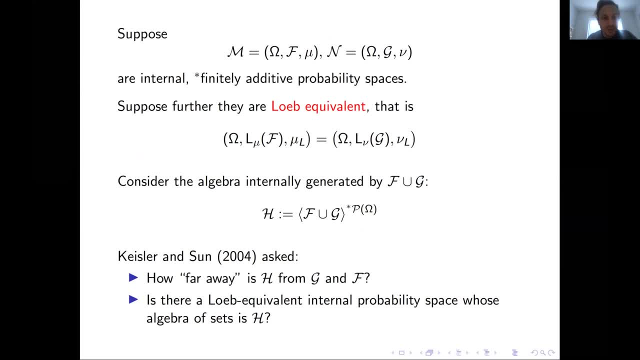 i want to talk about. so they said: suppose you've got two uh internal finitely additive probability spaces, m and n. they're both on the same set omega. uh, um, they're both on the same set omega, but they've got different algebras- f and g- and different measures- mu and nu. 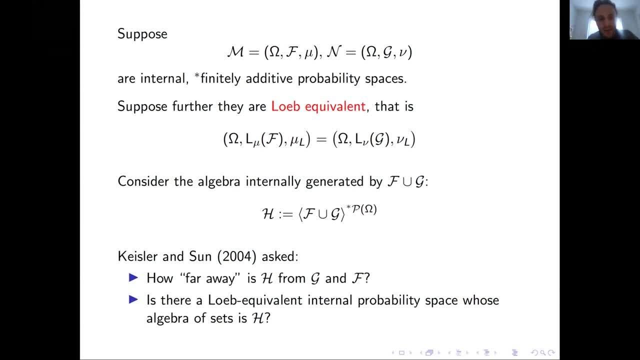 but we suppose that they're lobe equivalent. so, uh, if you take their, the lobe spaces um that generated by these, you get the same probability measure space. so kiesler and sun then asks: so if you've got these two lobe equivalent, uh, internal. 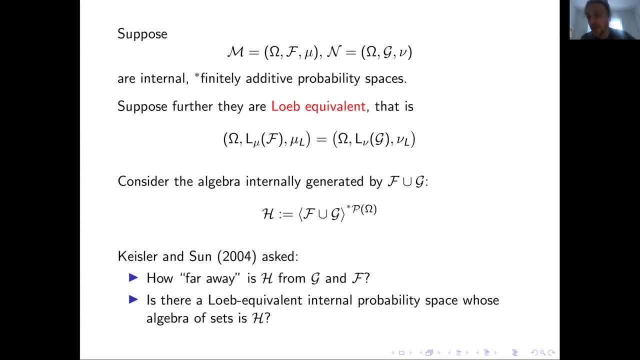 probability spaces. do they have to be close to each other in in some sense? so one way to to say that they're close to each other is: you can consider the algebra internally generated by f union g. let's call this h, so that's um, all the all, the internal, um finite unions of elements of f and. 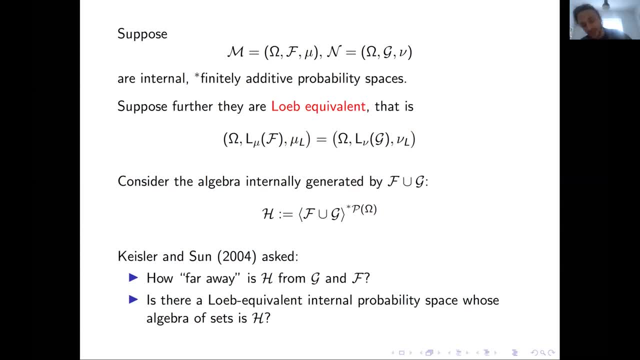 g and complements of finite unions and so on. that's possibly a pretty large object and that's actually the only place i need to use the star map on anything that's not a real um. so you look at this internally generated h and you can ask how far is h from g and f? oh, i guess it's basically the same as asking how far. 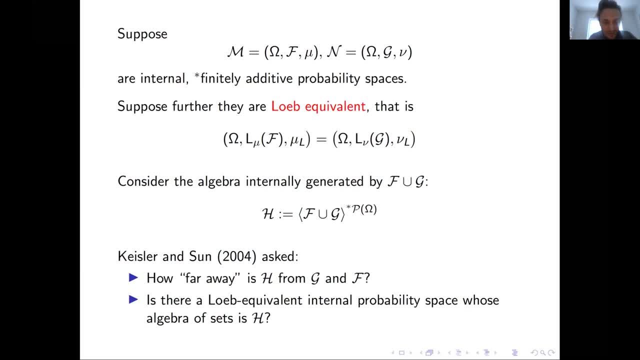 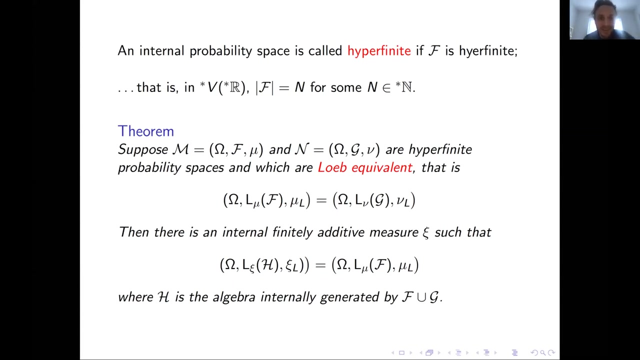 is g from f um. in particular, is there a lobe equivalent internal probability space whose algebra of sets is h, which would mean that they're not very far away. right, because that means that they're not far from each other, and so on. that's why you can ask for a unaltered 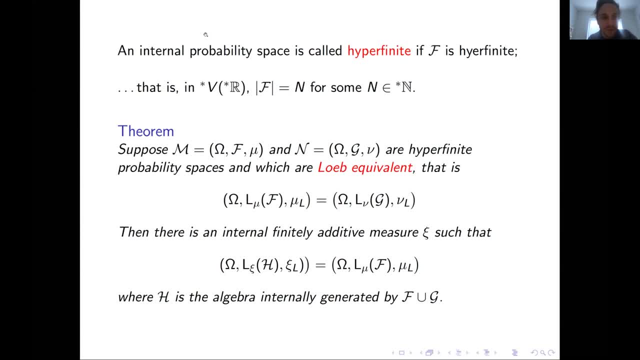 so here let me go back to the previous slide that out in more detail. an internal probability space is called hyperfinite. if f is hyperfinite, there's a p missing there, sorry. and that means that in star v of star r, in this target model f, the cardinality of f is some non-standard natural number, so some n in the star of n. 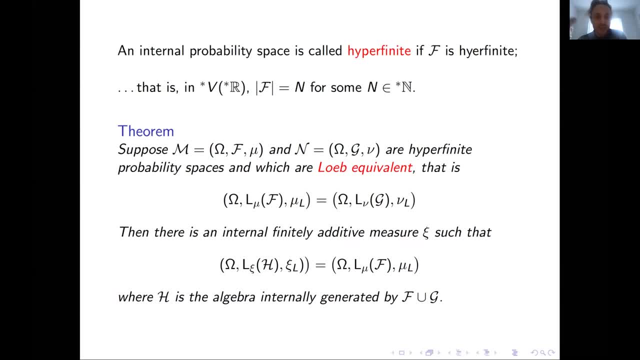 that means that you know the the target model thinks it's it's a finite set. it's not actually going to be finite. it's actually going to be very large in most cases. but you the, since the target model thinks it's a finite set, you can work with it as if it were a finite set, which is a very 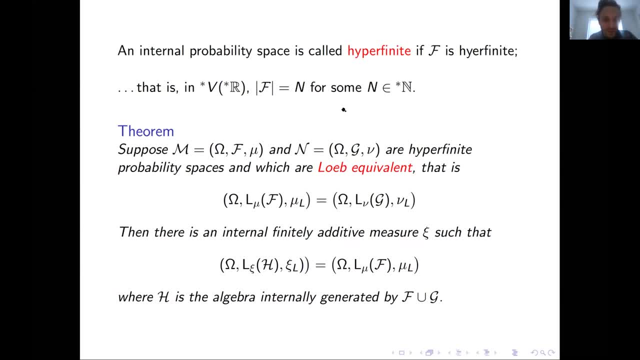 powerful tool. okay, so here's, here's the theorem that we proved. well, okay, i should say again. so the the reason that you're looking at these hyperfinite f is a very powerful tool is that the lobe spaces that you get from such hyperfinite probability spaces- 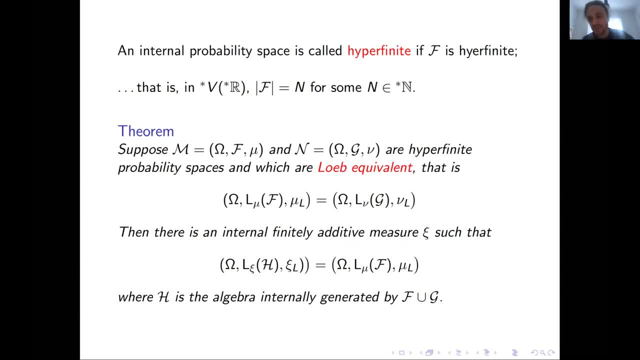 are a very rich class of measure spaces And you find a lot of measures that you work with in practice among these, or sometimes your measure is just isomorphic to a lobe measure module or measure preserving function, namely most of the standard map function actually. 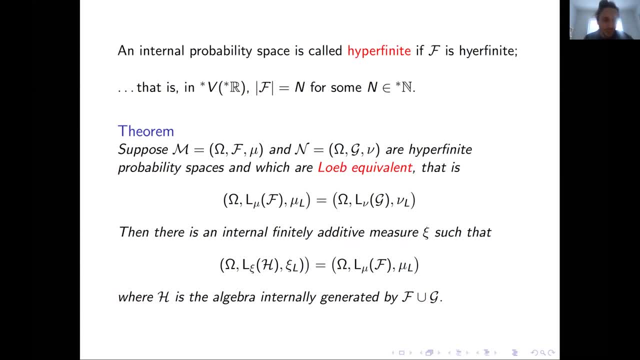 All right, so this is why this is interesting. So and the theorem that we proved is the following: Suppose that M and N are hyperfinite probability spaces which are lobe equivalent, That is, if you take their associated lobe measure spaces. 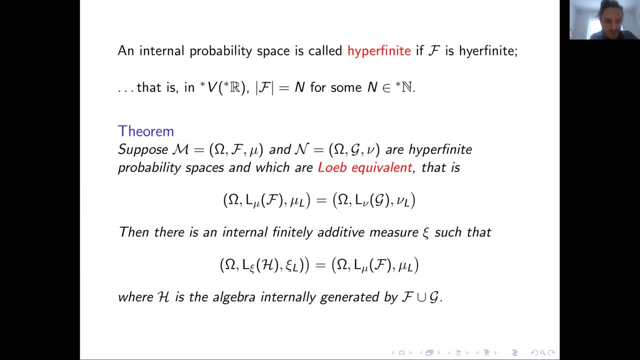 you get the same measure space, Then, indeed, there is an internal finitely additive measure defined on H, such that the lobe measure space generated from this new measure C is again the same space. All right and well, I was going to show you some of the proof. 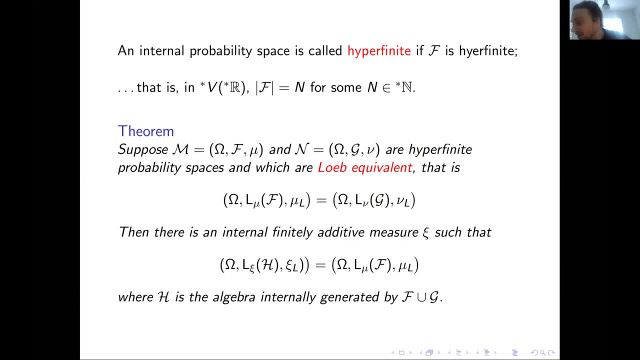 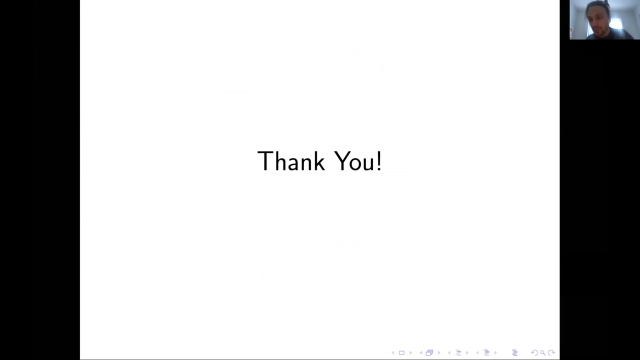 but I think maybe that's not a very good idea because I'm way over time. So for some reason I thought I could show you some of the proof, but actually I don't think I will. So I just showed you the theorem and I hope you find it interesting. 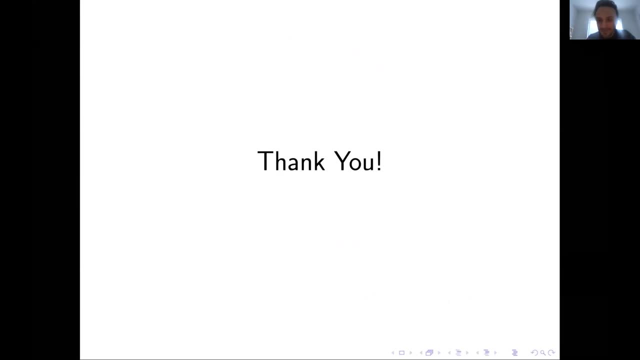 And I say thank you, That's it. Yes, any questions? Okay, I do have a question. So, if I understand right, what the theorem is proving is that whenever, even if you have like an external lobe space and whatever, 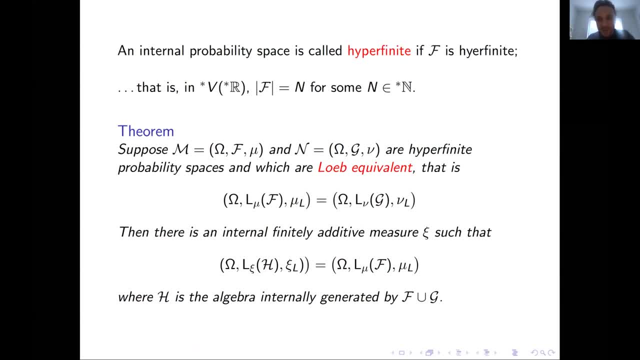 you can bring it back to be an internal one, right? Yeah, I mean, that's not our theorem, That's something that Loeb showed and many people extended it. his result: Yes, but that's true. Yes, you can start with an internal measure. 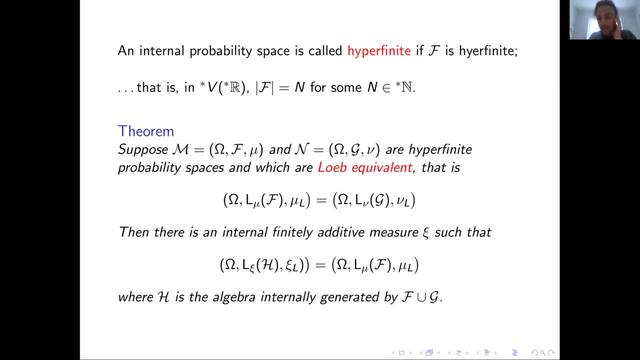 So you do this Loeb construction and sometimes you also perhaps move to a space that's very similar to the Loeb space using the non standard map, and you get very useful measure, something like Lebesgue measure or a stochastic process.